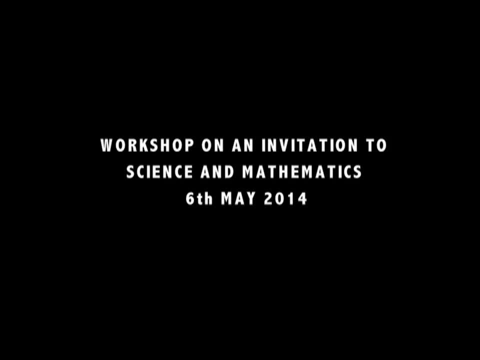 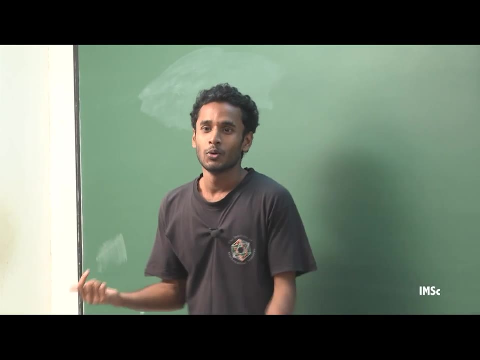 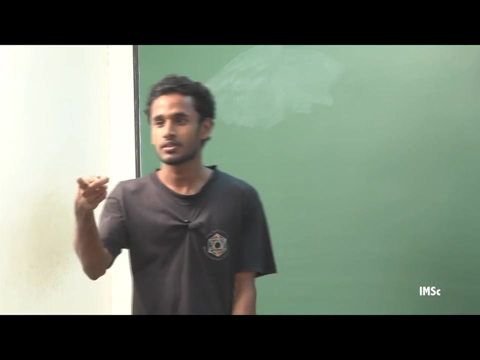 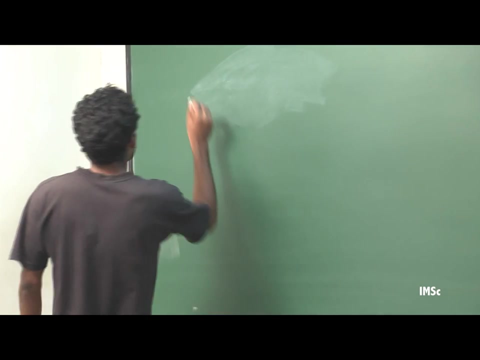 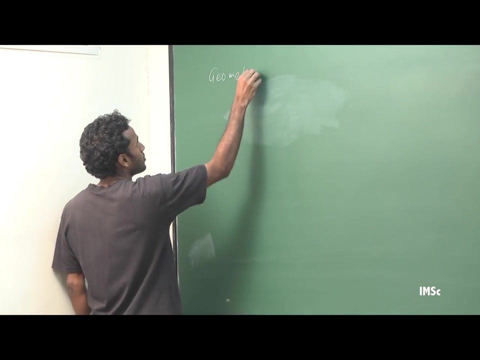 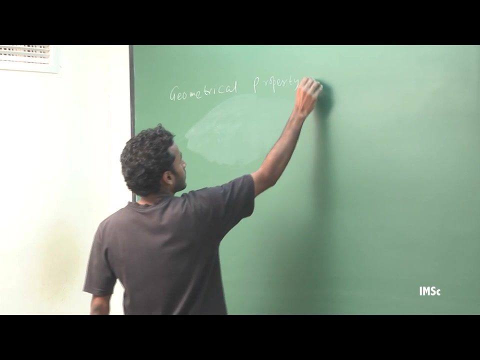 I am going to demonstrate you some geometrical property with the help of with folding some papers. folding or cutting some papers So that papers are with you and everyone has got two sheets of paper right. So folding some papers right? So I am going to demonstrate. 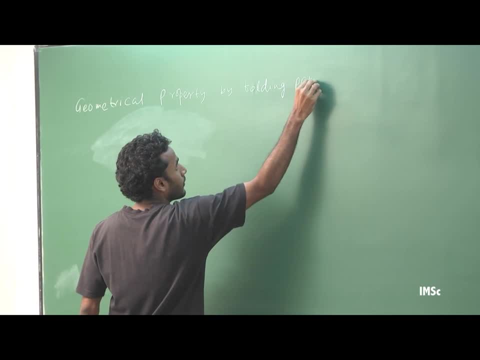 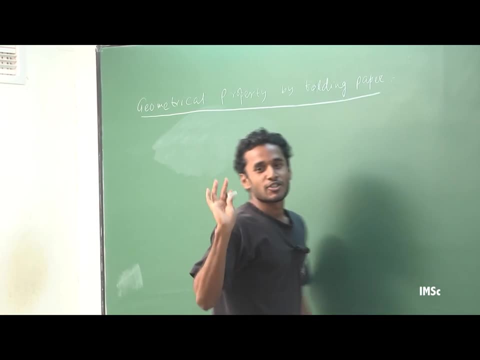 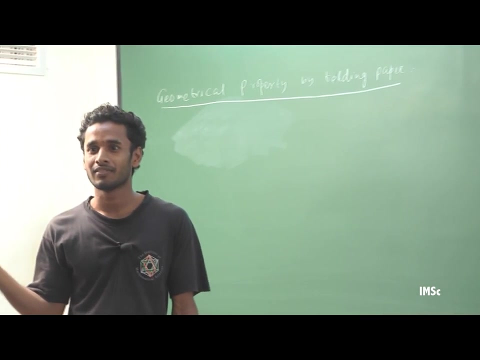 you some geometrical property with the help of with folding some papers, right? So that paper is a little big piece, right? So I assume that everyone is familiar with some basic things. Everyone knows about what are parallel lines. everyone knows, right, everyone. 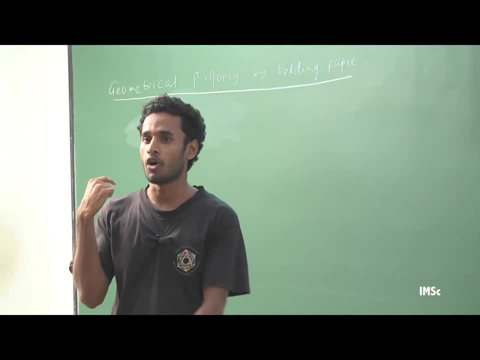 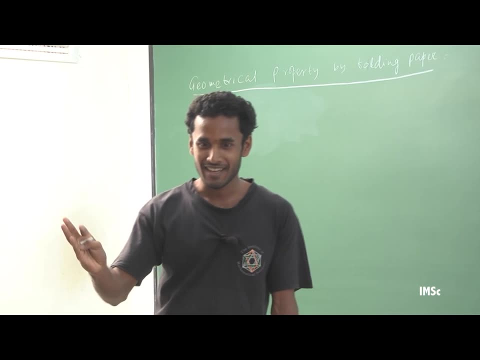 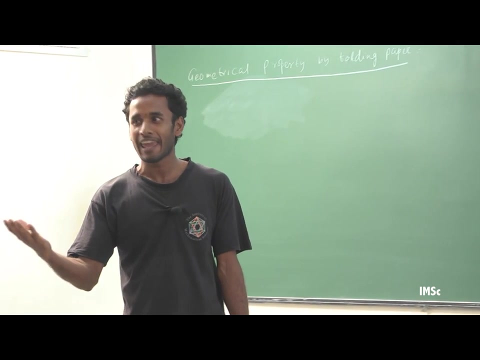 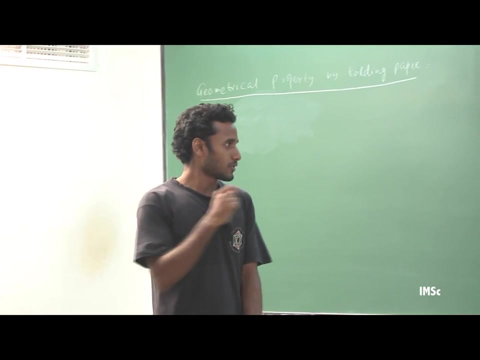 And what are? the theorem for congruency of a triangle? Everyone knows this: S, A, S, A, A, S, S, S, S, R, H S. and is there any? A, A, A, No, Good, That is similarity. Yes, that is similarity. Good, I know. I want that you should know some properties of similar. 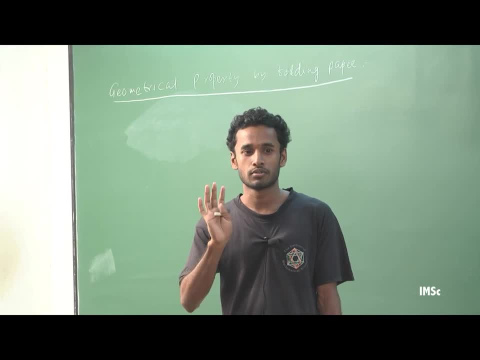 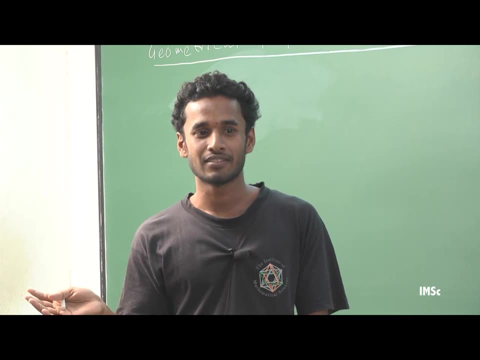 triangle also, Do you know about what are similar triangles are? Yes, sir, What are similar triangles? They are similar to each other. That is, ratio of the sides are same. Ratio of the sides are same. Proportional- Good Proportional. 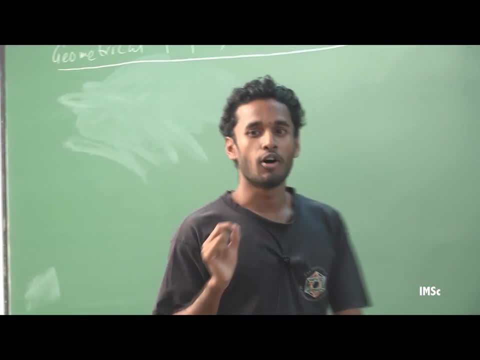 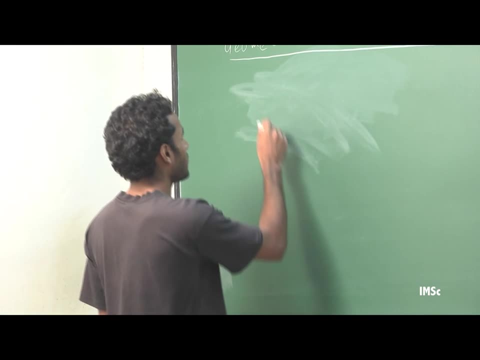 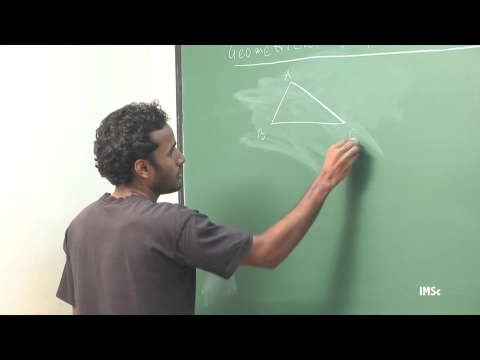 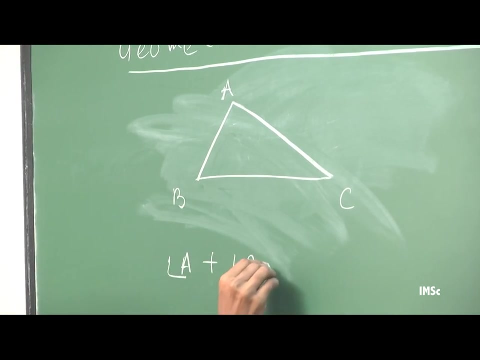 So everyone knows what is the sum of the all angles of a triangle: 180.. 180. Right. So if I have a triangle A, B, C, Let me call this angle as A and let me call this angle as B. and this angle. 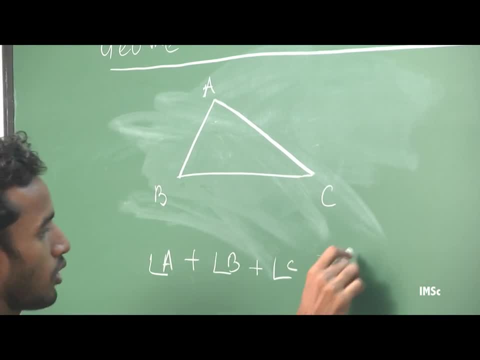 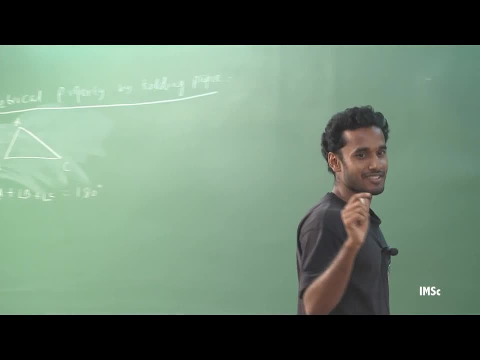 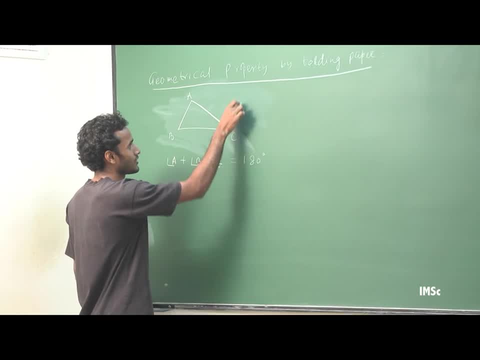 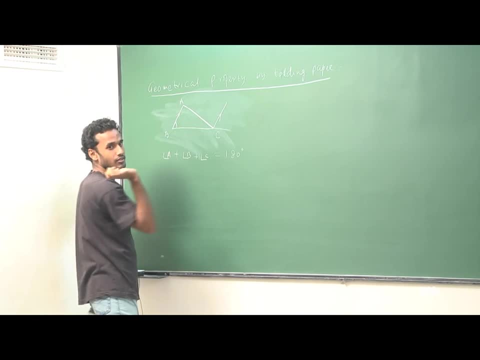 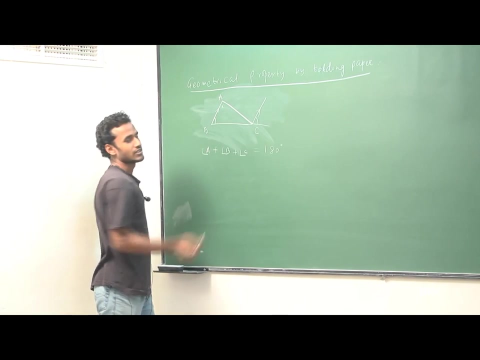 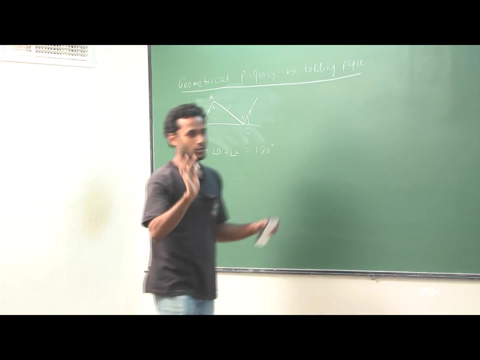 a line, Draw a parallel line to this Right. This is parallel to this And this angle is equals to which angle? This one Right, And this angle is equals to The upper angle, The upper angle, Good, And this is common. So this is 180.. Right Now. 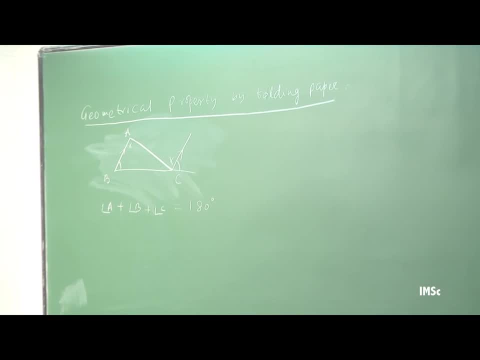 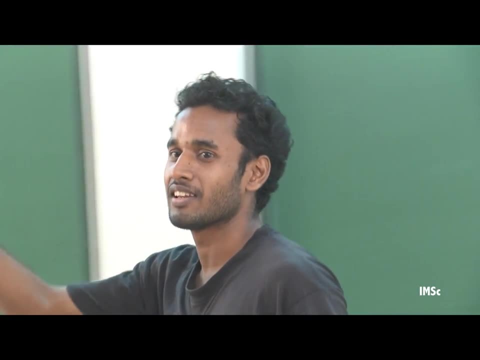 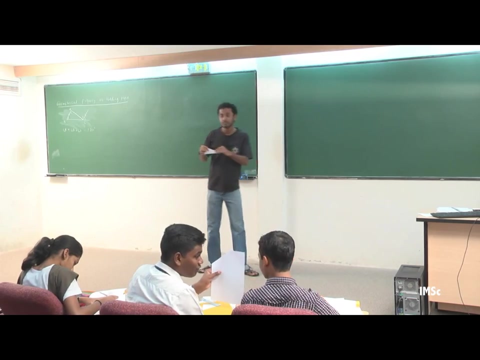 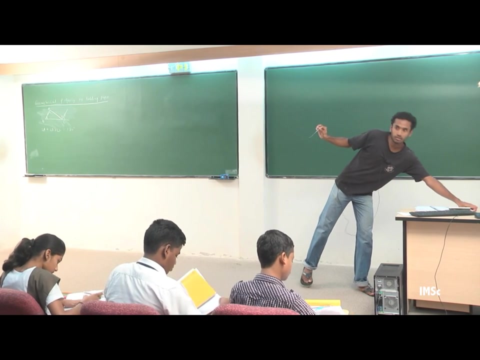 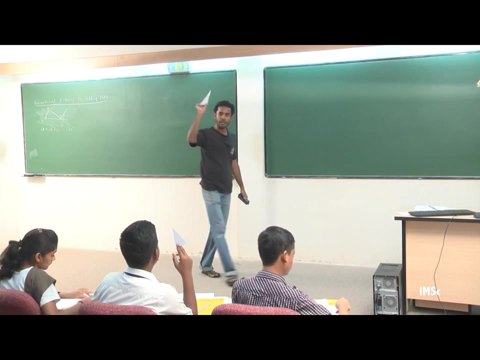 from any sheet, From any sheet of this paper, just cut a triangle of any size, Any size of triangle, Just cut it. Everyone has cut this triangle, Yes, Sorry, Yes, So you have two sheets of paper, Right So, from any one of the sheets, just cut a triangle of any size, Right So? 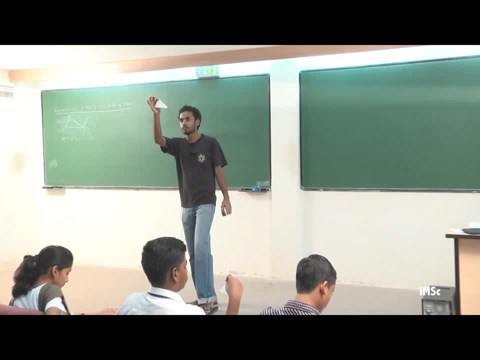 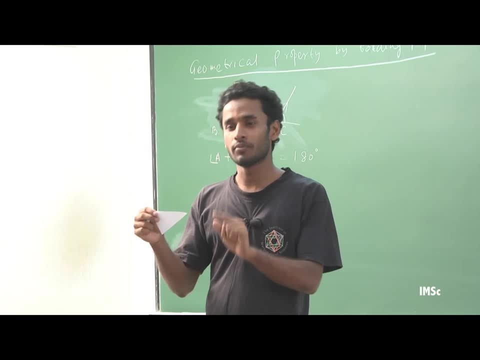 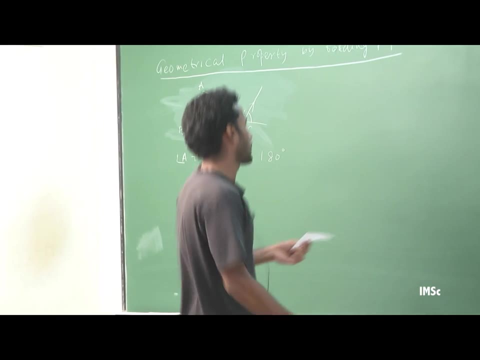 just cut a piece of triangle. Everyone has done this Right. So now leave the biggest side of this triangle. Concentrate on the other two sides Means this is the biggest side of this triangle. So what I have drawn, like this, Like this- Don't look at this. 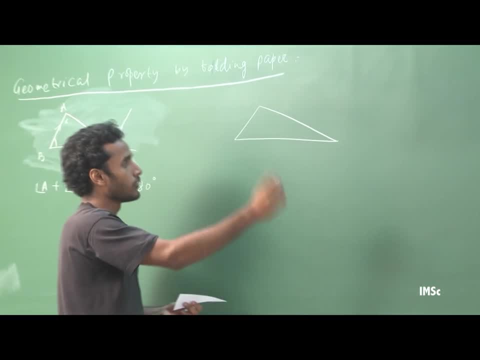 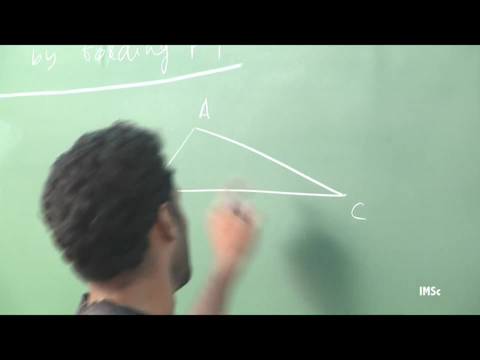 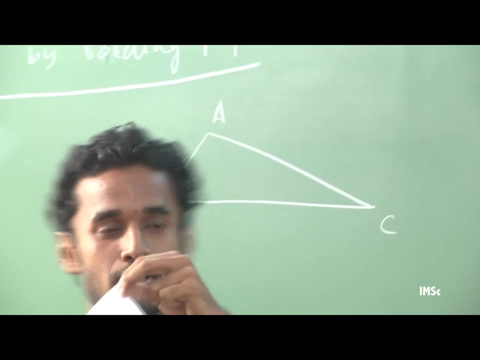 This one is the biggest side of this triangle. So look at these two sides. Let me call A. Let me call A, B, C. Now locate the middle point of A- B. So how to do that? Just fold. 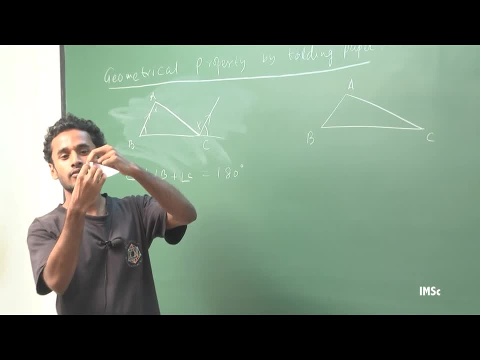 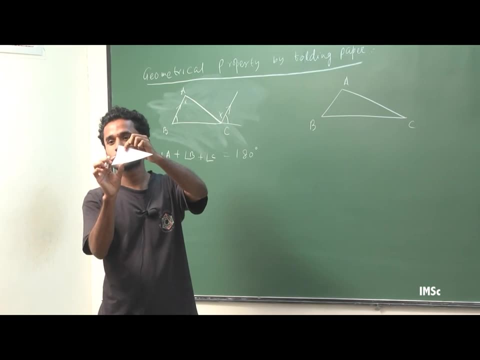 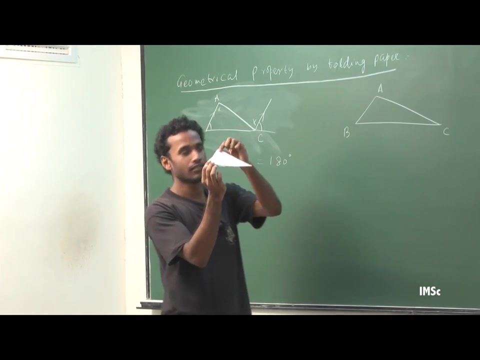 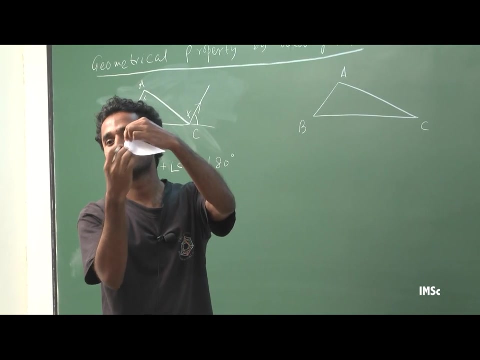 it. fold these two vertex like this and make a- just a scratch. So this should be the middle point of A- B. Everyone has done this. Yes, Take this vertex A and this vertex B and just fold it with together and just make a scratch. 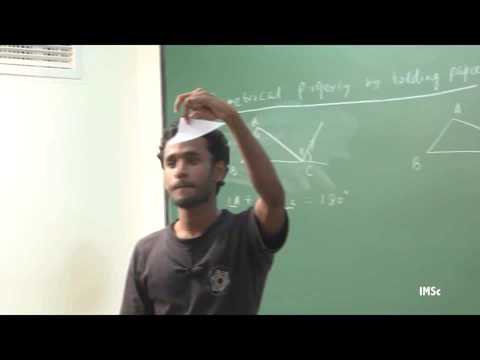 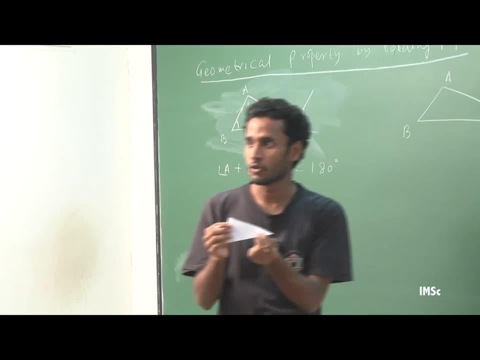 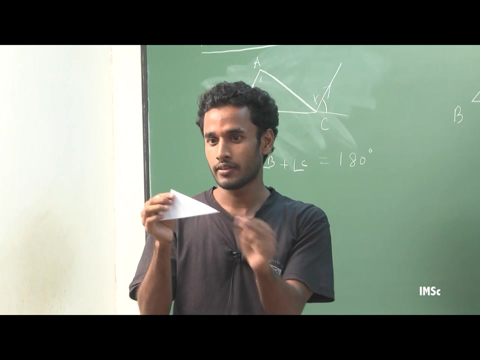 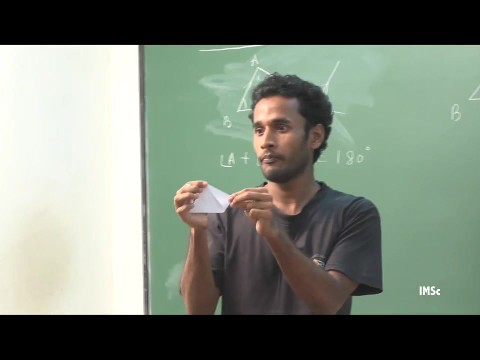 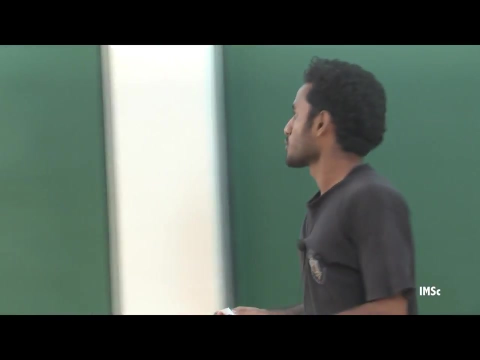 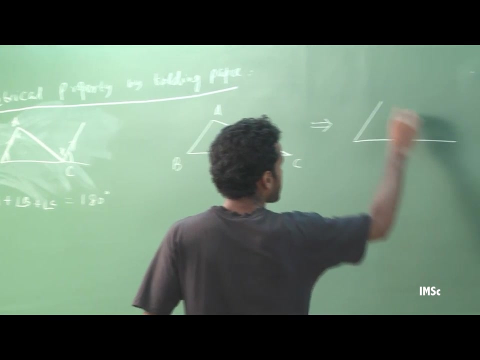 Everyone has done up to this. Yes, Everyone, Yes, Okay, Similarly, do it for the other side, Other side, also This side. How to do that? Just again, make a scratch on this. Everyone has done this. Yes, So what I have done up to this? I have just face the middle point. of A, B and A C. Yes, So what I have done up to this? I have just face the middle point of A, B and A C. So what I have done up to this, I have just face the middle point. 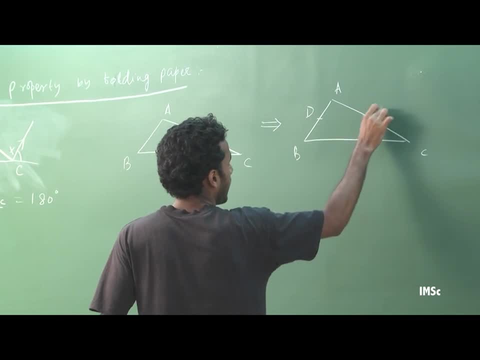 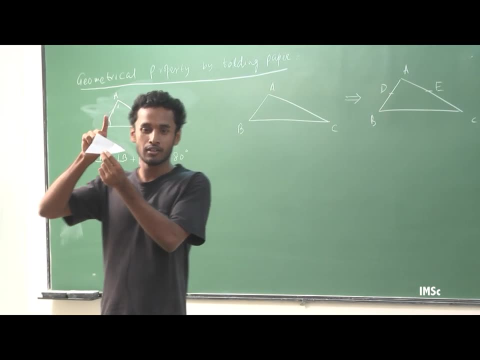 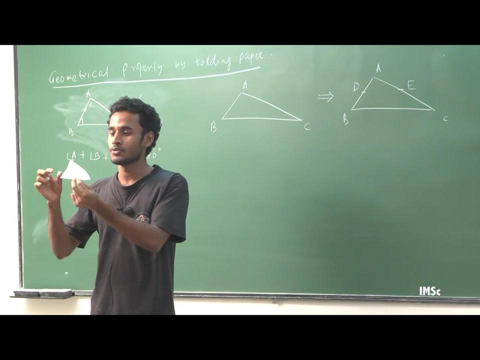 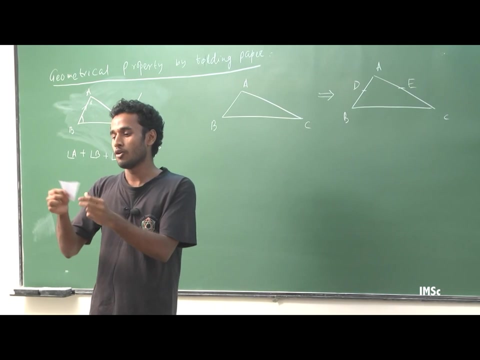 of A, B and A, C, Let me call it B and E respectively. Now fold this upper half of this triangle, this vertex A with respect to the line joining D and E. So you have made two points. you have made two points and now fold the upper half with respect to. 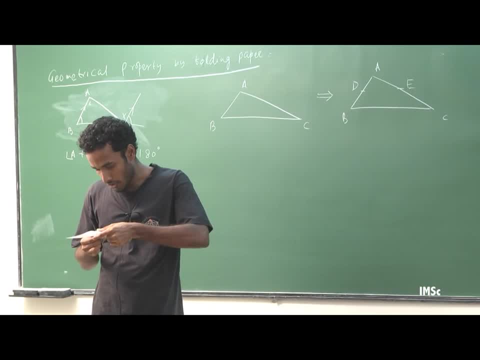 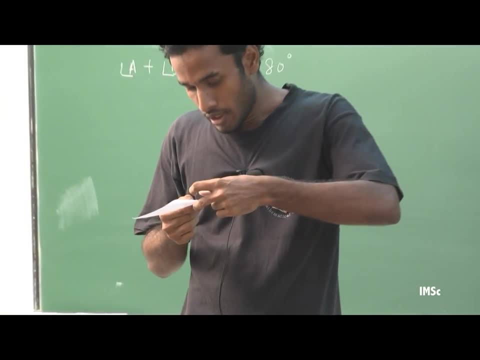 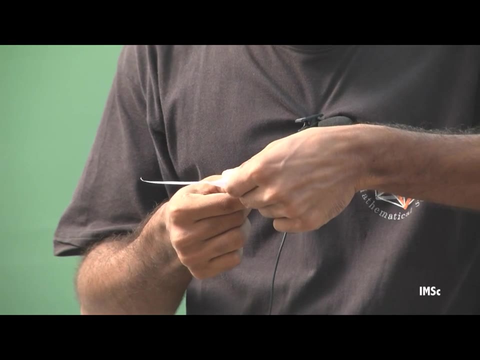 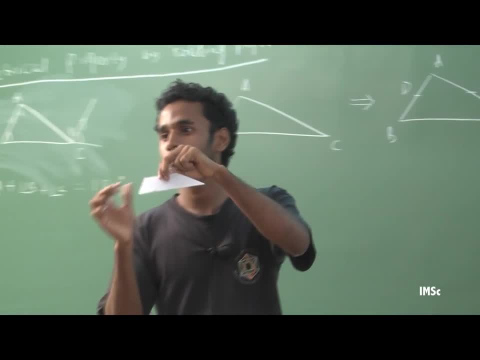 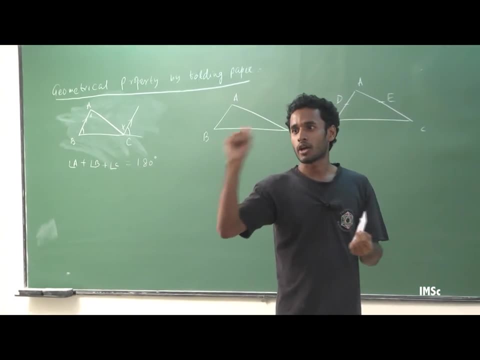 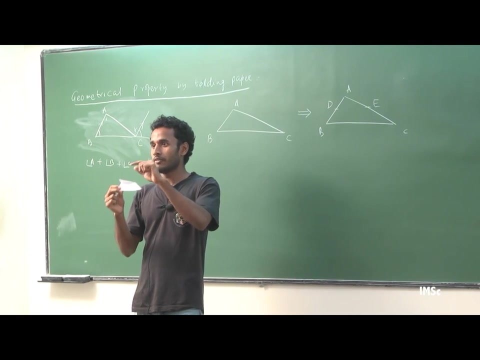 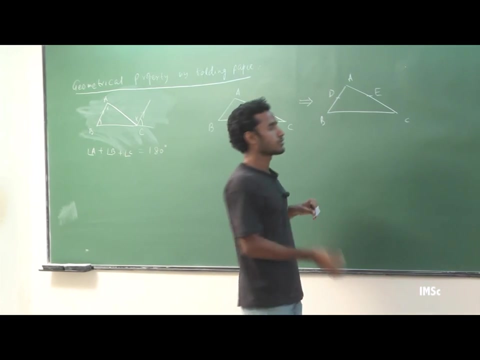 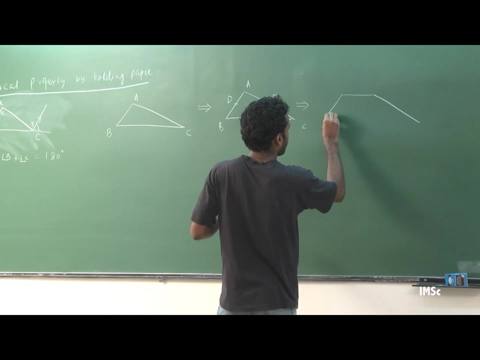 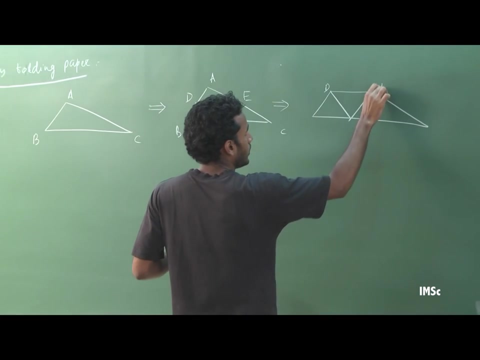 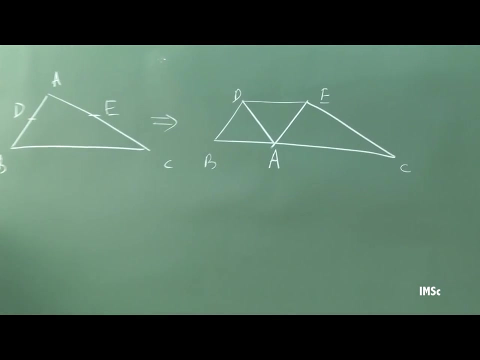 Everyone has done up to this. Hold the upper half of the triangle, vertex A, with respect to this line D E. If you do it carefully, the vertex A will touch the base B C, Right, Yes, Yes, Yes, Yes. Let us add the point point A, B, C. 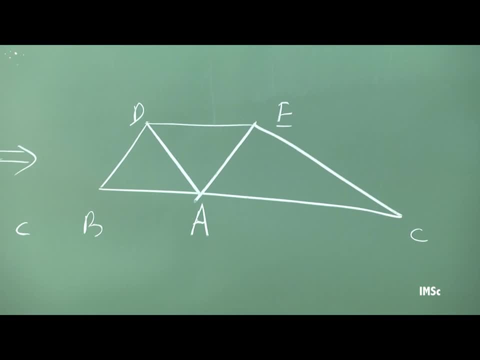 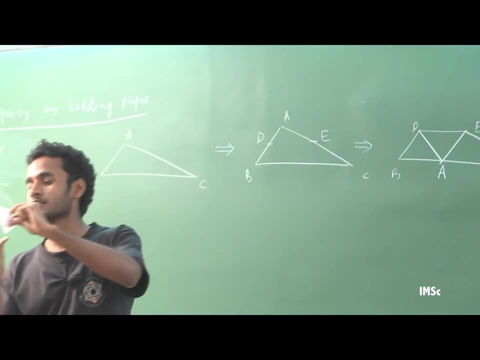 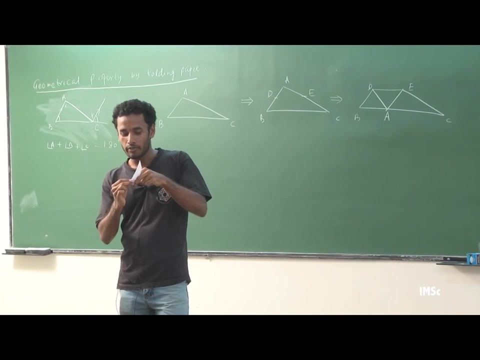 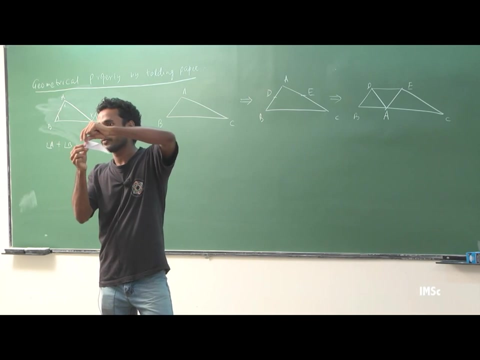 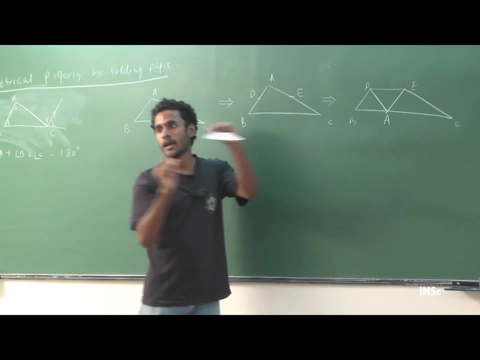 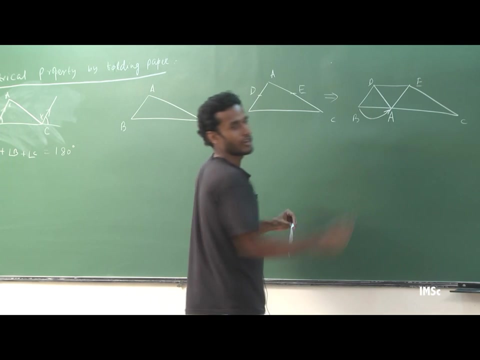 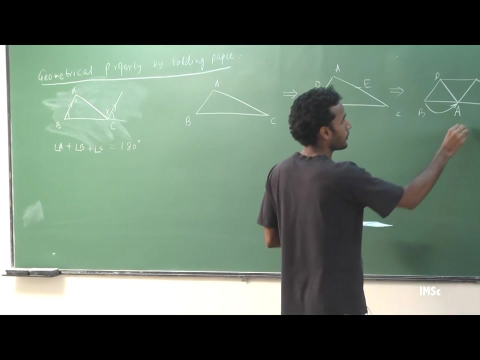 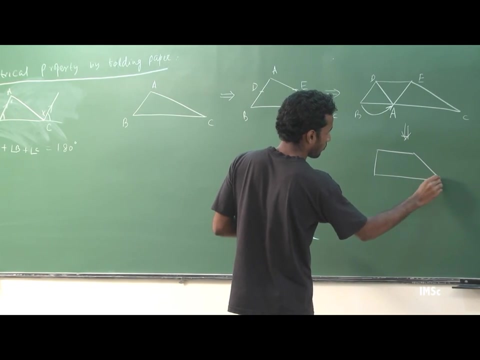 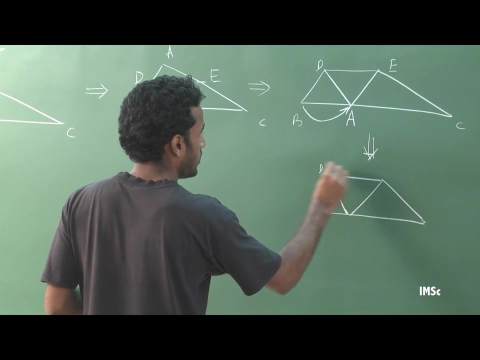 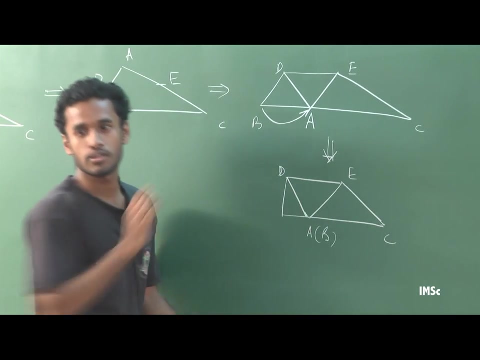 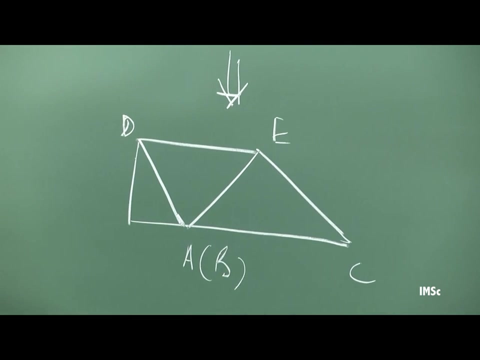 This is D, E, this is B, C and now A the point has. So what I have done now look like: this is D, E, A and B point come together, C. Now do it. do the same thing for the vertex C also. Just take the vertex C, just fold it you. 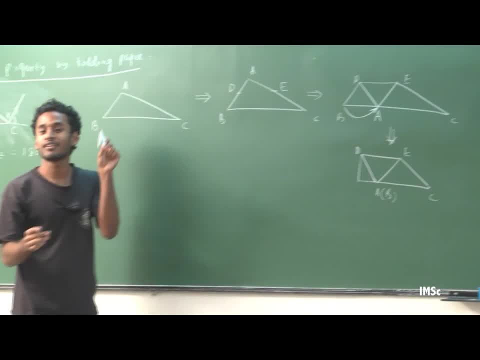 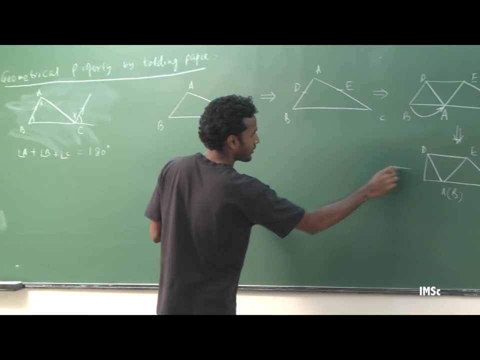 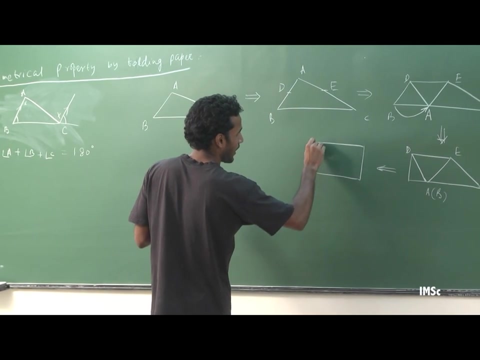 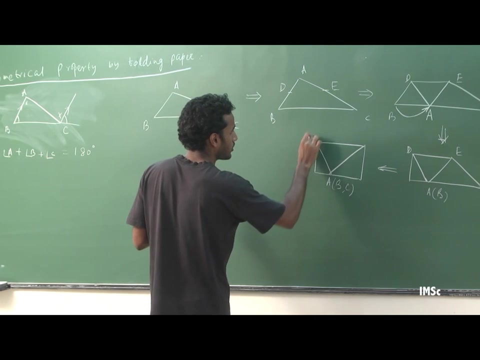 will get rectangle right. and what you have got, You have got another thing also. So what we have got here, Yes, a straight line, and like this: A, B and C all come together, this is D, E, They come. 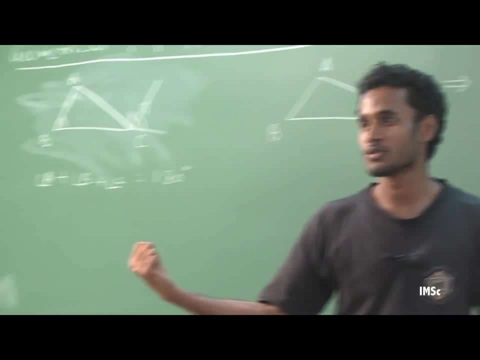 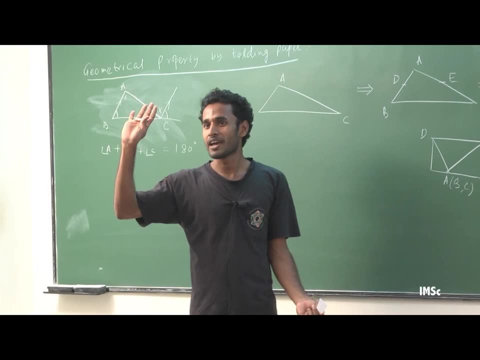 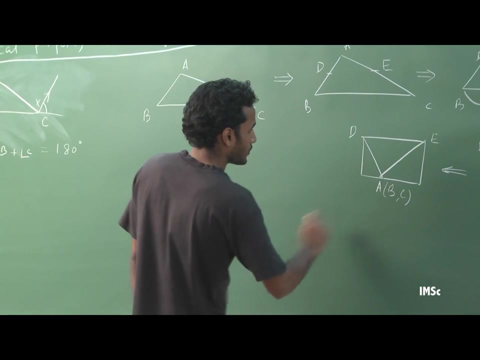 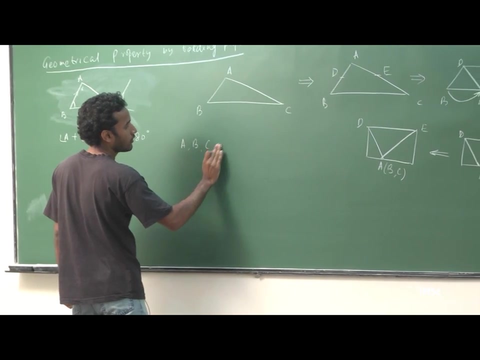 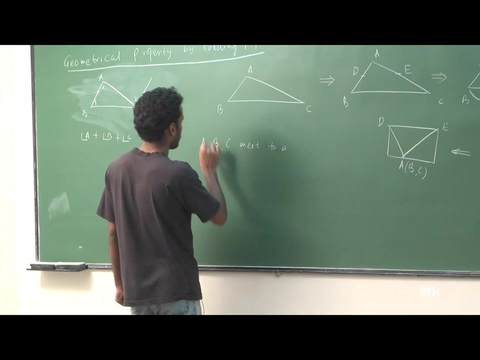 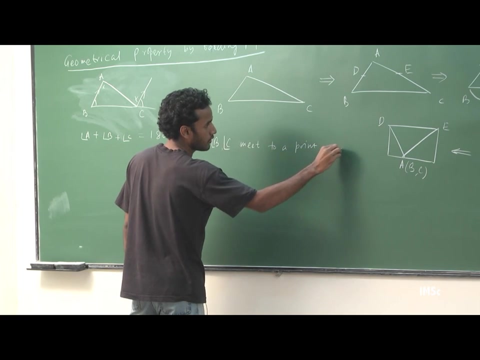 to coincide to a one point and coincide with one line also right? Everyone is happy with this. Yes, Yes, Okay, thank you. So point A, B and C angle, A B, C mean with point and coincide. So point A, B and. 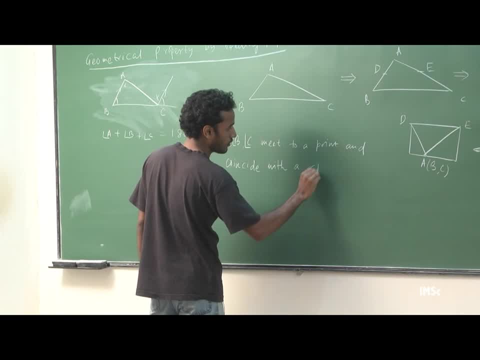 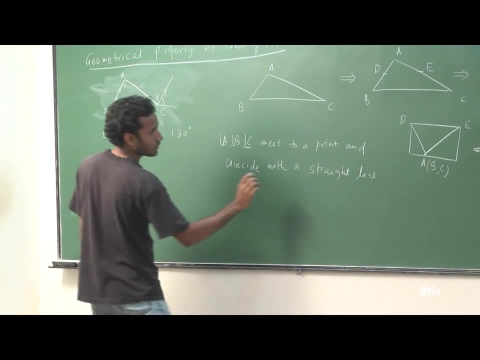 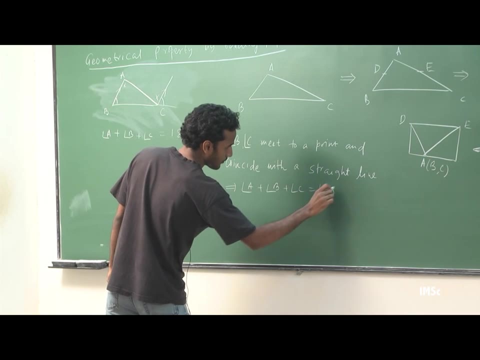 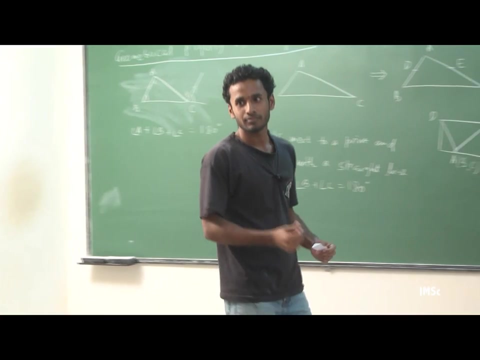 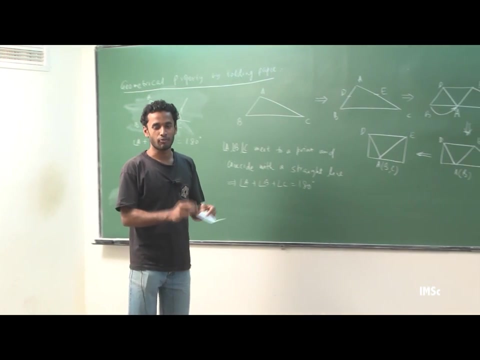 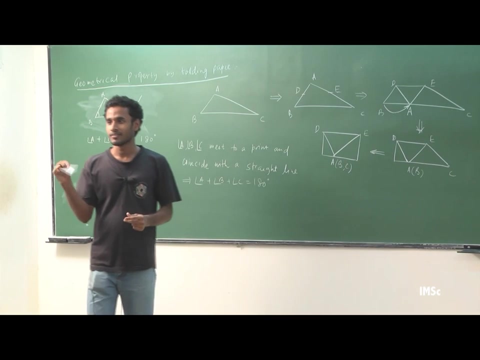 with a straight line. This means angle A plus angle B plus angle C is 180, right? How does this work? Anyone can tell me. I have told you to just make some folds and certainly these three angles come to a point and meet the straight line. Sorry, Sorry, No take. 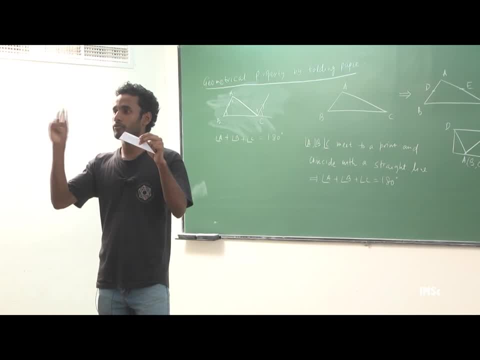 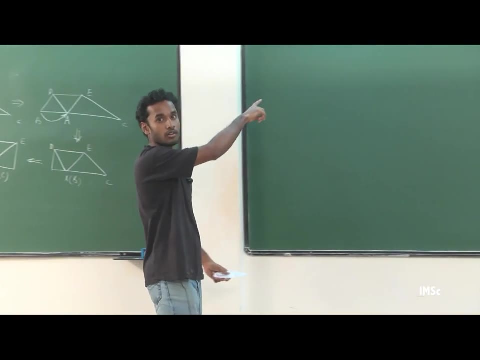 any triangle. It is not true for right angle triangle. So some of all the angles of a triangle is 180.. It is true for any triangle. I have not taken any right angle triangle here. Okay, just let me tell you. So how does this come? Can I use this board? 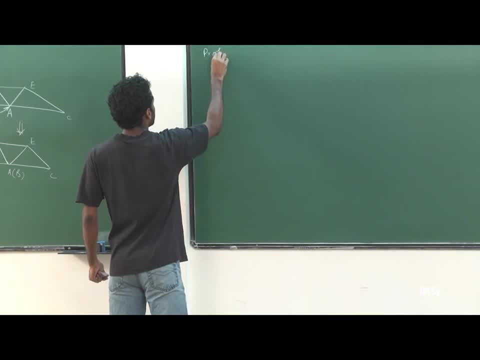 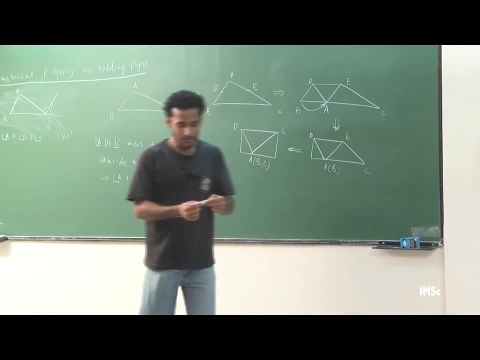 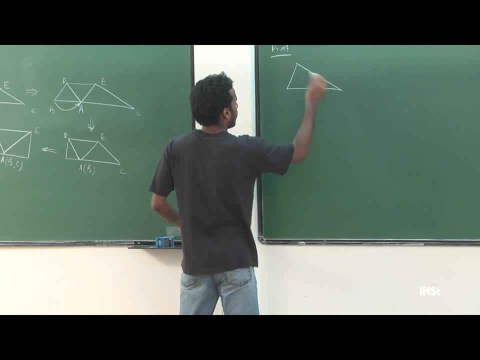 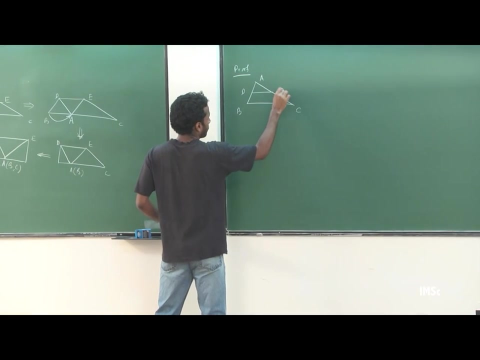 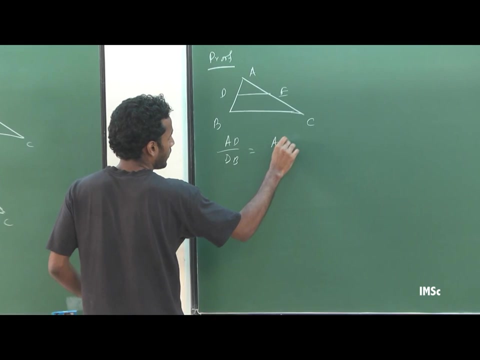 Okay, Okay, Midpoint theorem: Yes, midpoint theorem. I have used midpoint theorem here, So what I have done- I think all of you know this here- right? Midpoint theorem: A, B, C. Yes, In my construction here, my A, D divided by D, B equals A, E divided by E, C equals to, in my 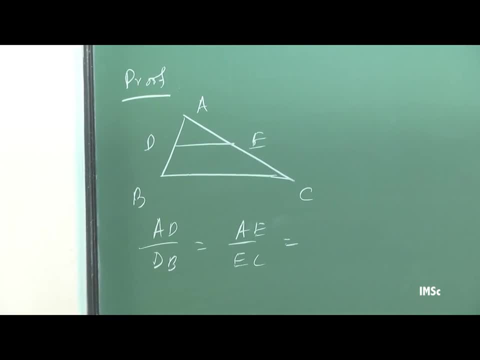 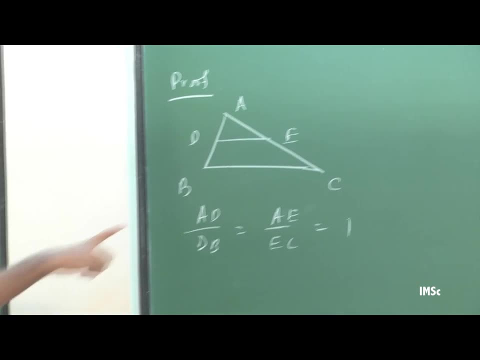 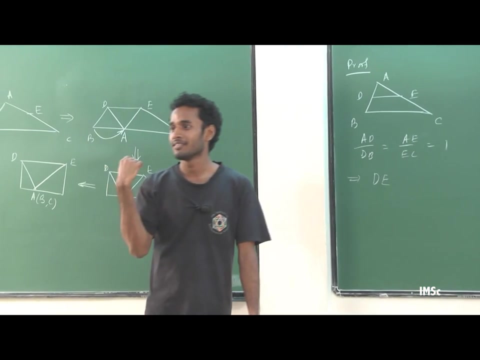 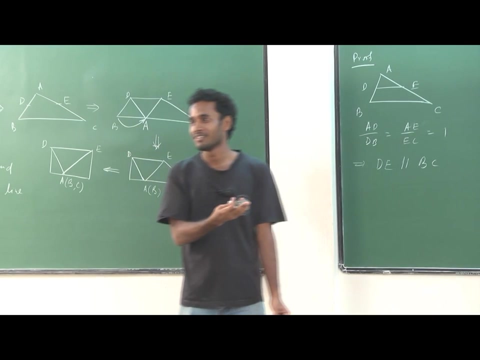 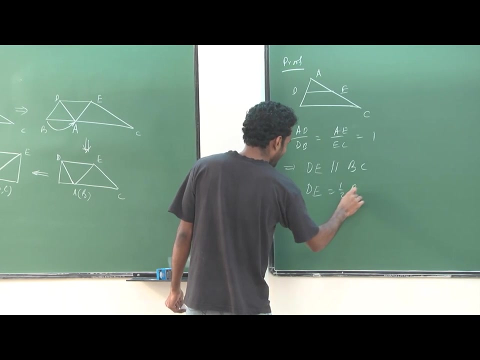 construction: A, D divided by D, B equals is 1. 1: 1 Good, because this is the midpoint Right. So for that reason D? E should be 1: 1 Parallel to which line B C. Very good, D E should be parallel to B C. and there is one more thing: D is half of B C. 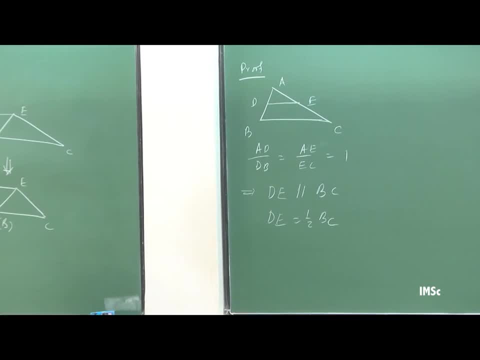 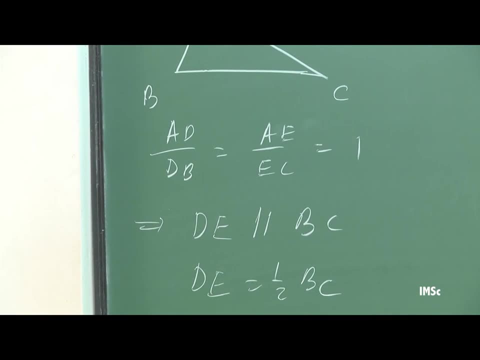 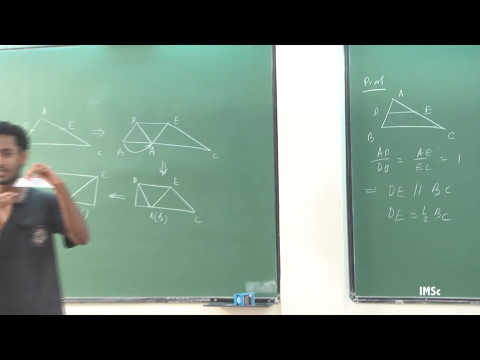 Very good. D is half of B C. So when I have fold this vertex A with respect to this line D E, why this vertex A exactly comes to the base B C? Again, one point here: It is an isosceles triangle. 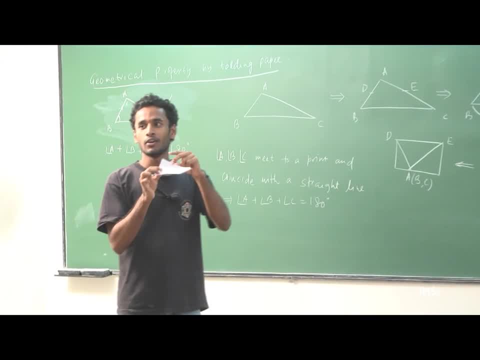 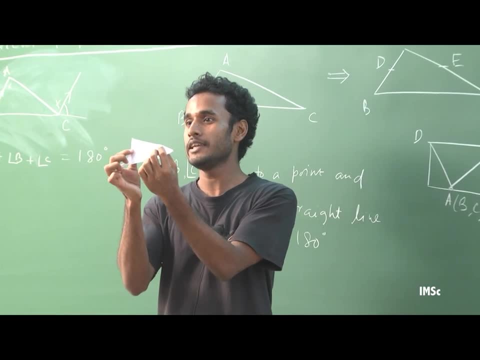 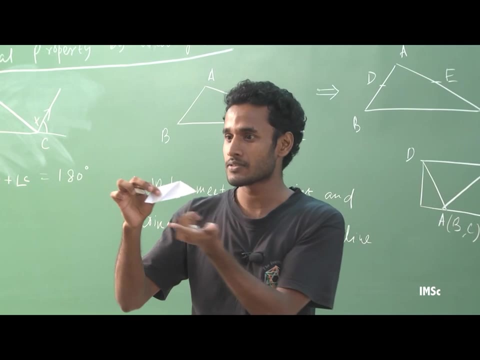 No, it is not isosceles triangle. So what I am asking to you: when I have fold this vertex A with respect to this D, E, you see that this vertex A comes to the base B, C. So why is that true? That is because- again, one point here- it. 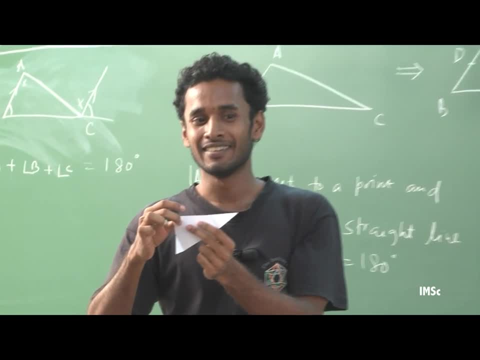 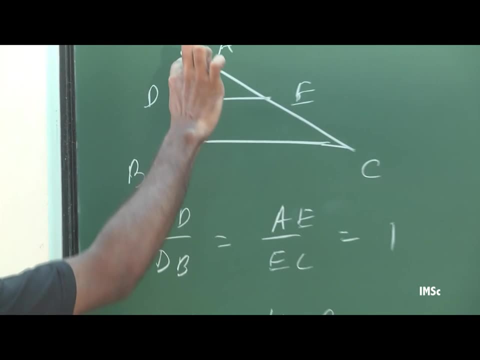 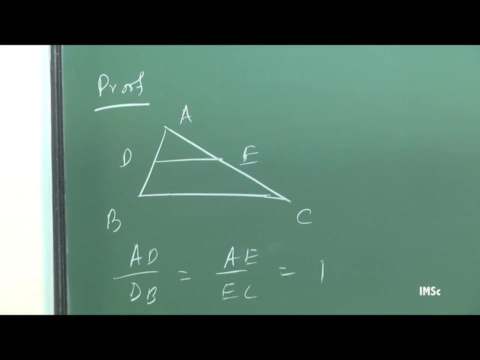 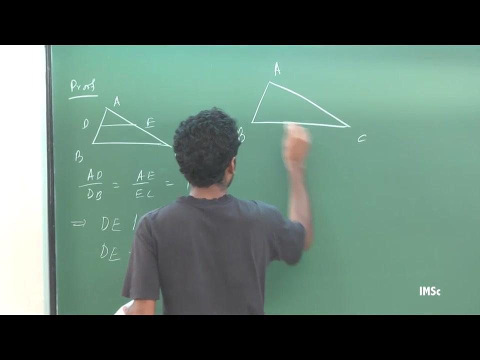 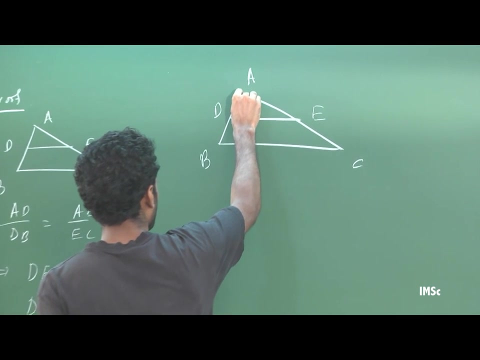 will be equal to half B C, Half B C. this is because this height is equals to this height. So if I now draw A- Yes, A B C, and this is the middle point of D- E Draw a perpendicular from A to B C. let me. 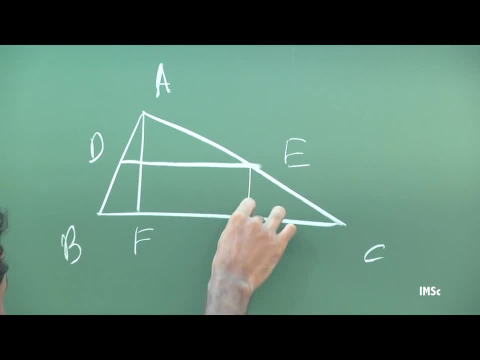 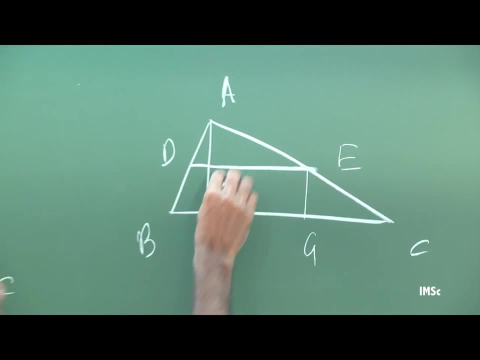 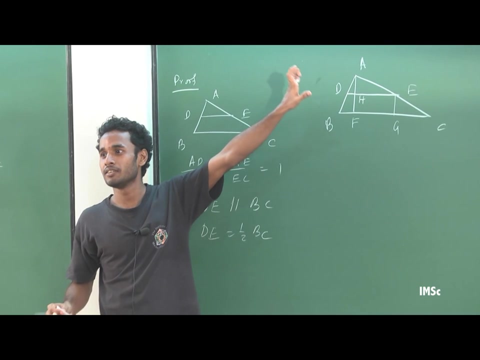 call it F and draw a perpendicular from E to B, C. let me call it G. So can you see this that? let me call it H. Can you see A? H equals to H, F equals to E, G. Yes, sir, How can you see that? 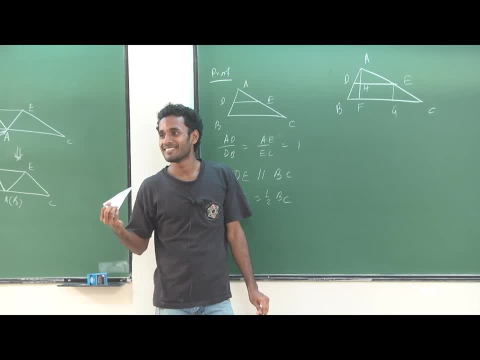 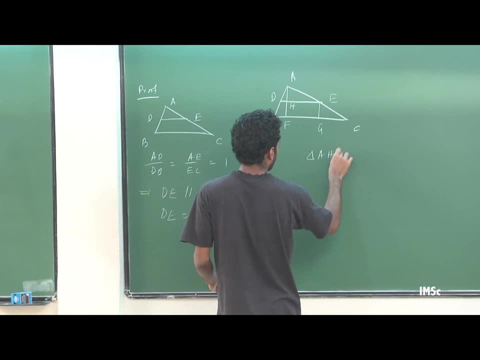 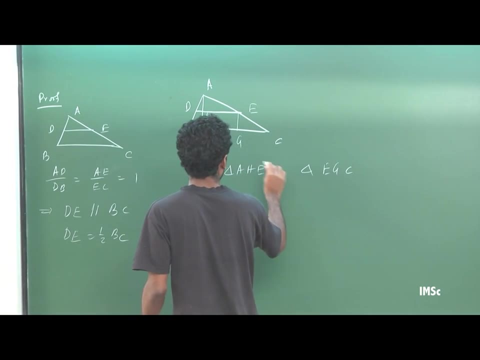 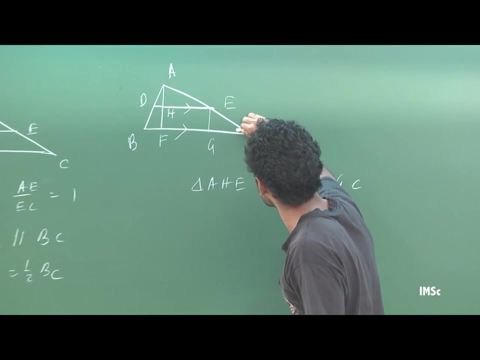 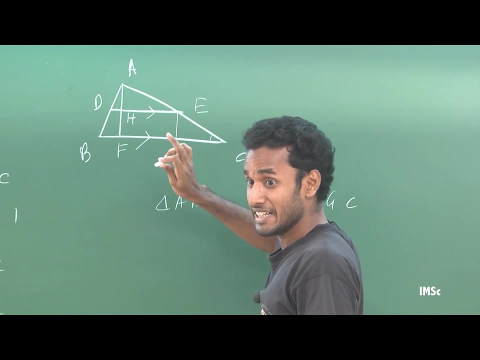 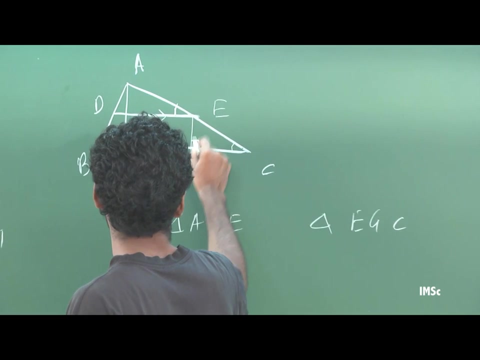 Sorry, Look at this two triangle: A, H, E and E G C. So these two lines are parallel. that means this: Yes, sir, Yes, angle should be equals to which angle AED? Good, this one, and I have drawn a perpendicular. 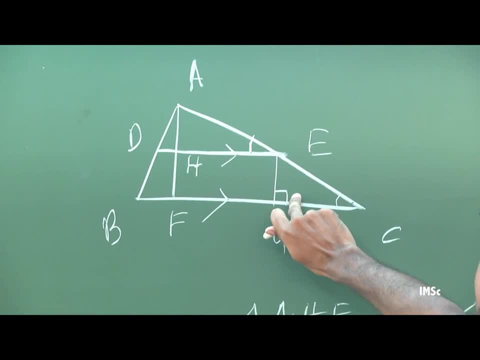 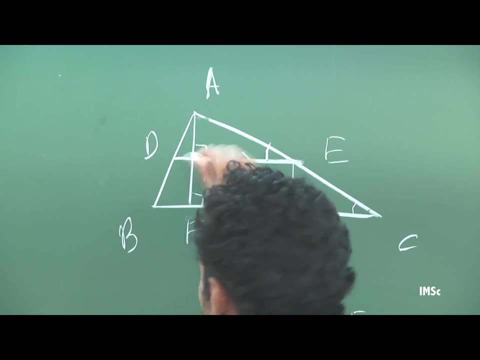 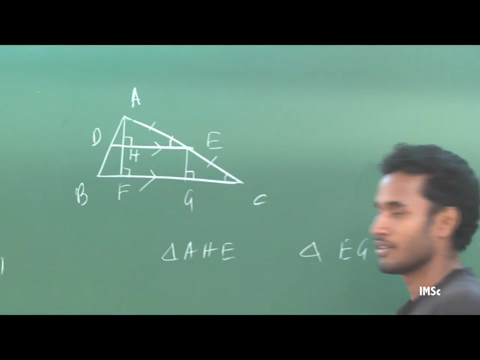 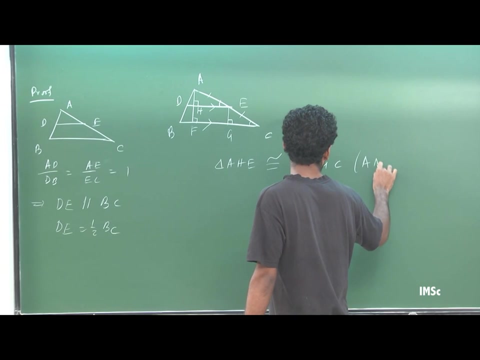 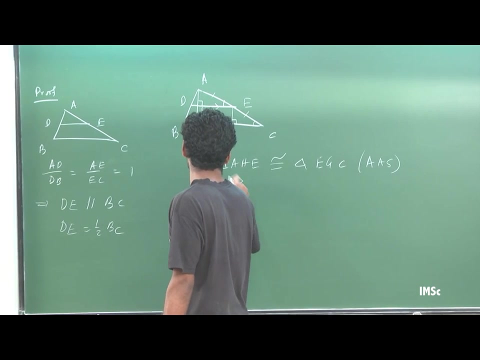 from this point. for that reason this is 90 and I have drawn a perpendicular from this point to this point. So this angle is also 90 right, and this side is equals to this side, right. So it is what Congruent by AAS, right. So for that reason, A H should be equals to. 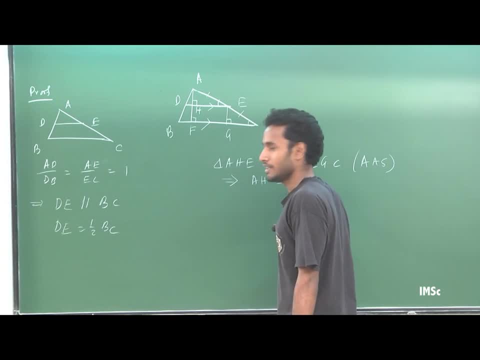 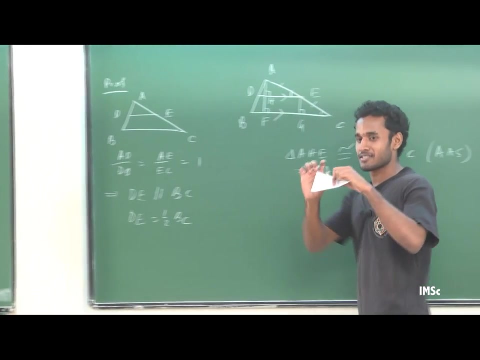 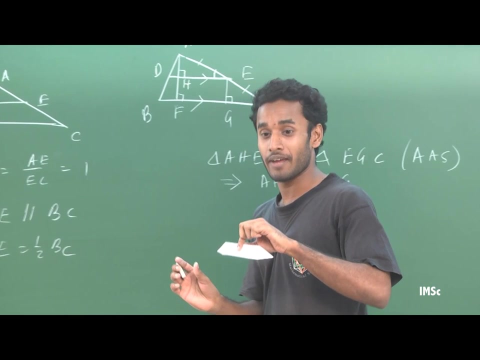 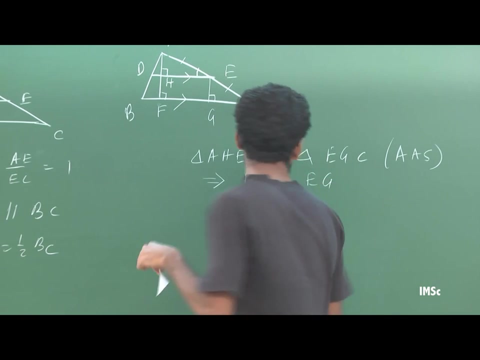 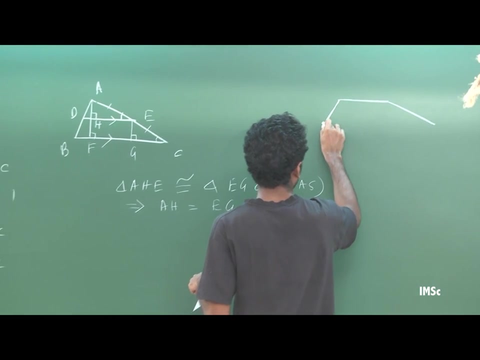 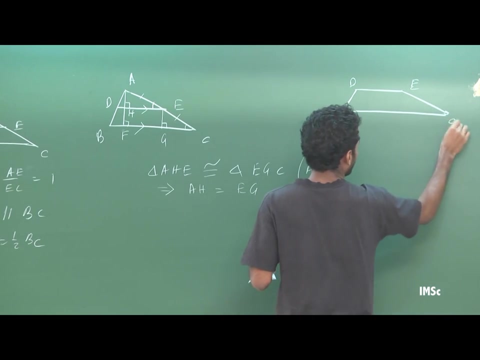 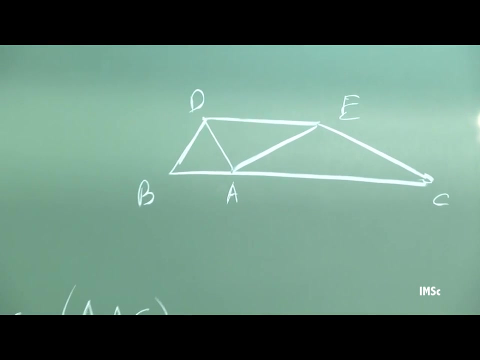 E, EG. Why this is true, Very good. So for that reason, this vertex comes to the base: right. So now, and then what I have done? I have fold this vertex like this: Yes, Right, So what I have done, then: This is DE, this is BC and this is A right. So now. 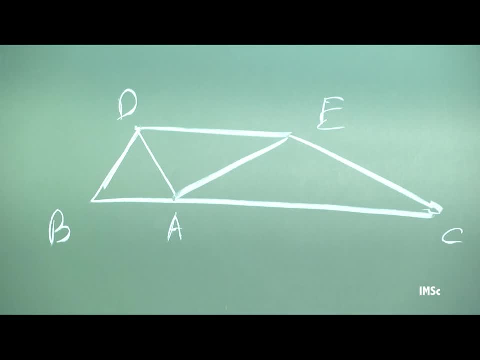 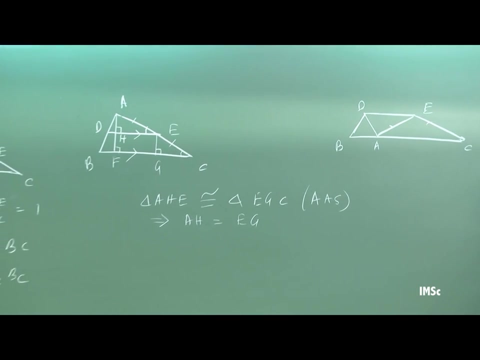 look at this triangle, AEC, This triangle, have one property: AE equals to EC, right for because I have cut that AE Midpoint, Midpoint. So AE equals to EC. that means Yes, and for that reason this angle should be equals to. 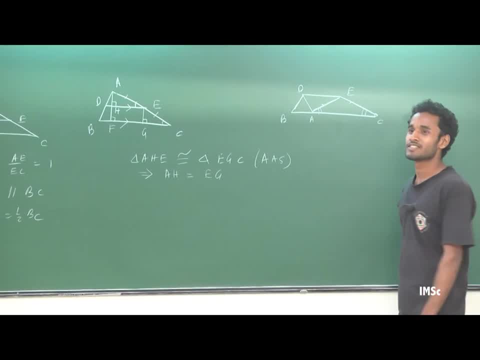 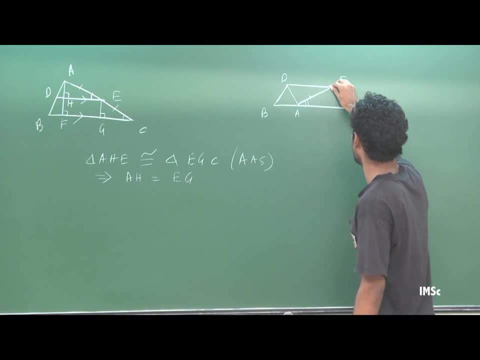 Unstra positive, Unstra, positive, Good, this angle right. So when I have folded like this, that means Yes. So I have folded with respect to a perpendicular. They will be congruent, Right, they will be congruent because this one is: 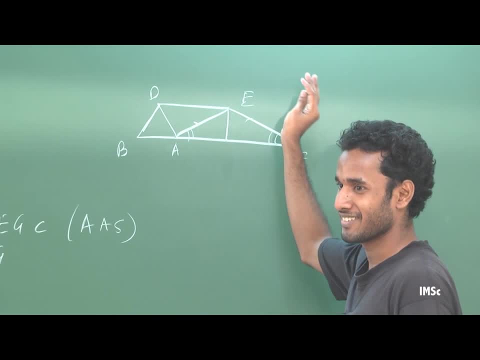 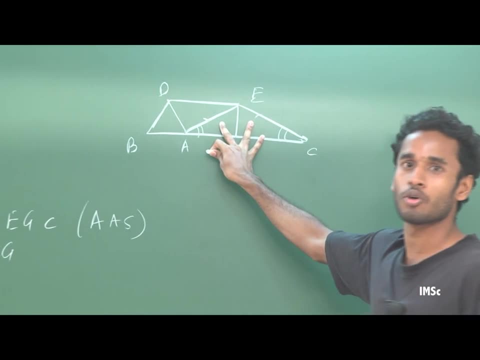 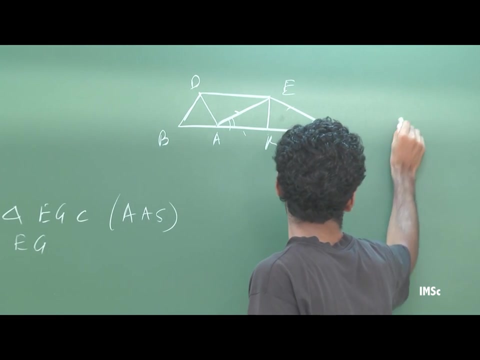 Yes, the common line, Yes, common line. All of all of you agree with this right. Yes, sir, That these two triangles are congruent. Yes, Yes, Right, and for that reason let me just write it: Yes, sir, AKE is congruent to. 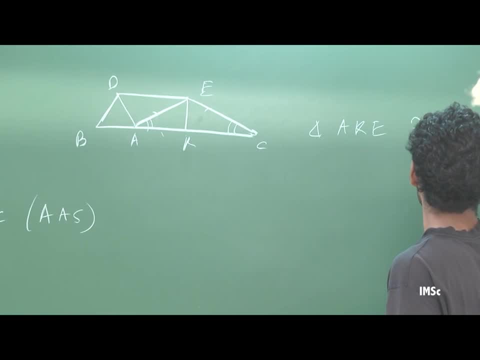 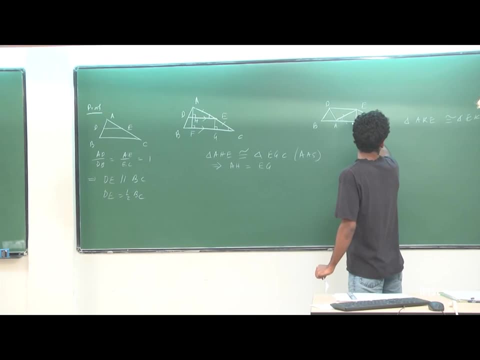 Yes, sir, EKC, EKC, right. How sir, For sorry, CKE, CKE, CKE, this one, EKC, same thing, EKC, same thing, Same thing. How sir, by what congruent CKE is congruent? 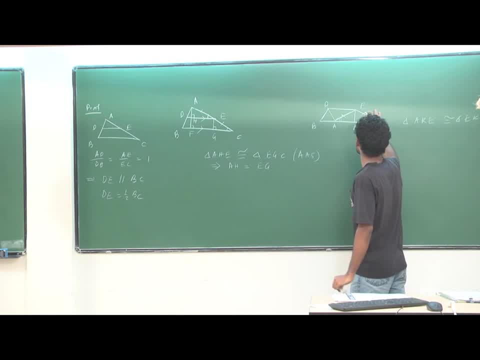 By what congruent CKE? It is the same thing. That is the common. This side is equals to this side. Yes, sir Right. Yes sir, Sir, Ok, It is common, right, This is right angle. First of all, 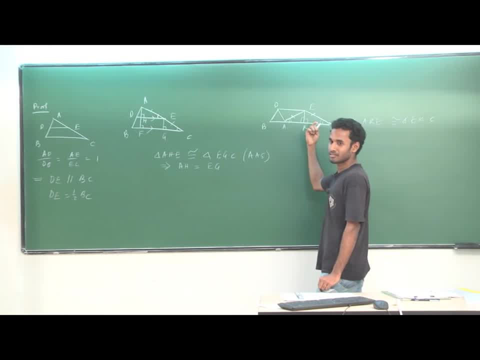 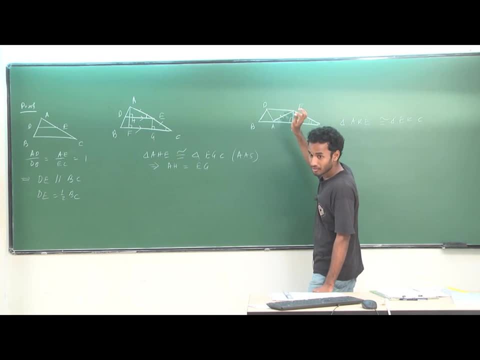 This is right angle, Why AAS That is a common one, EK is a common, EK is common, Sir. then also. then there is no property, Sorry, Like SSA, No No AAS, AAS, AAS. 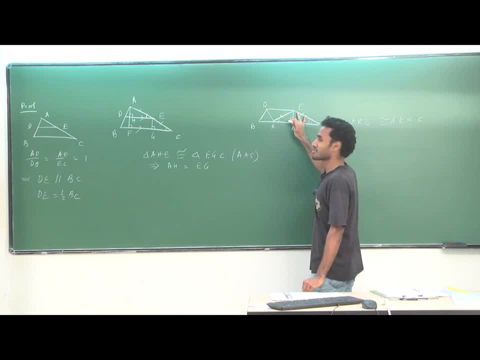 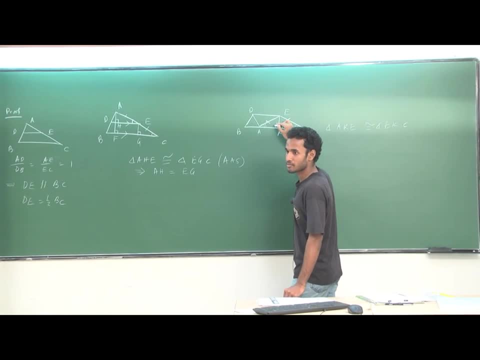 Or RAHS also, RAHS also. yes, This is R, This is AHS Same. Yes, This is common S, So RAHS Right. So for that reason AAS is congruent. Yes sir, Yes sir. 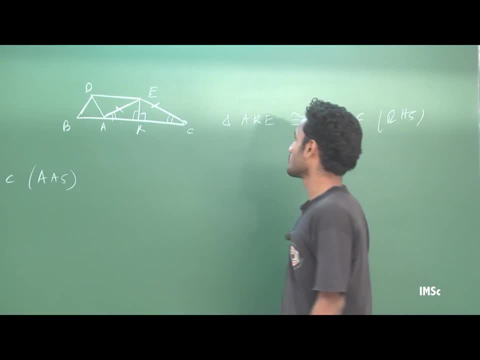 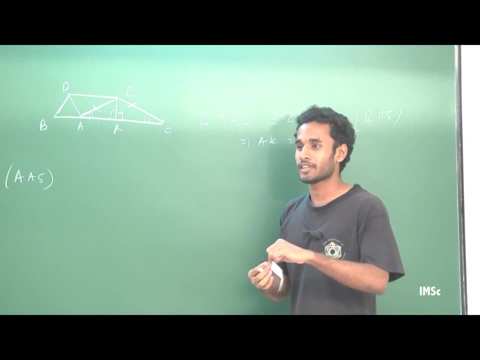 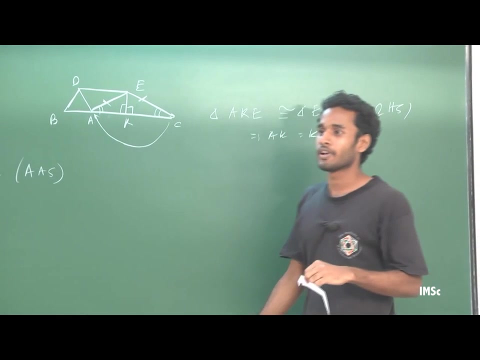 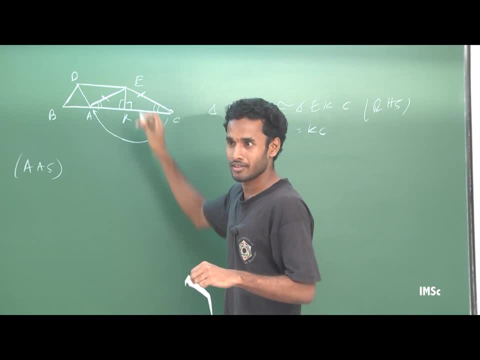 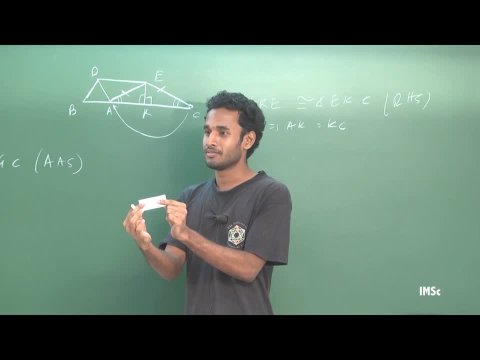 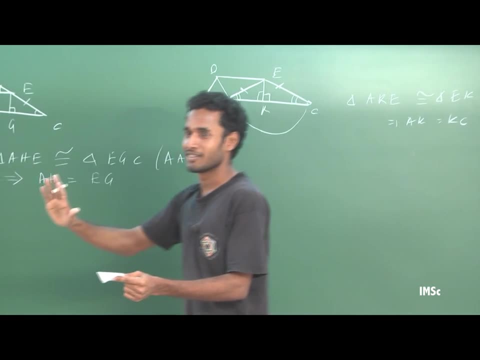 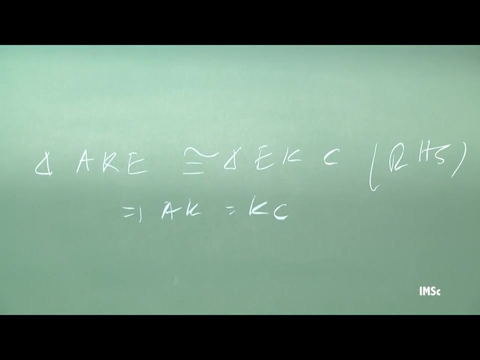 Right, That is true for this half also. Ok, sir, So for this half, the same logic Over there, Over there. So for that reason, So all of you have are satisfied with that, the angle of three triangles is 180.. 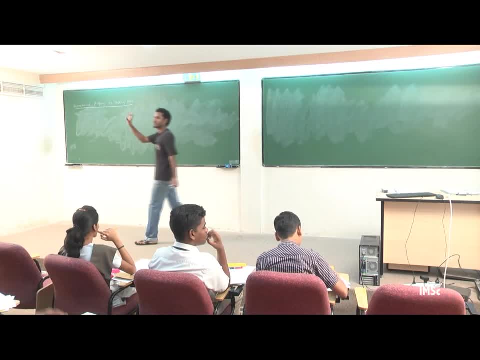 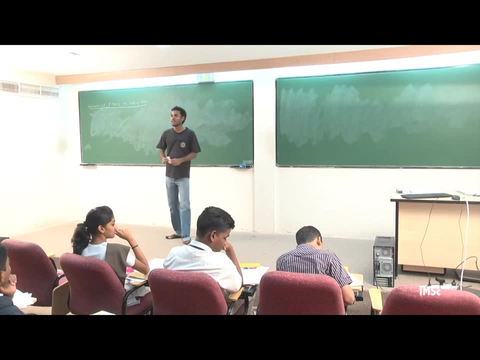 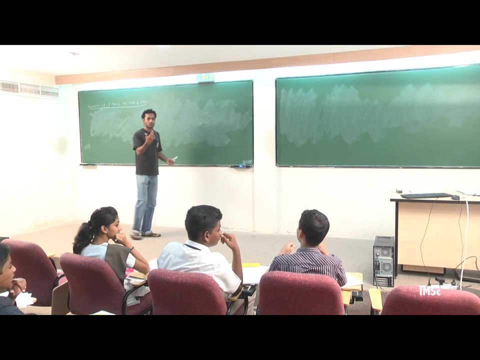 Right, Yes, sir, Yes sir, Ok, By construction. No, sir, Who knows this? Anyone knows how to trisect a line, Sir, Sir. You know, Sir, How to Can you do with only pencil, compass and ruler? 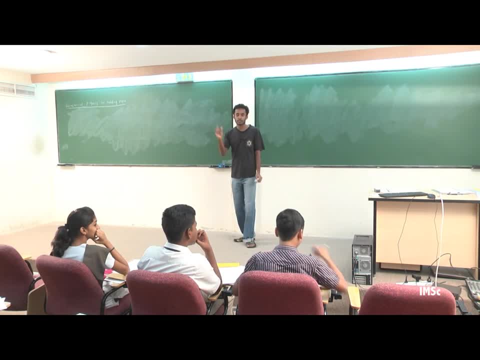 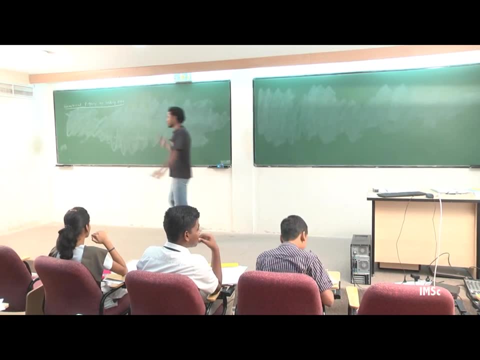 Yes, sir, With pencil, compass and ruler can you trisect? and just a line. Yes, sir, So how to bisect a line If you have? Sorry, If you have a line, So how to bisect it, Sir. 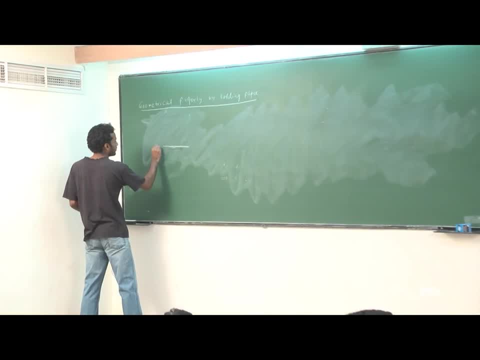 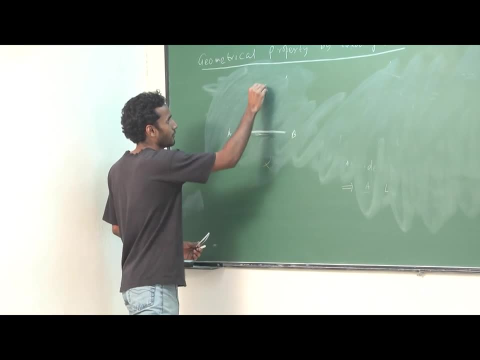 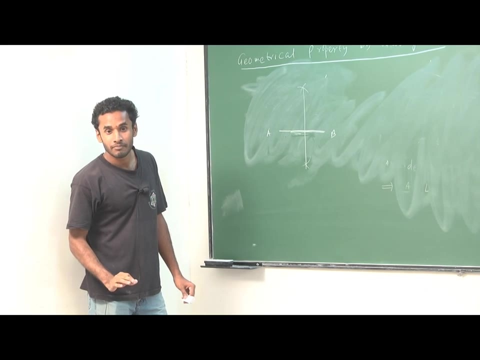 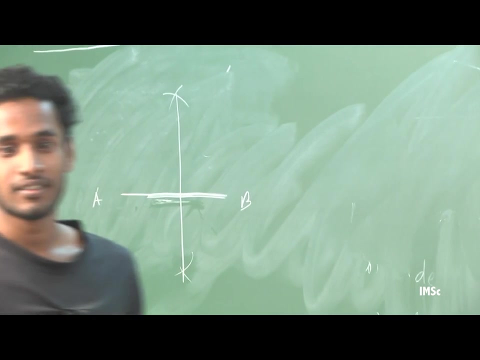 Sir, Sir, Sir, Sir, Is it necessary that the line should be cut equally? Is it necessary when trisecting in line, does the line should be cut equally? Cut equally three parts. No, no, Yeah, Cut equally three parts. 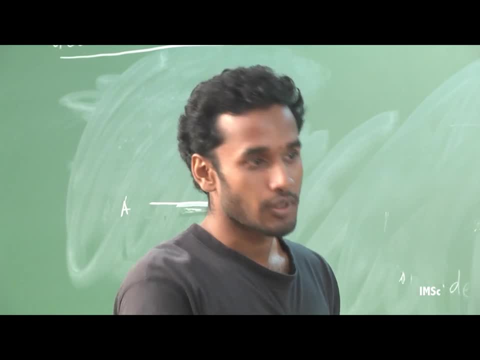 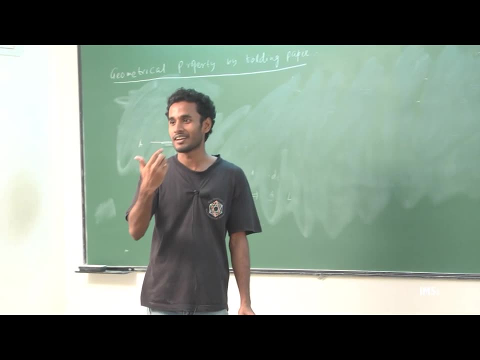 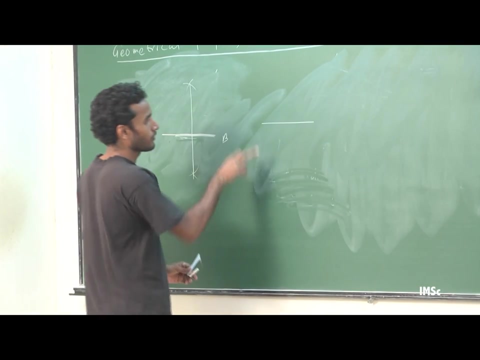 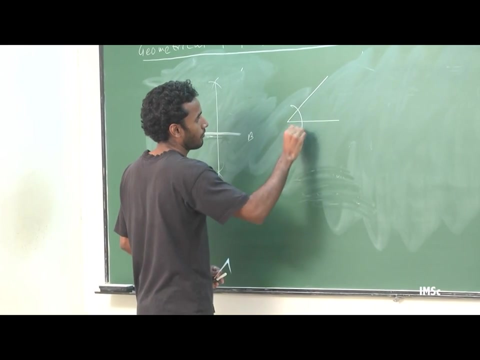 Sir, Will we be supplied with a graph sheet? Will we be supplied with a graph sheet? Ok, You want to do with by a graph sheet. When you asked me- Yes, sir, by your geometry class construction- How to do that. Draw any line and draw any angle. 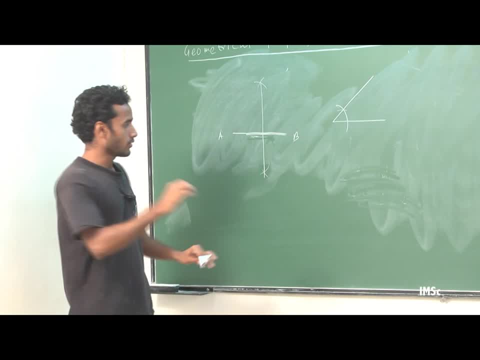 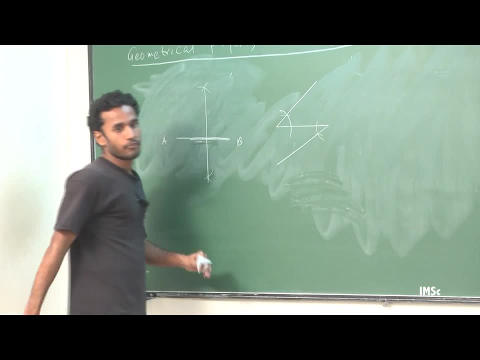 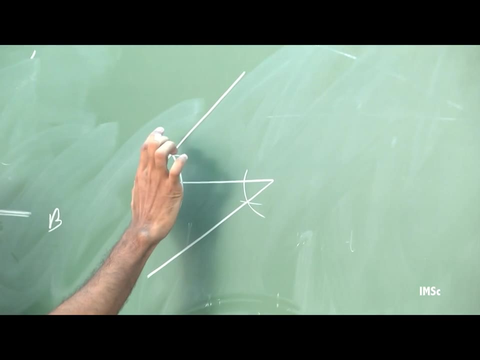 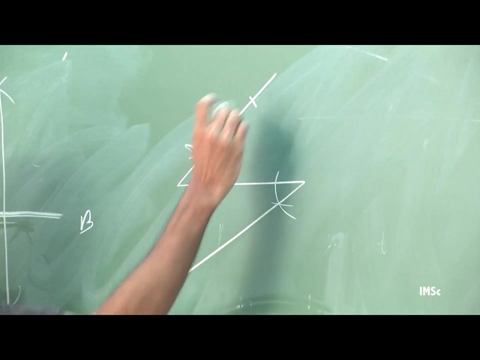 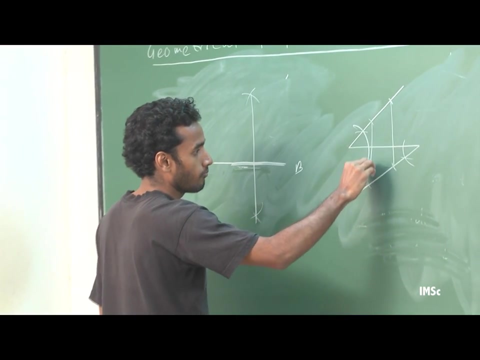 with pencil compass. Similarly, draw a angle here. The same angle. Draw a angle here and draw a same angle here. Now take any arc length and cut it. and the same arc length and just cut this side. We do this same arc length and again from this same arc length. Now join these two points. 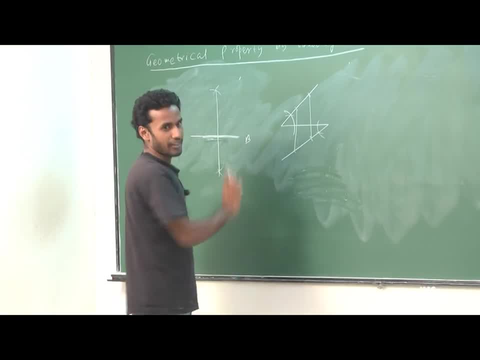 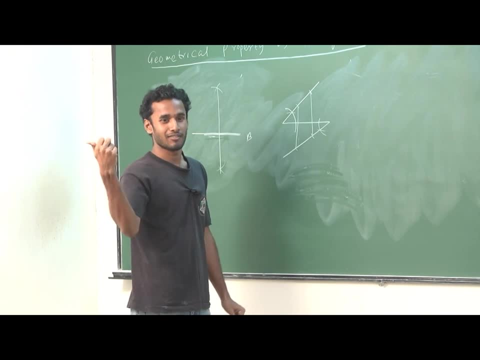 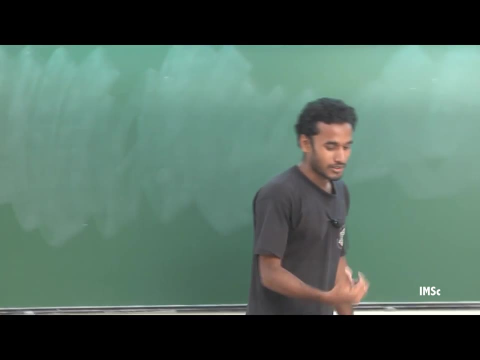 My claim is that it trisects this line. Similarity between triangles. So you will prove me in the Break session. Break session. I will just ask you for this proof Why that is true, Why that is trisection of a line. 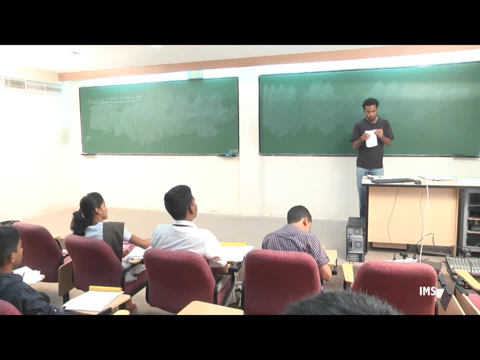 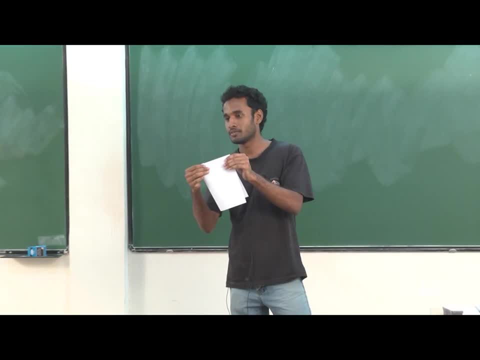 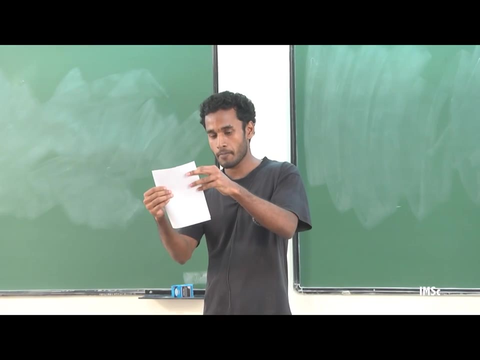 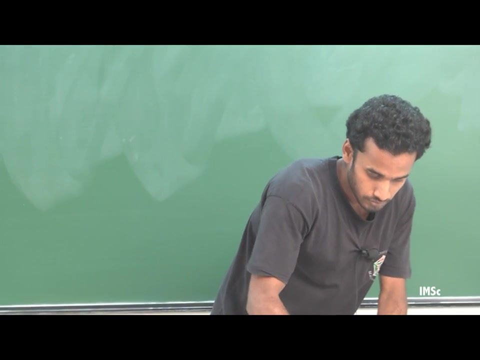 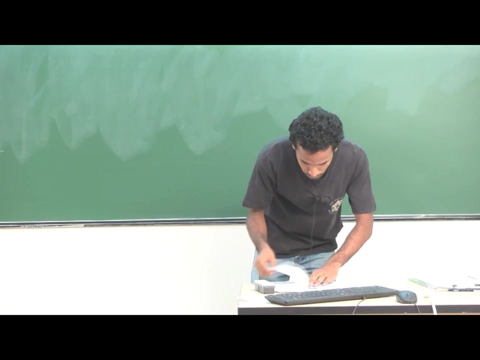 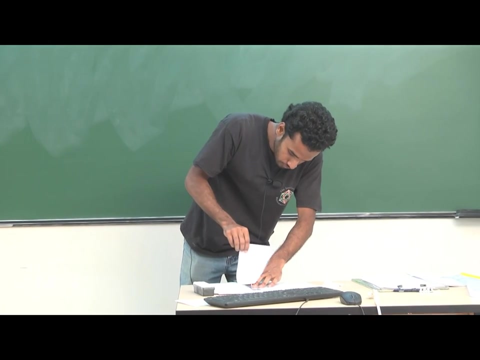 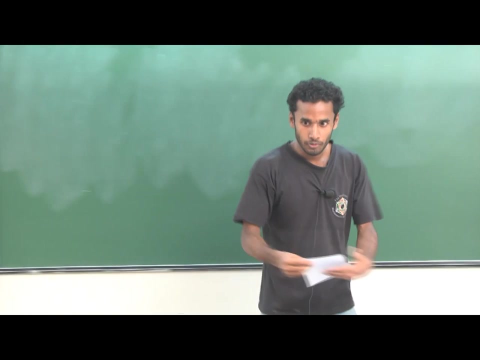 Now, this is a rectangular sheet of paper. So from here, cut a square sheet of paper. How to do that? Just make it half. You can just make it half, and it is also a rectangle, right, Yeah, Now make a diagonal. 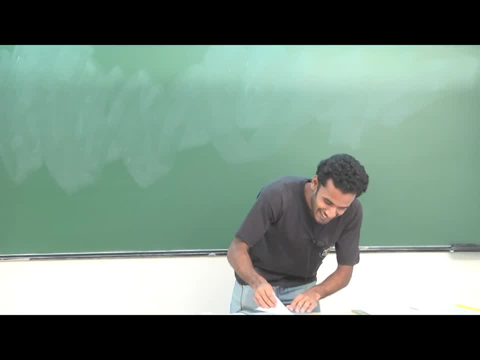 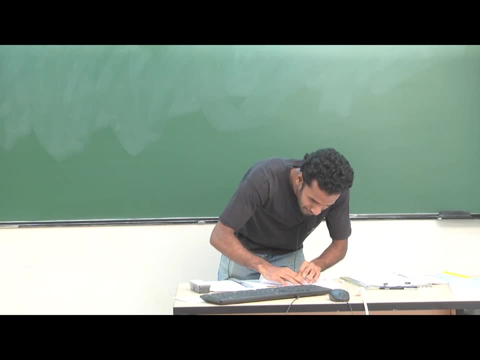 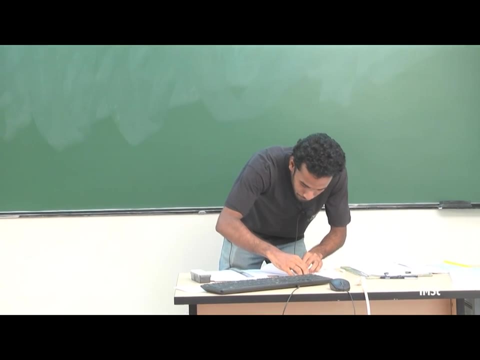 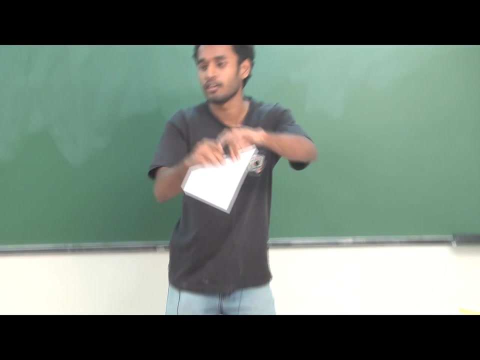 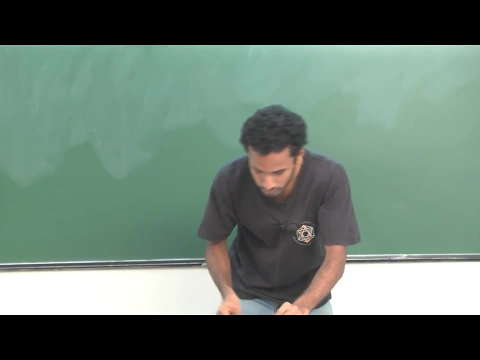 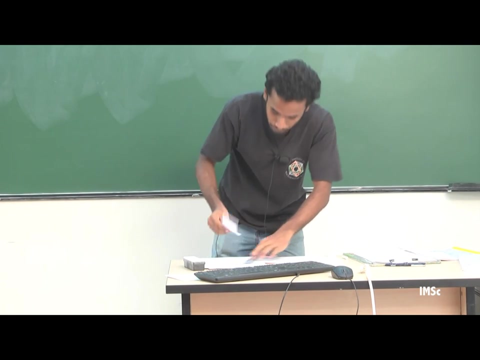 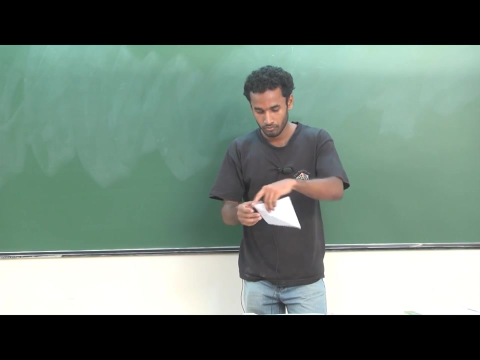 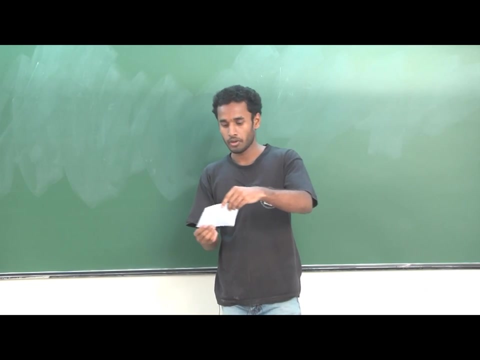 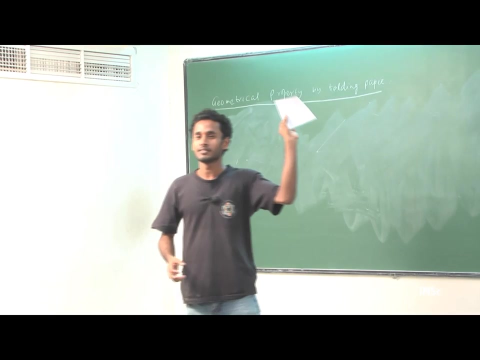 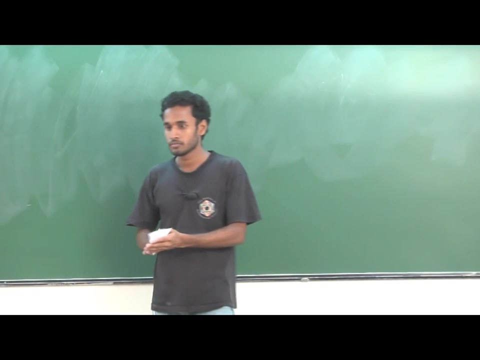 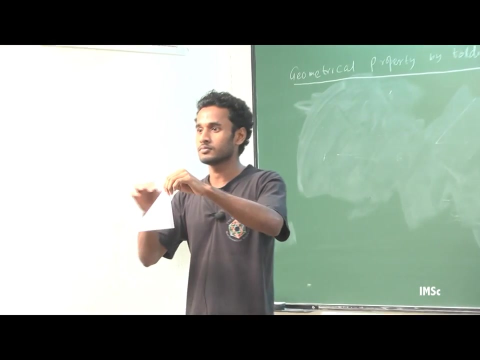 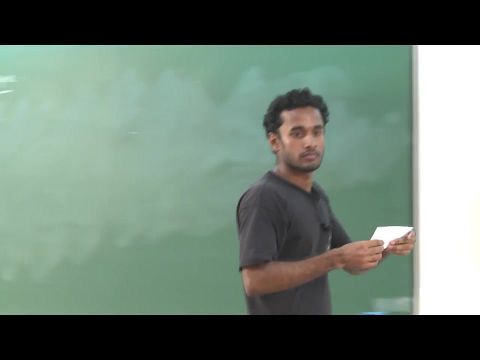 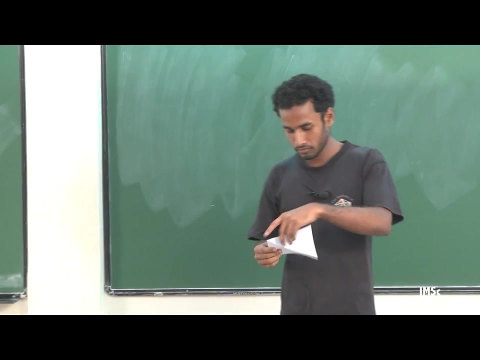 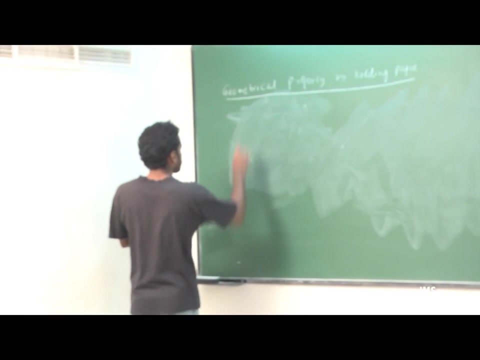 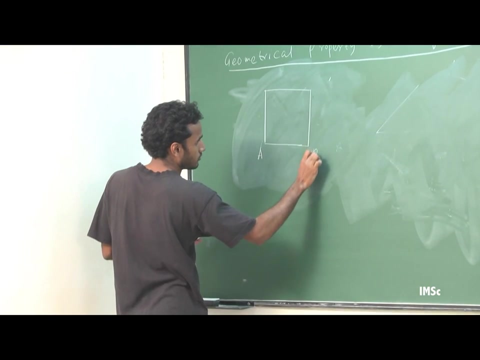 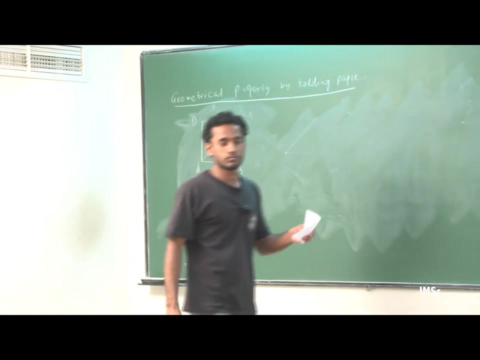 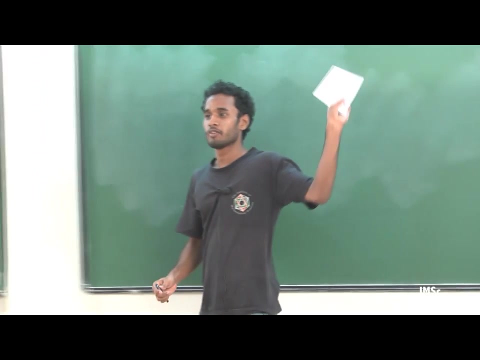 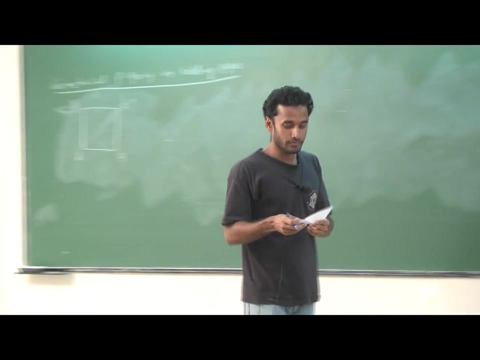 Make a diagonal. Yeah, Good, And make a diagonal. Make a diagonal and then cut along this line. Right has cut this square piece of paper. take your time. Everyone has cut this square piece of paper. Everyone has done this. Now, with your pen or pencil, make a line along this diagonal. 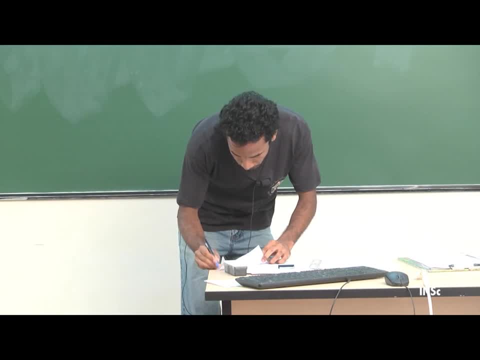 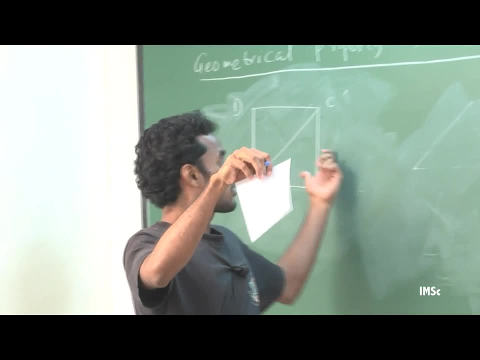 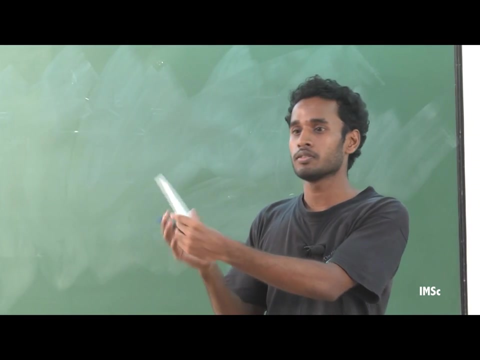 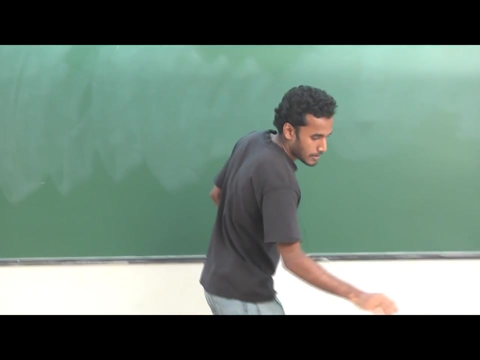 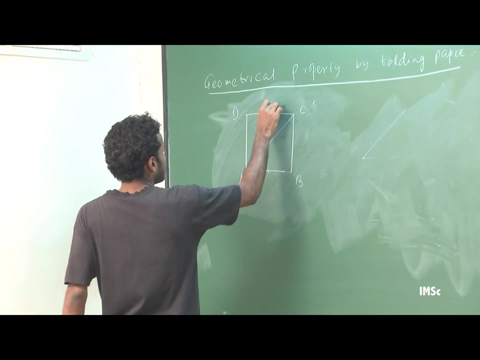 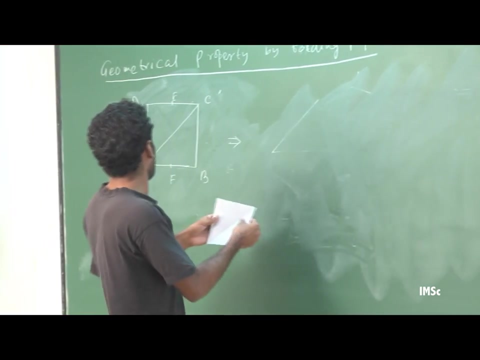 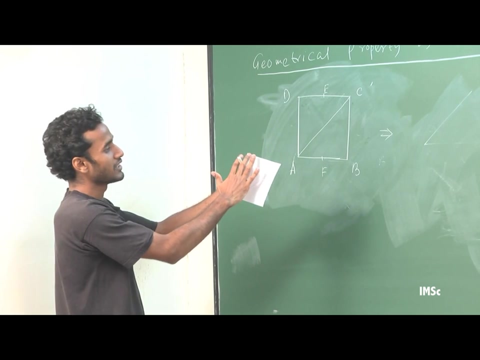 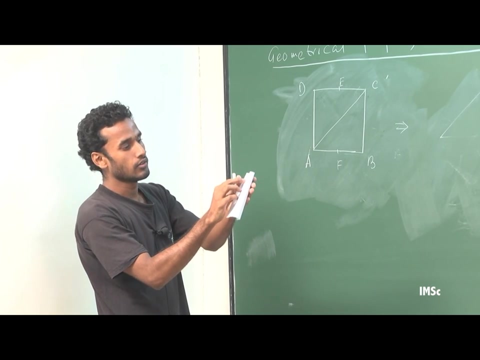 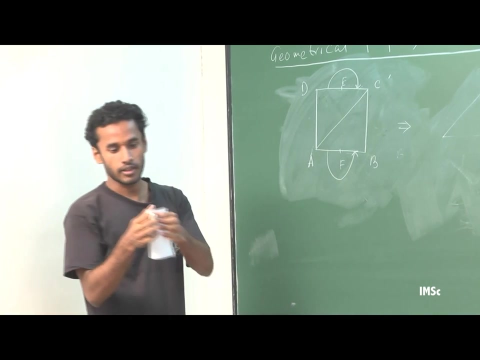 Just draw a line along this diagonal like this: Everyone has drawn a line Now fold with respect to this line, Respect to the middle point of this side, CD and AB. How to do that? Just to this one, such that this line coincide with this line and this line coincides with this line, like this: 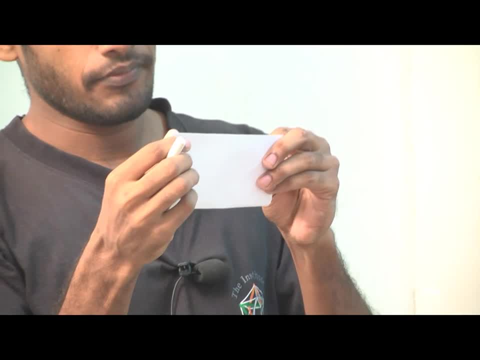 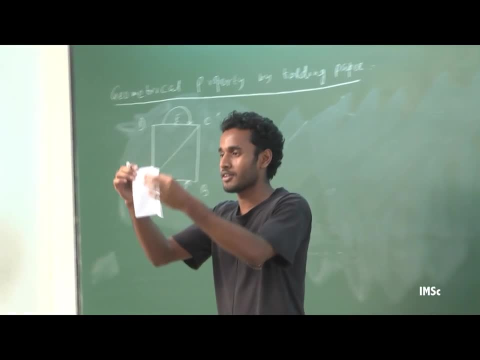 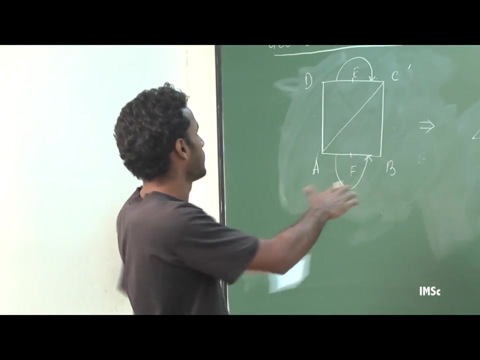 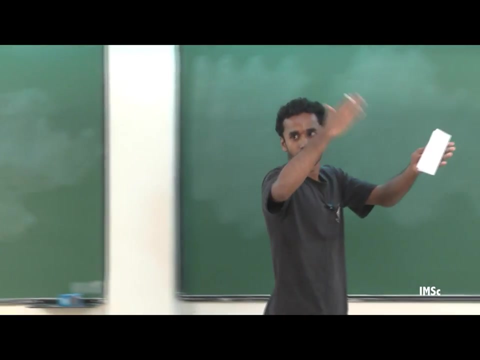 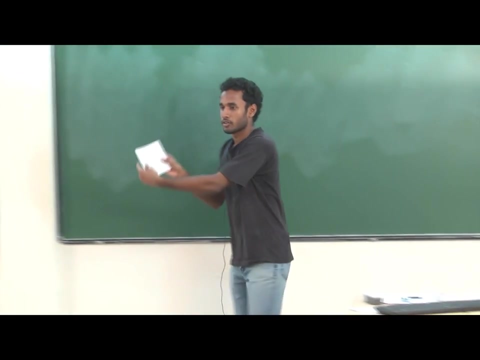 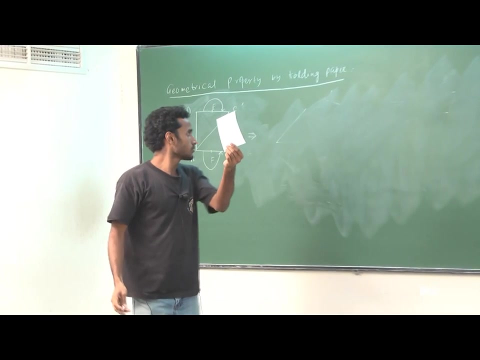 Do it carefully. All of you have done this. So you have created 2 small rectangles with respect to this line, EF, and again draw a line along this folded line like this. Everyone has drawn this. So what have done? This is ABCD, this is EF. 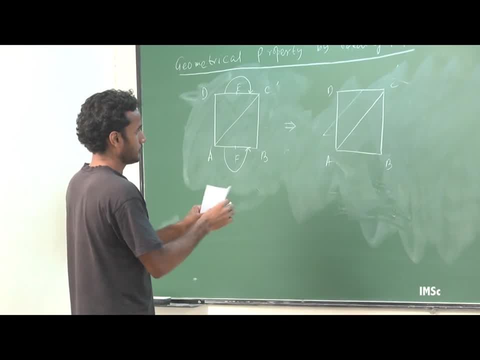 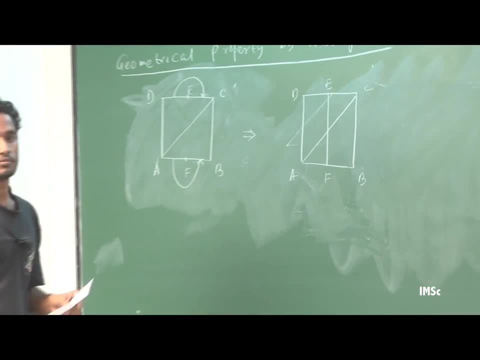 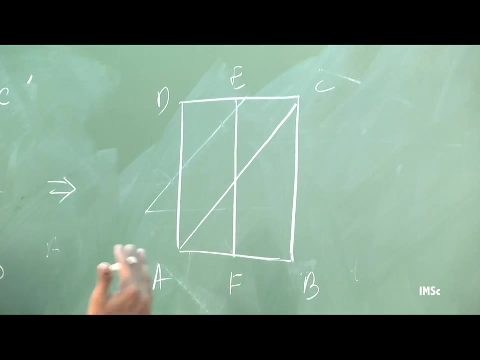 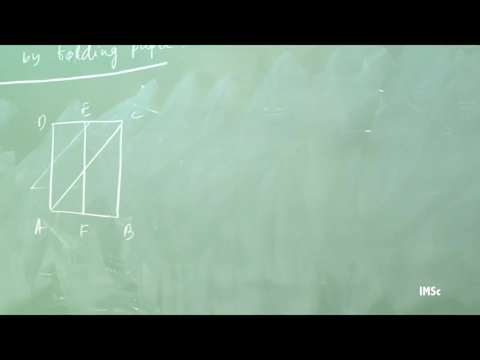 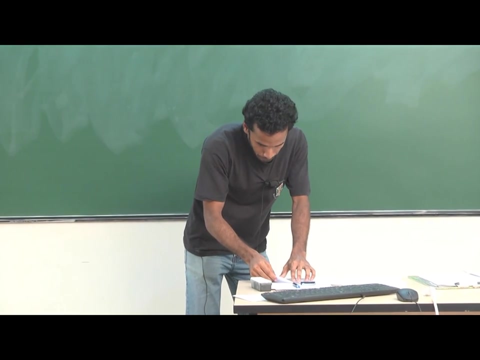 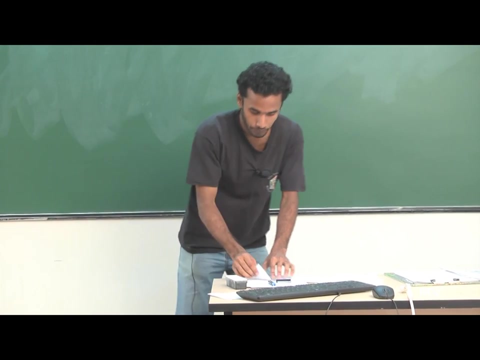 So this is EF. Now fold along with the diagonal of this rectangle, F, B, C, E along E B. Fold it along E B, or just draw a line along E B. You can fold Once again. I am just telling that. 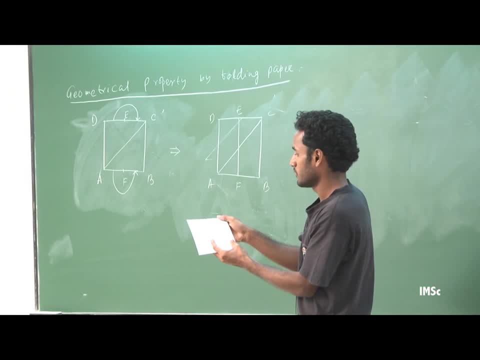 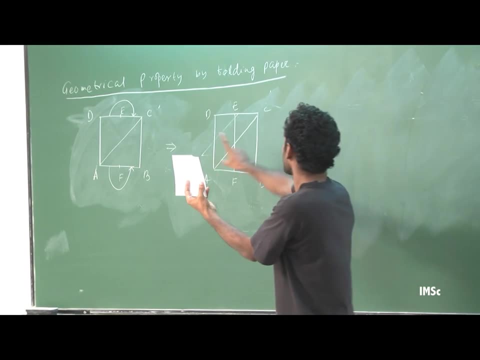 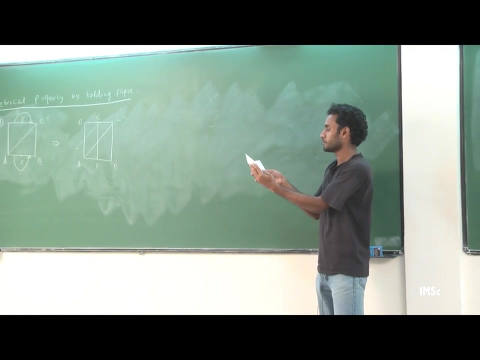 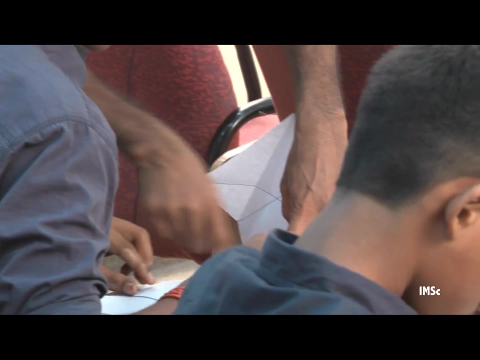 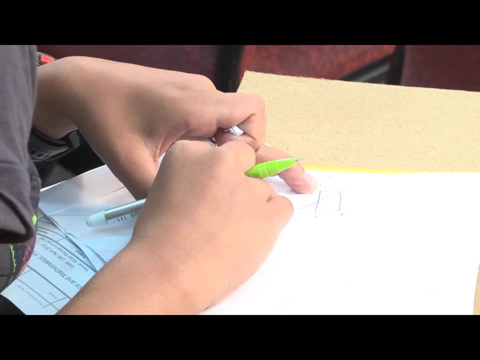 Just fold along the diagonal of this rectangle F, B, C, E, along E, B, The diagonal of this rectangle E, F, B, C. Just draw a line. You can draw a line also. Just draw a line like this. 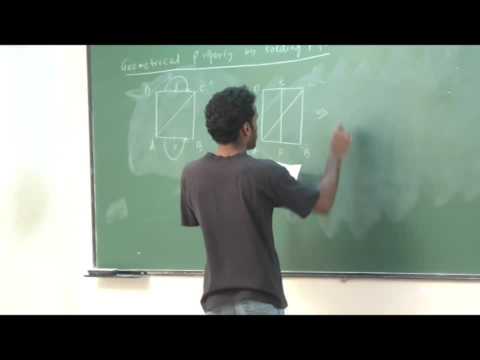 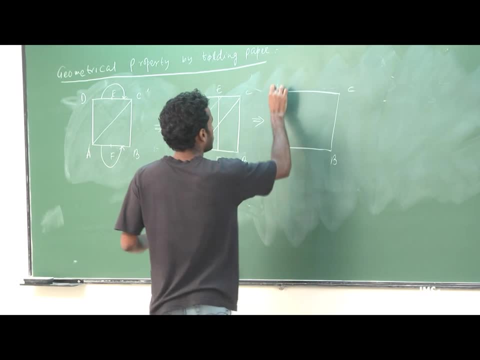 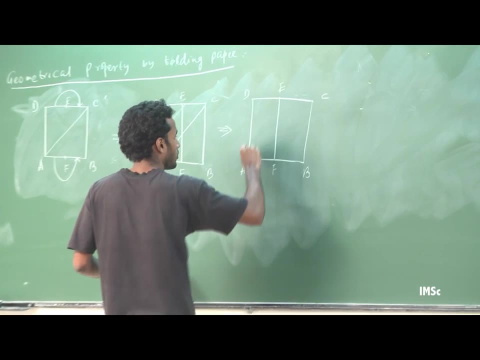 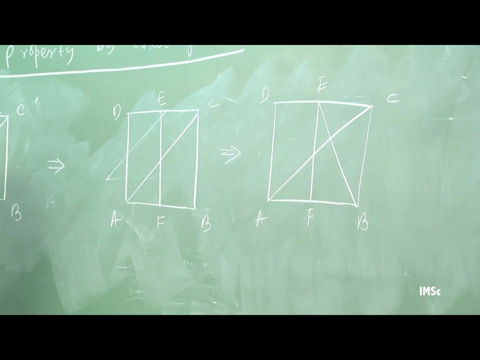 So okay, After this what I have done, This is my square. This is the rectangle E F. This is the first diagonal of this square. This is another diagonal of this rectangle. Everyone has drawn up to this. Yes. 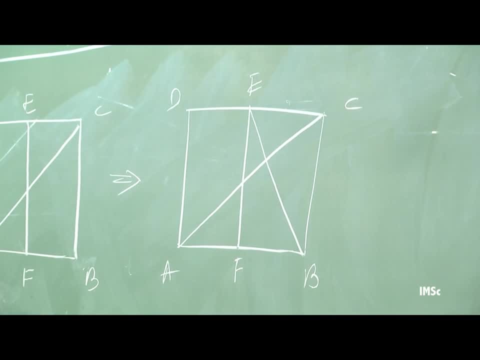 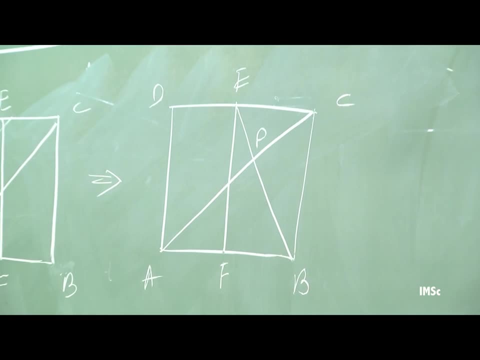 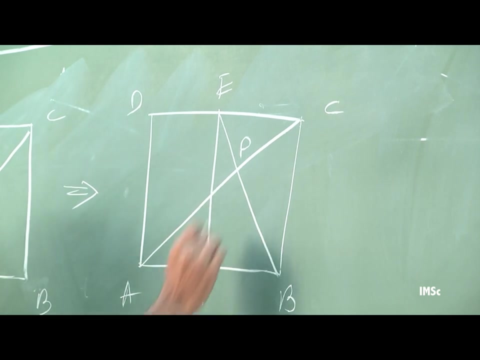 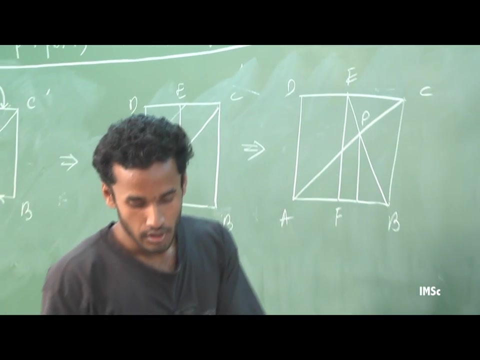 Everyone. Yes, Yes, Yes. Okay, Now let me call this point as P. Right Now, draw a perpendicular from P to the base A, B. How to do that? So if you fold the paper such that this line coincides with this line, 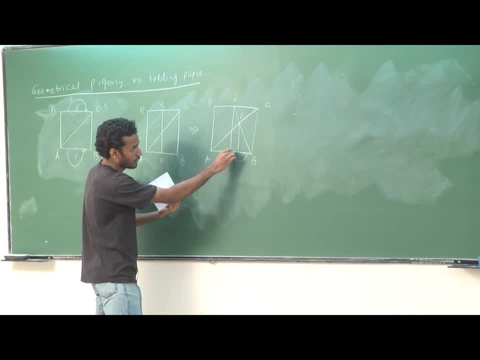 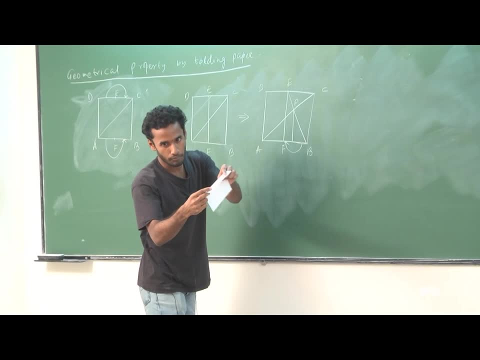 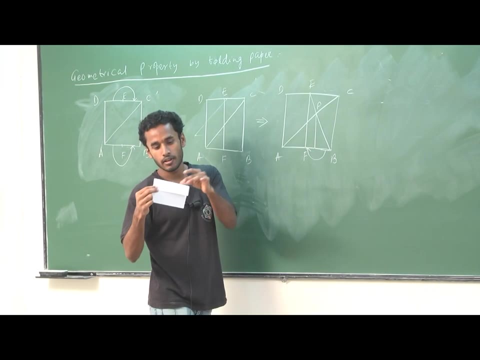 Coincides with this line and it passes through P. So how can you do this? Just if you just look at the, just fold it in back side such that these two lines coincide like this and it goes through the point T like this: 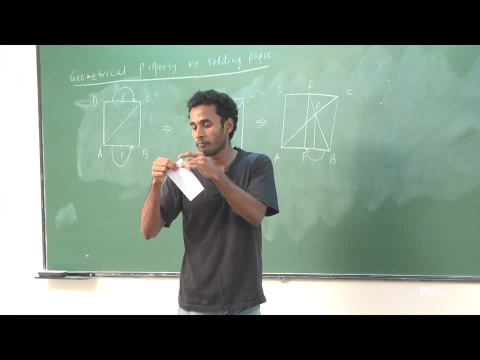 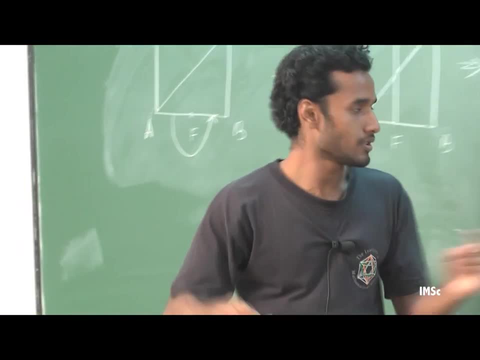 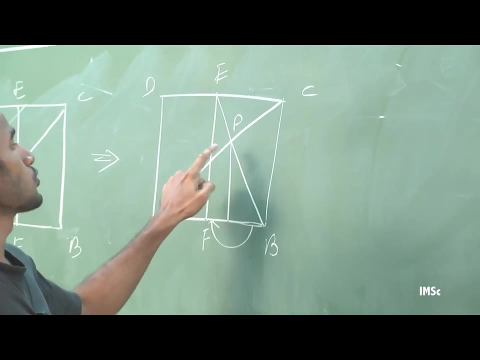 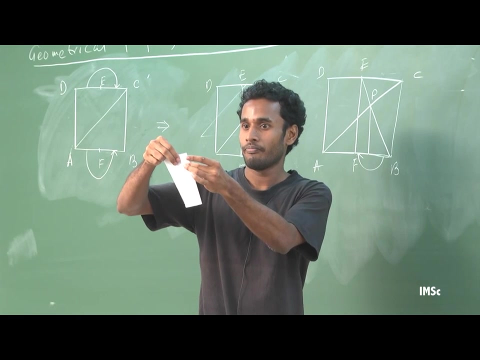 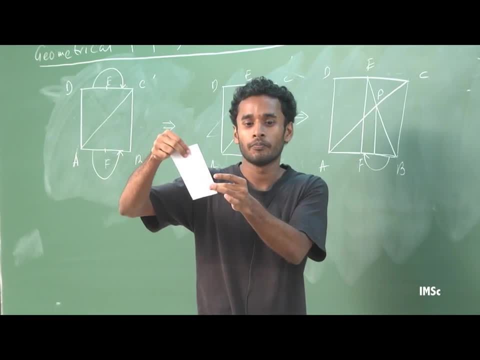 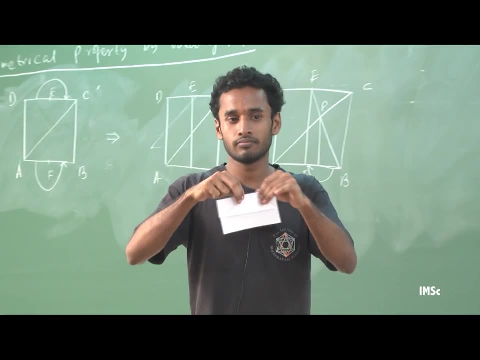 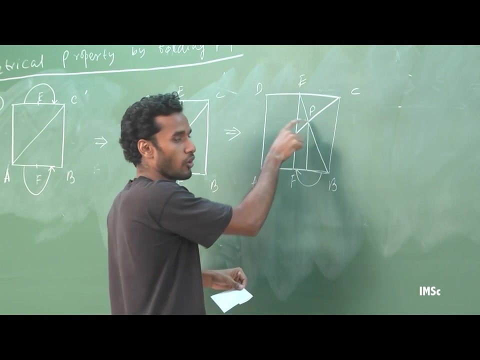 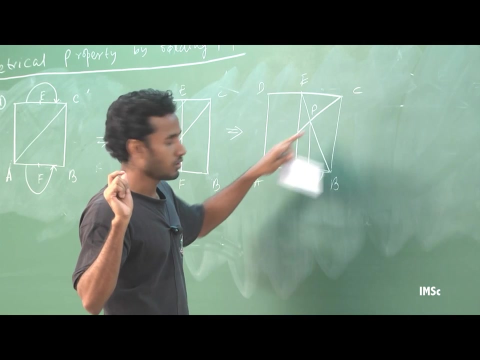 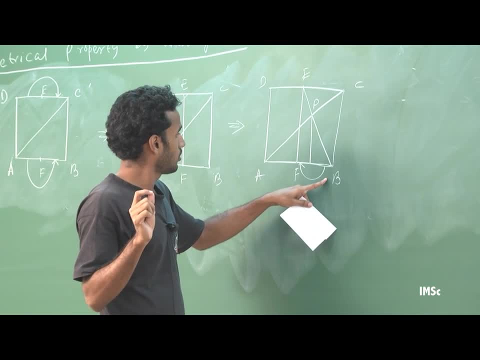 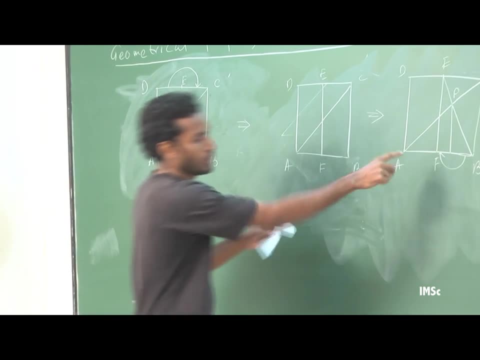 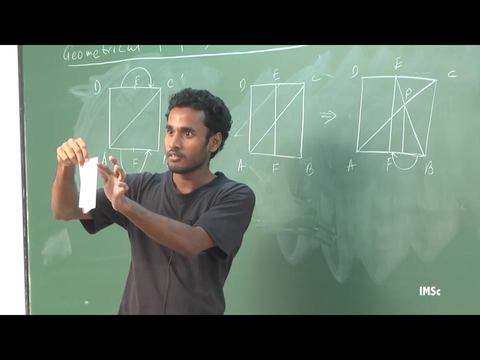 No, You can draw perpendicular from any point, right? Yes, So that is P need to be that. Sorry, Does B need to be that? P need to No, B. B need to be that you can do it by taking this piece of paper like this, such that this line passes through: 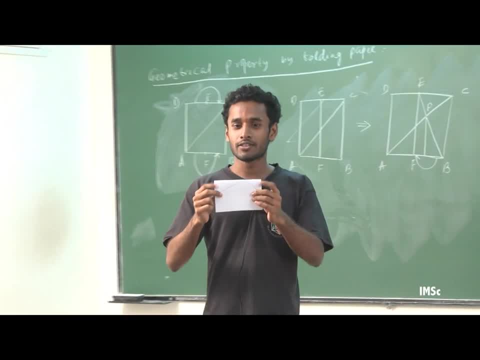 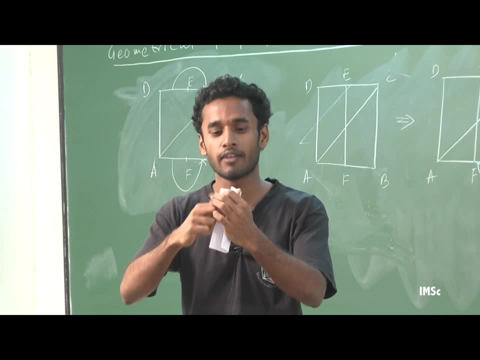 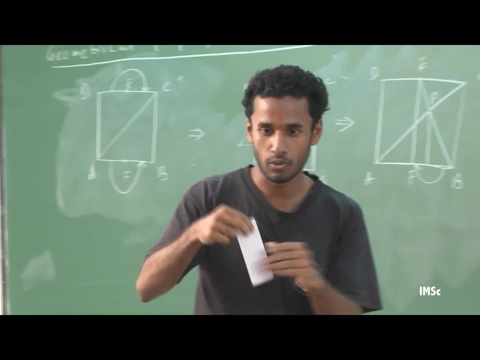 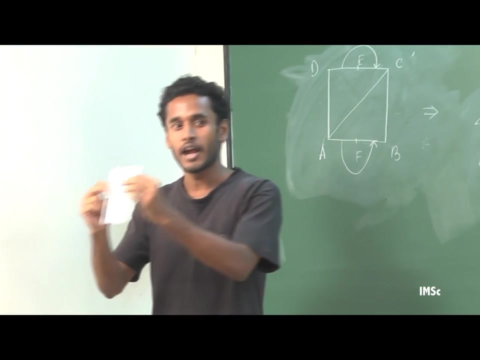 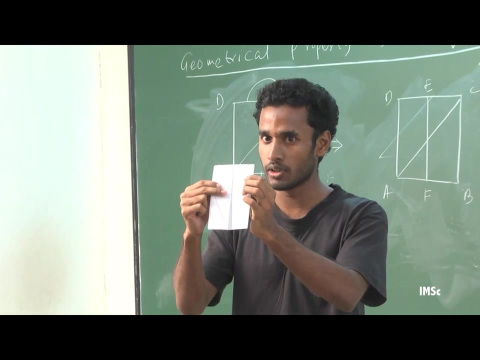 P, then fold it once more with respect to this line, like this, and make another fold. Let me tell you once again: I have fold it with respect to that perpendicular and fold it once again with respect to this line. at first, fold that perpendicular, create that perpendicular. 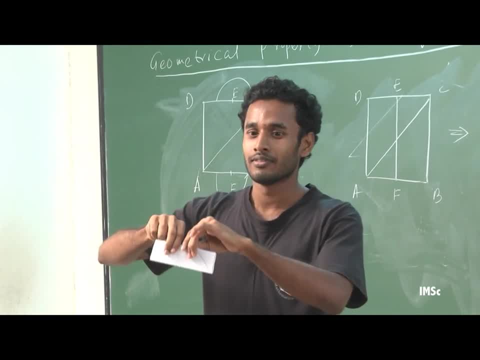 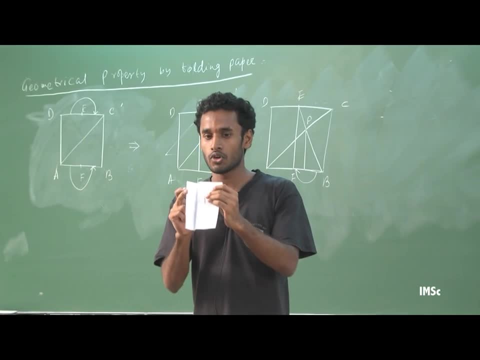 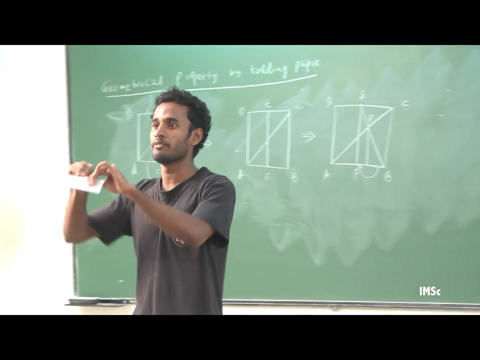 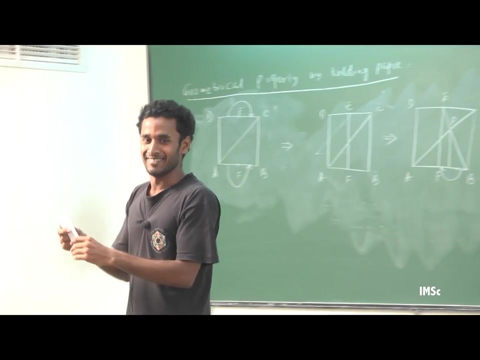 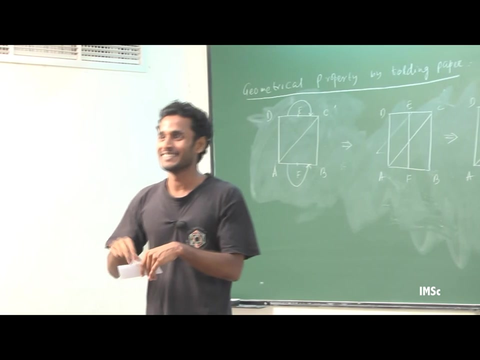 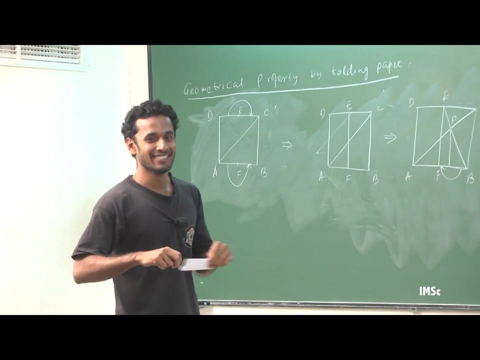 again. just fold it like this. Just draw this perpendicular and again once again fold like this. Everyone has done this. I am not getting anything. It is trisected, Diagonal trisected, No, not diagonal trisected, exactly. Have you got anything? 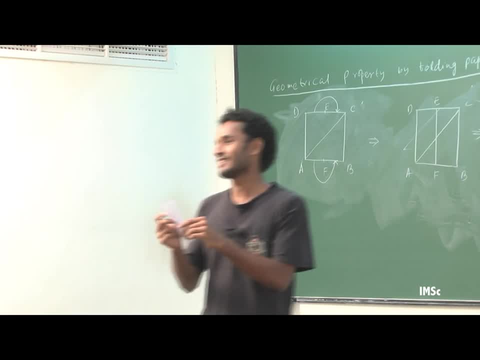 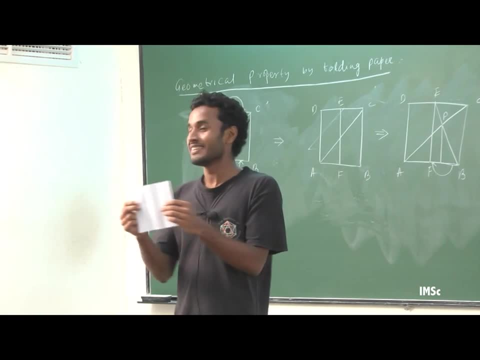 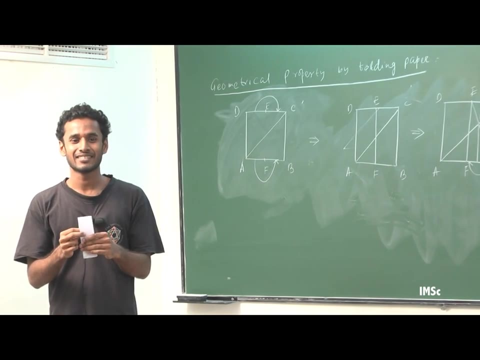 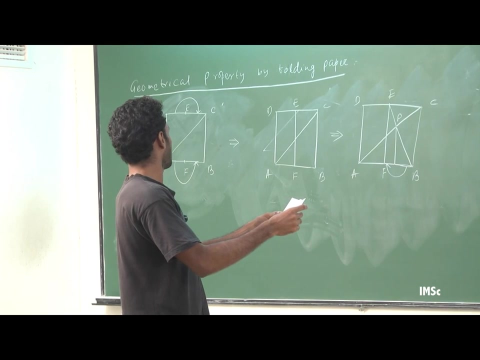 Which line gets trisected? Diagonal of the square. Diagonal of the square, Not diagonal, Not diagonal, Not diagonal. You have just Diagonal, sir, Diagonal angle side. Very good, I am not sure about that diagonal, but it is clearly. 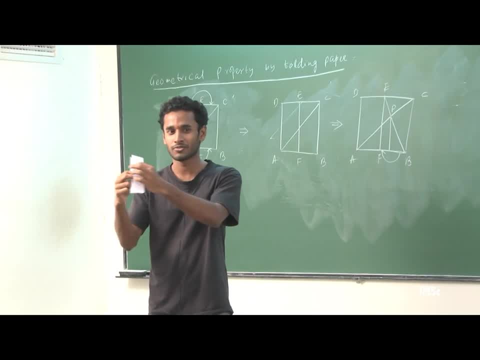 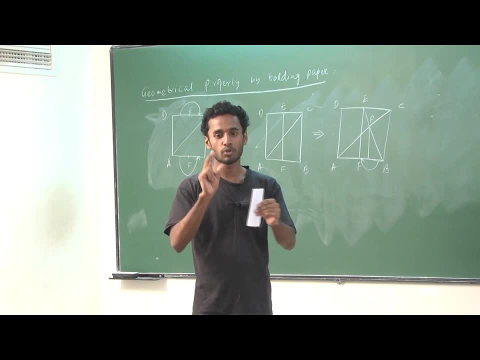 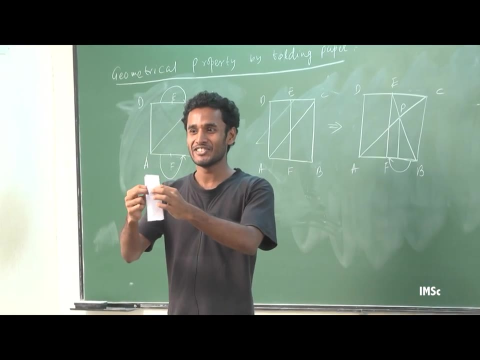 seen that these lines are getting trisected because this fold, this fold, this fold, Even the tiles and tiles, The ratios. That may be true, but I am going to trisect this line So you can see it clearly, right. So why that is true, Why it gets trisected? 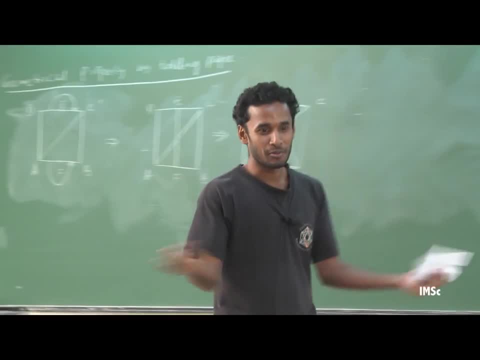 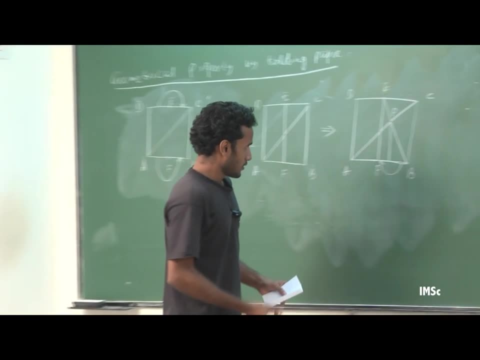 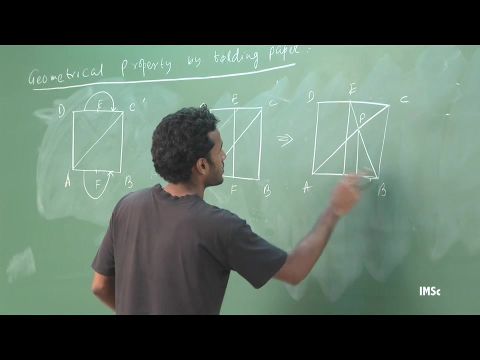 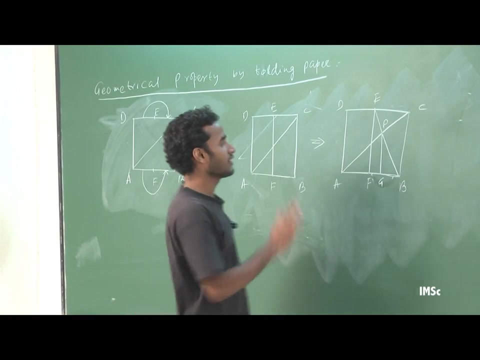 I have just told you to do some fold. do something and you will get trisected. The line will get trisected, So let me just erase it. Let me call it any name, maybe CDEFG? So why that line gets trisected? 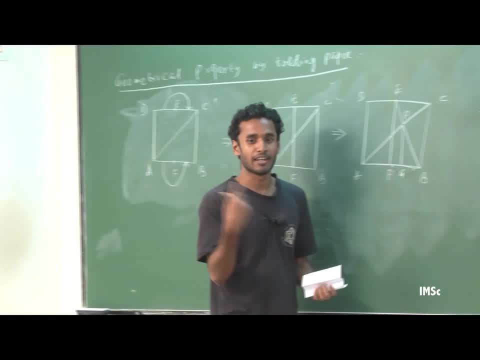 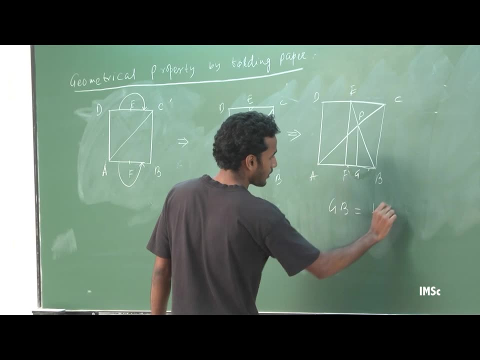 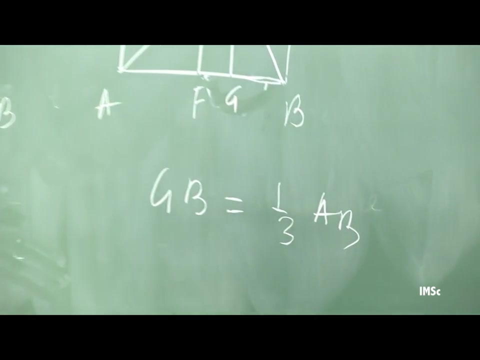 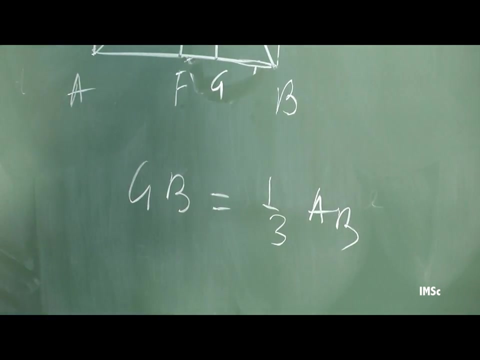 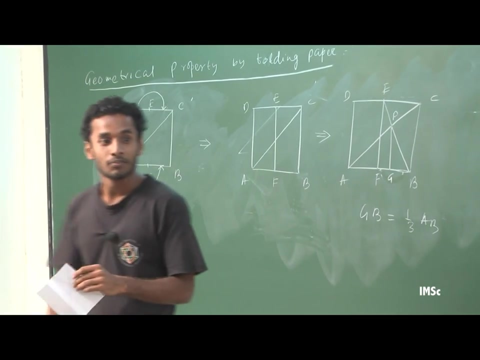 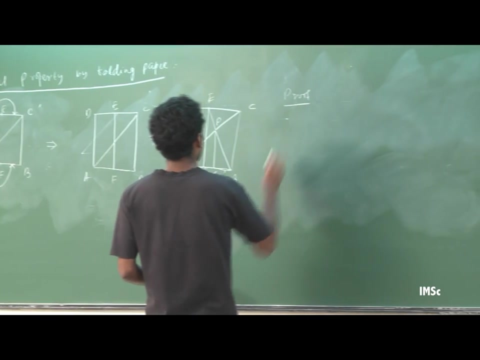 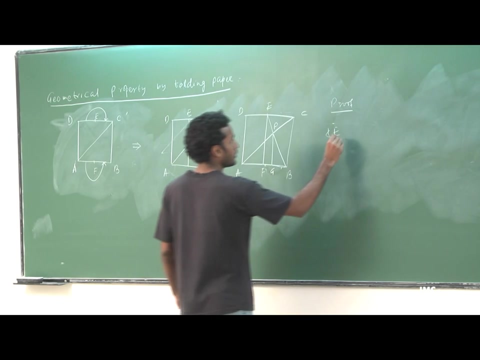 What is the proof of this? What is the reason behind that? Anyone, Any guess, Anyone. So b should be one third of a, b, and you will see this because this is one third, exactly, this is right. So why that is true? What is the proof of that? So we can use similarity, Similarity again, Yes, what is proof? So look at this two triangle, this triangle: E, F, B and 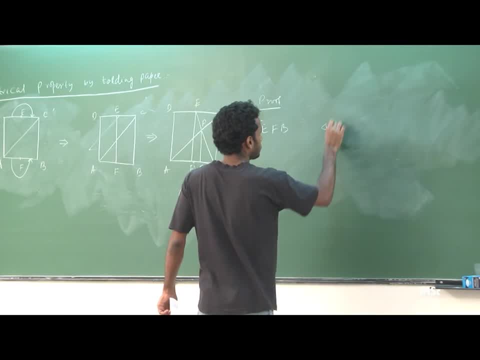 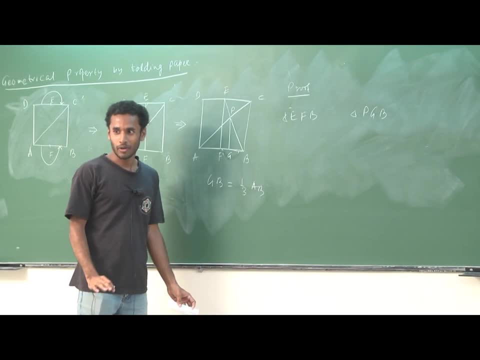 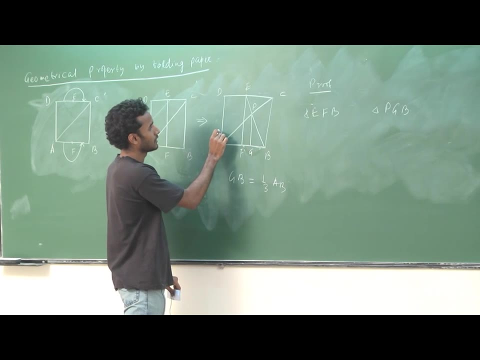 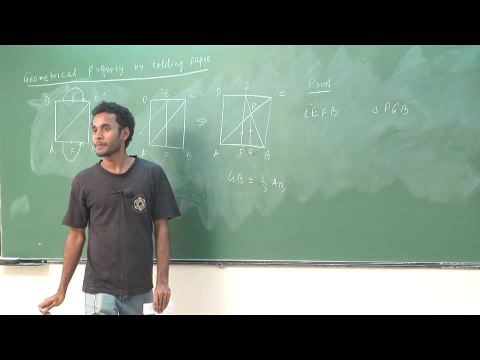 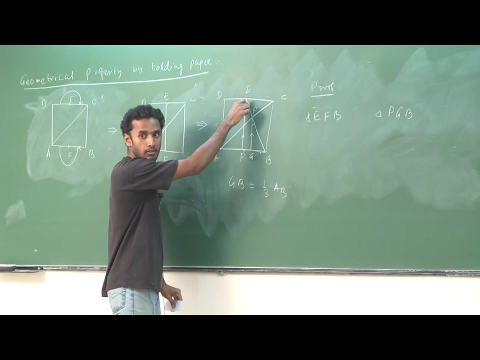 triangle: P, G, B. right, They are similar. Why? Because this line is parallel to this line. everyone agrees with this. Yes, Right, because both are perpendicular, right? Yes, For that reason, this angle, This angle is equals to F E B. 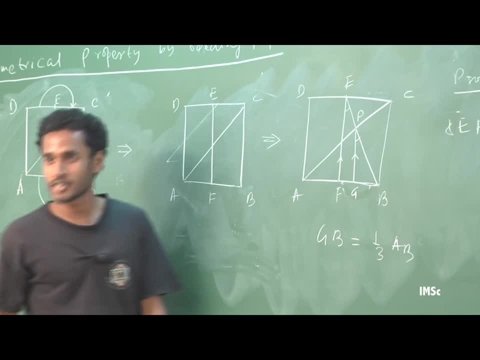 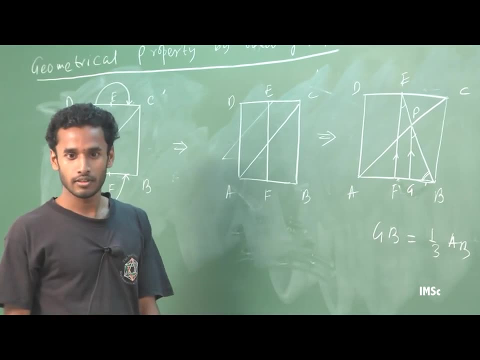 F, E, B. Good, This angle is equals to this angle. Yes, And this angle is common. Yes, Yes To both. and this is ninety, Ninety, Ninety, Right, Yes. So this, this big triangle and this small one. 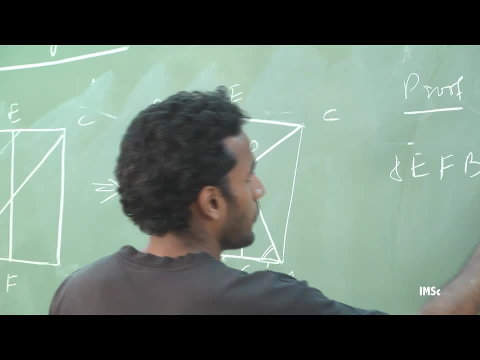 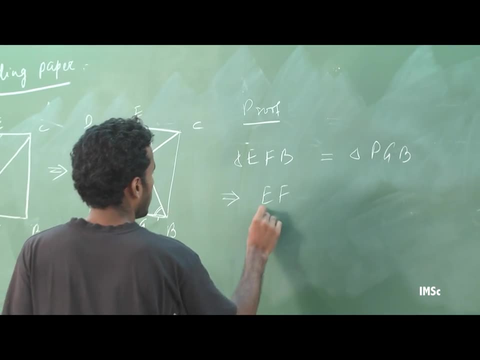 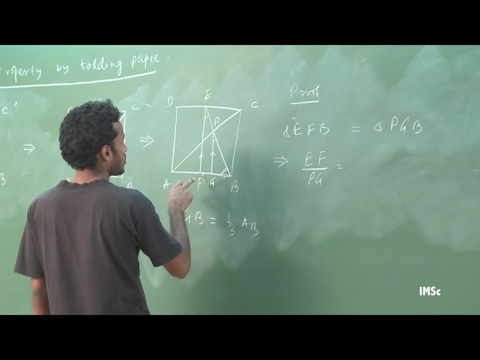 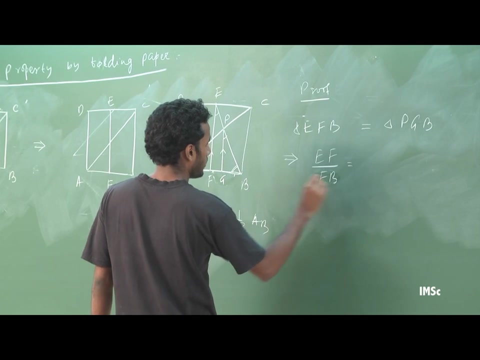 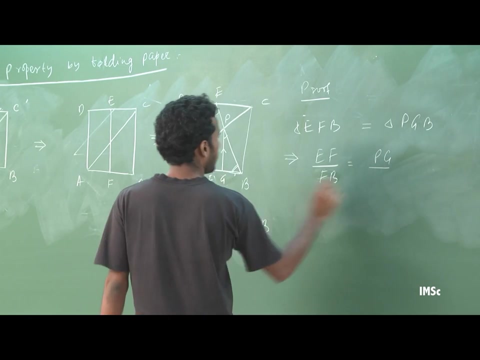 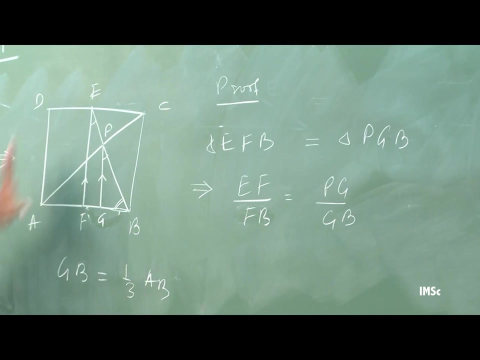 Small triangle Are similar. Yes, So by the properties of similarity triangle. then I can write: E? F divided by P- G, P G equals to E? F divided by F- B should be equals to P G divided by G B. It is right, right, What I have written there. E? F divided by F- B should be equals to: 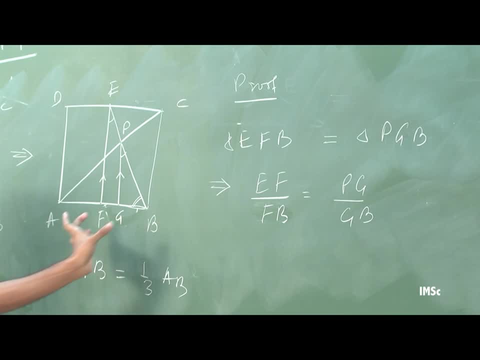 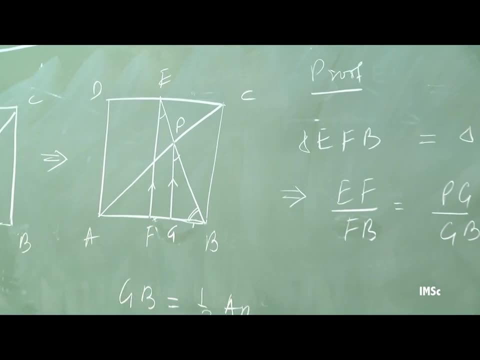 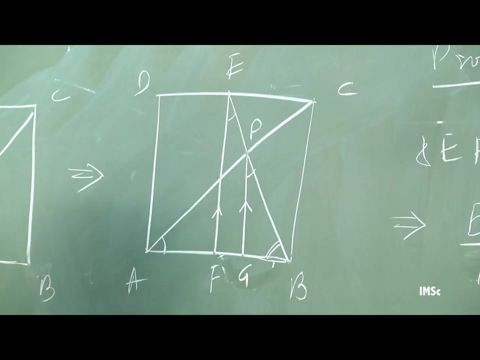 E, F divided by F B should be equals to P G divided by G B. Right Now, look at this triangle: A, G, P, This small triangle Similar to that. This angle is similar to which angle Like this? What is this angle? 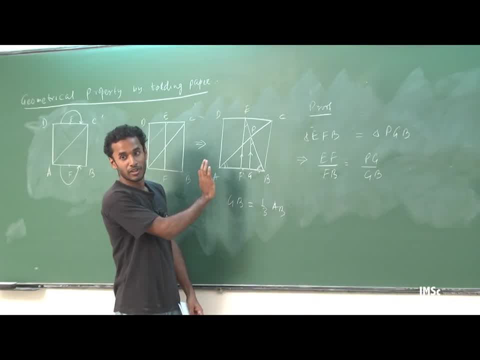 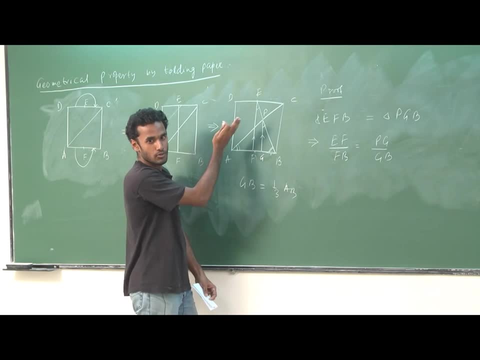 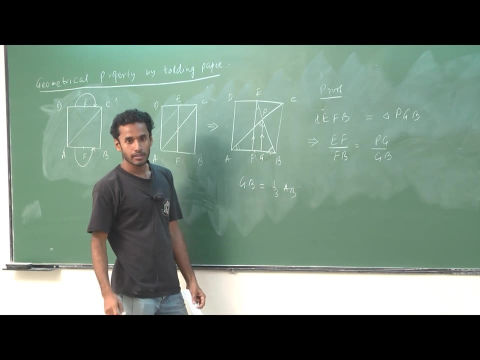 this angle, it is how much? Forty five. Forty five, Good, because it is bisecting a square, and for that same reason this is also forty five, because I am drawing a perpendicular from here, right? And for that reason a g should be equals to g p, a g equals to p g. 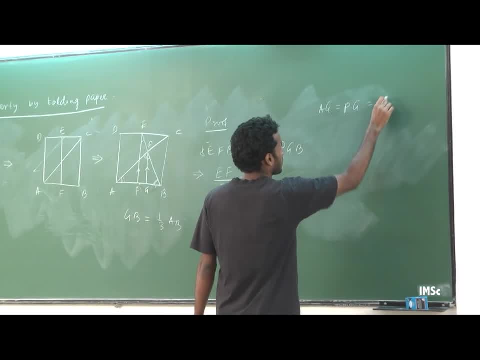 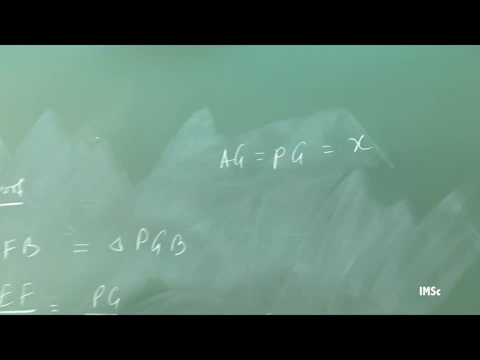 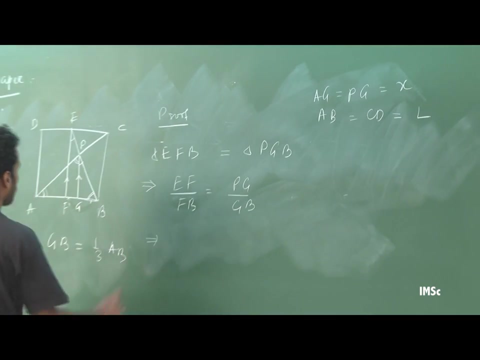 call it p, g. Let it take x, a, g equals to p, g equals to x. and let me take the length of this square side of this square: a, b equals to c, d equals to a, g. The length of this square is l. right Now, just put it. What is e, f? e? f is same as a. 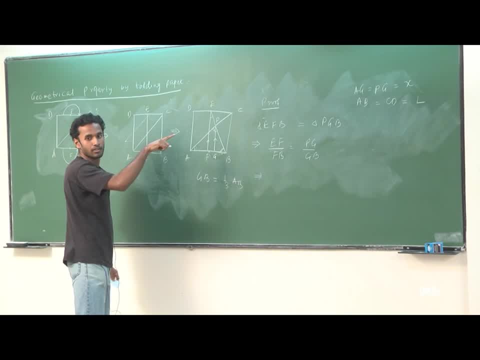 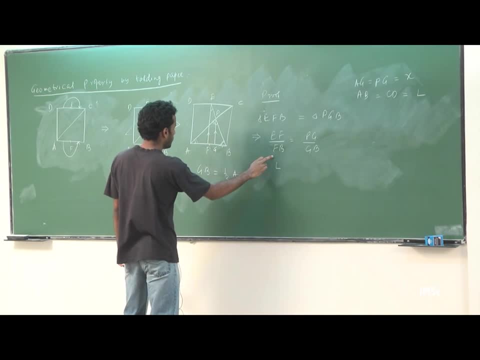 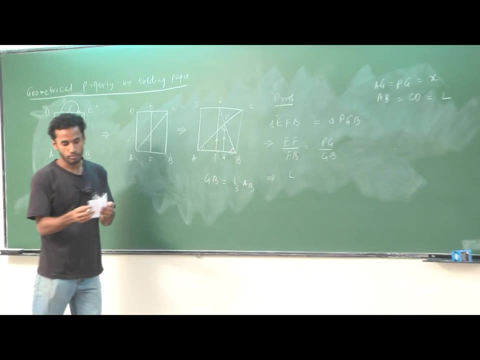 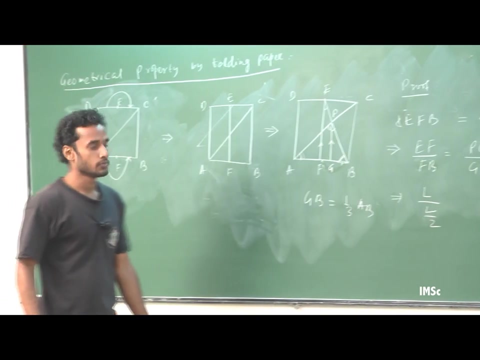 d right. a d is same as c? d because it is a square, So it is l right. What is f b? f b- this is half of a b because I have folded it half Right, So f b is l y 2.. Okay, yeah. 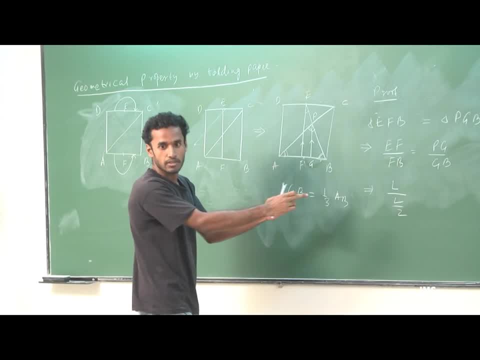 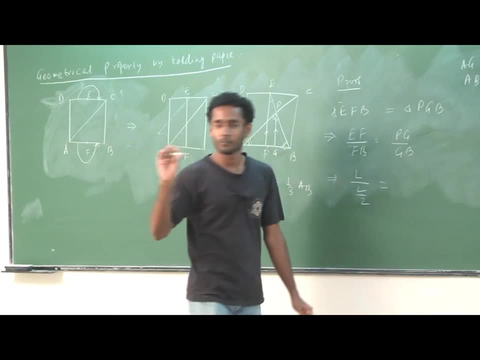 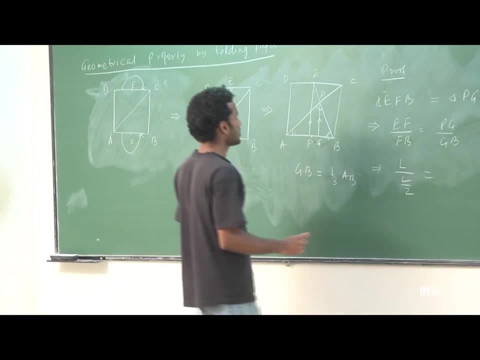 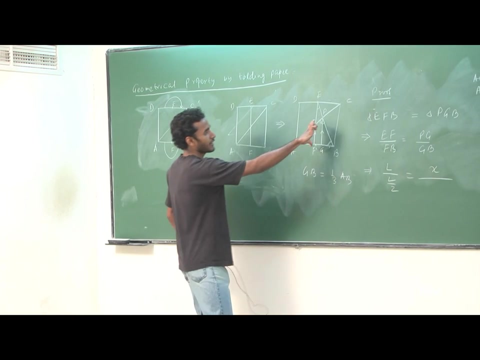 f, f, e is l y 2, right, Everyone is following me. Yes, sir, Yes sir, Okay. And what is p? g, p? g is x, x, And what is g, b, g, b? This is x, p, g is x, a, g is also x because of this. 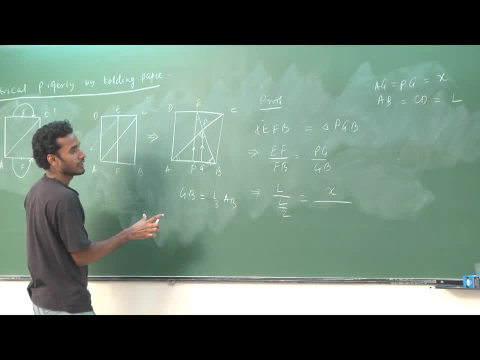 g b. What is g b This? this is 1 by 3.. 1 by 3.. 1 by 3.. a b minus x, a, b minus x, a b minus x. Yes, sir, What is a b? a b is l. 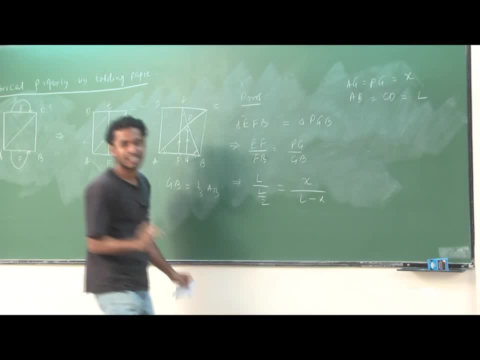 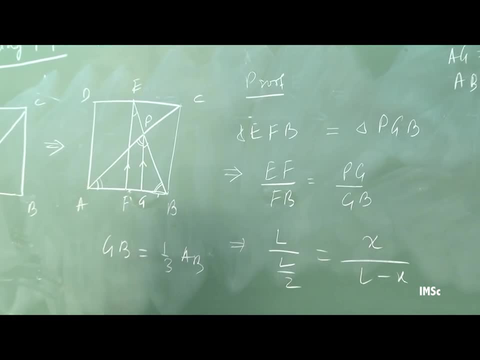 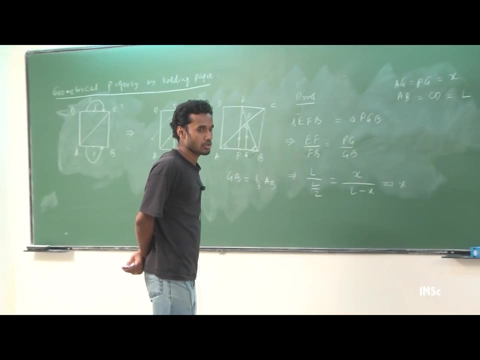 a b minus x, l minus x, l minus x right. So g b is a b minus a g and a g is x, l minus x. Now solve for x. I do not want to solve that. Tell me: x equals 2 in terms of l, 2 l. x is 2 l. 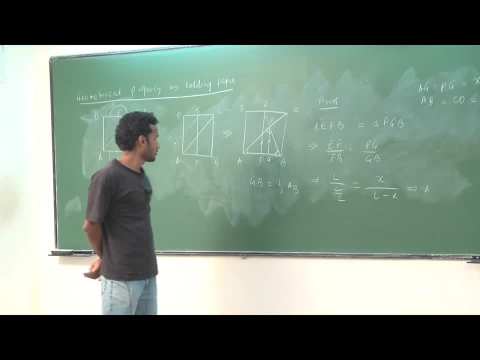 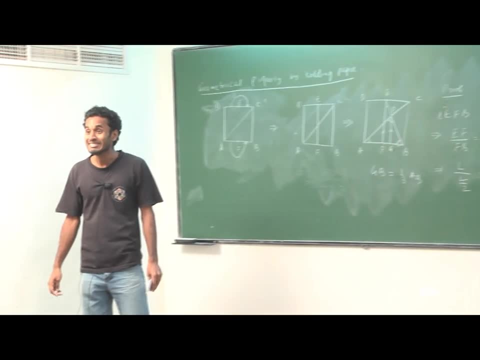 x is 2 l. At first that is not possible because x is inside l 2 by 3. l sir 2 by 3l. sir 2 by 3.. Sir 2 by 3. l 2 by 3l. 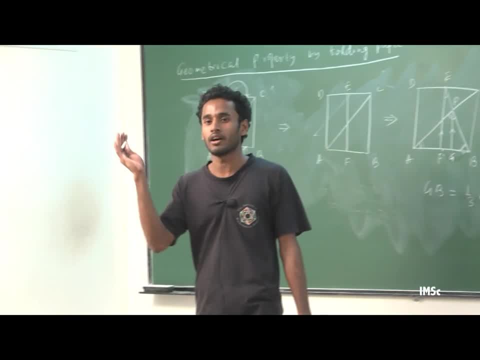 Sir, sir, Sir sir. 2 by 3l, 2 by 3l, 2 by 3l, that is correct. 2 by 3l and another. any other answer? l? l, 2 by 3l. 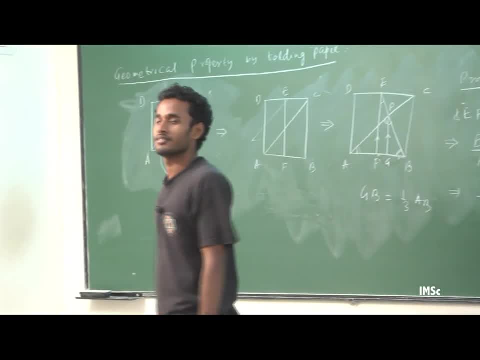 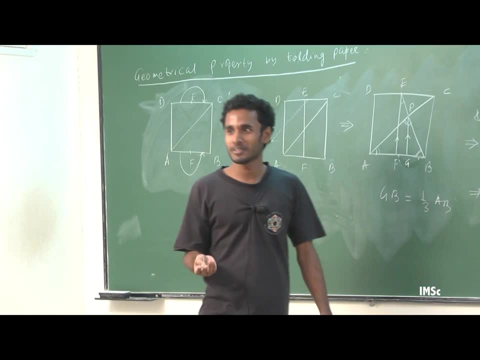 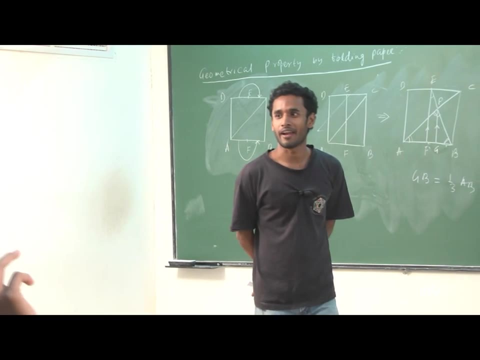 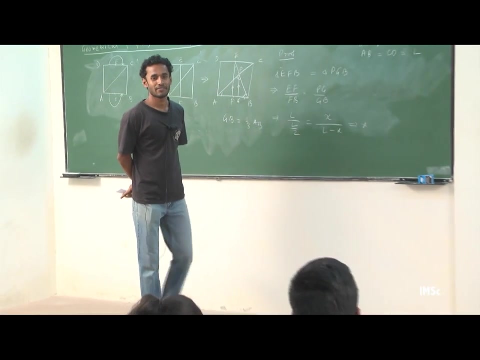 2 by 3 l and now and 2 l by 3.. 2 l by 3, It is so simple: 2 by 3 l. what 2 by 3 l? So how many 2 l of by 3? raise your hand, man, just. 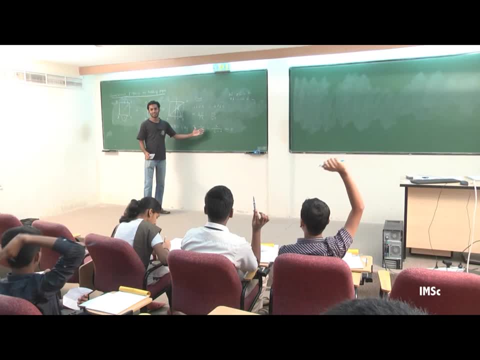 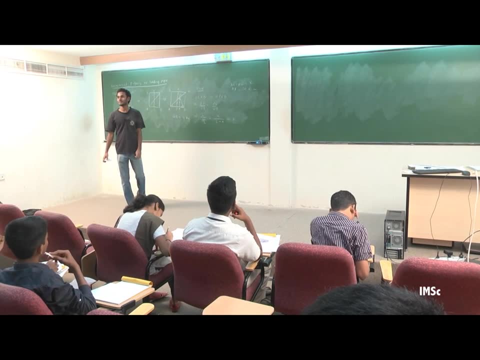 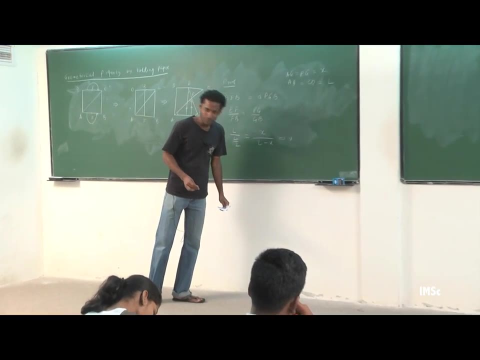 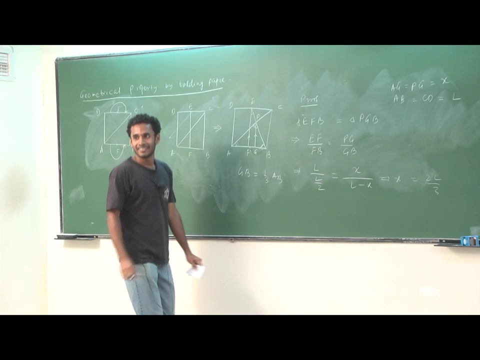 solve for x. this is so simple for 10 standard, So good. x equals to twice l by 3. right. So d g should be l by 3.. d g should be l by 3. d g should be l by 3.. So d g should be l by 3.. So d g should be l by 3.. So d g should: 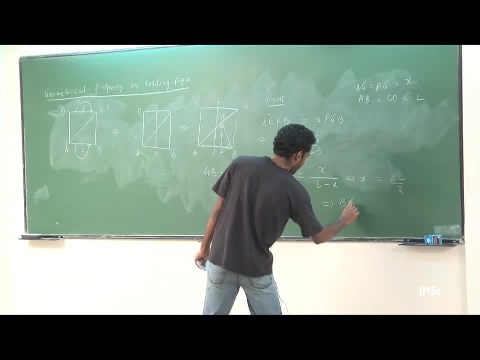 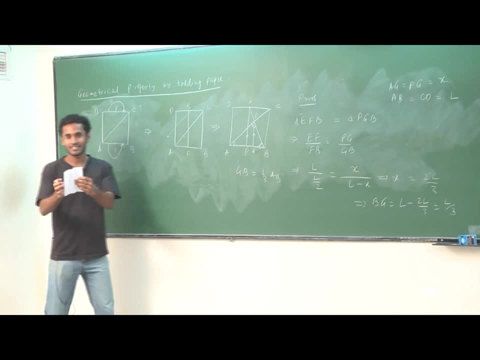 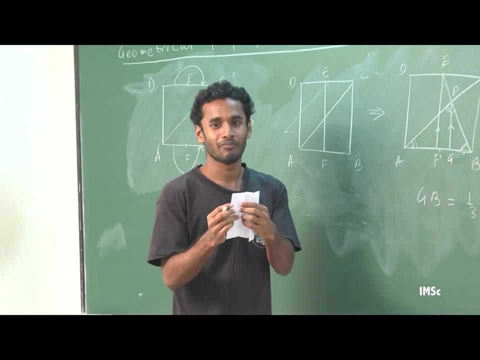 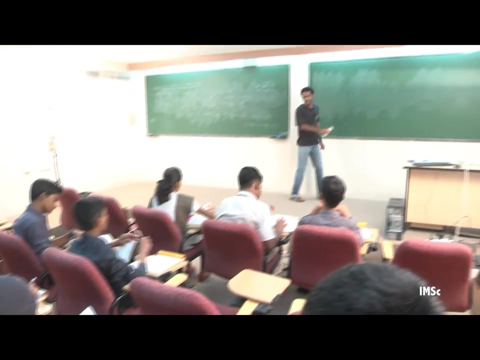 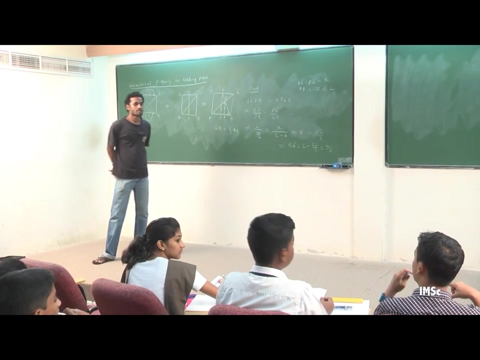 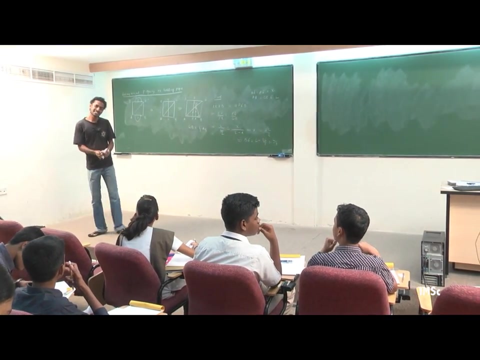 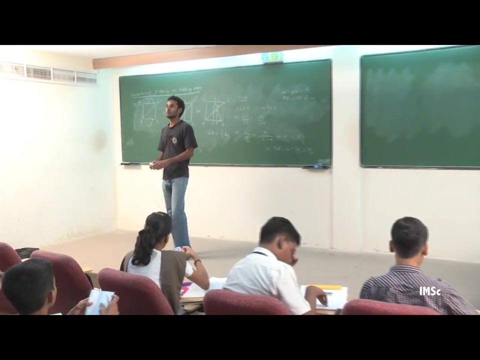 be l by 3.. Good, very good. d g should be l minus 2, l by 3, this is l by 3. for that reason it is trisected. So now, how can you get the one fifth of this line, 5 equal marks. No, I want to do what, just tell 3.. So now the question is how to get. 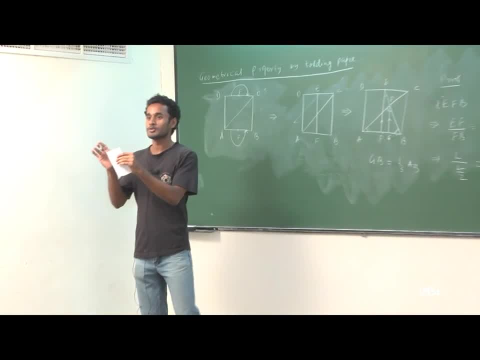 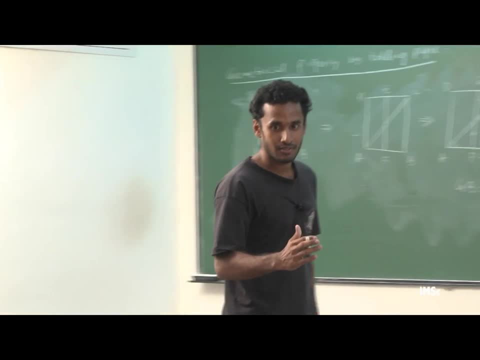 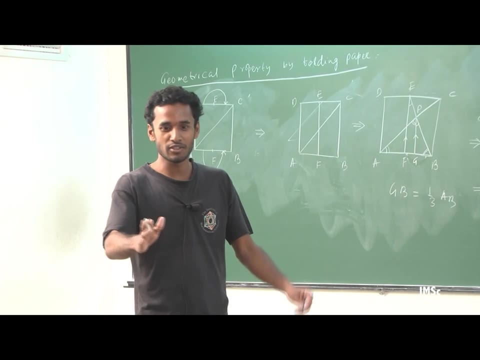 one fifth of this line. So the first class will over. at what time? No, no, no, the first class: 10, 15.. 10, 15. 10, 15.. Oh, already you are saying Already it is over. Yeah, Oh, you need a break. No, sir, So 10 minutes or 5 minutes? 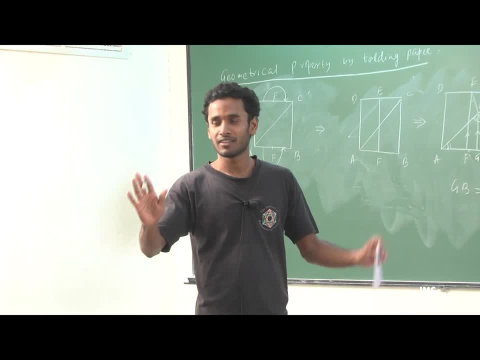 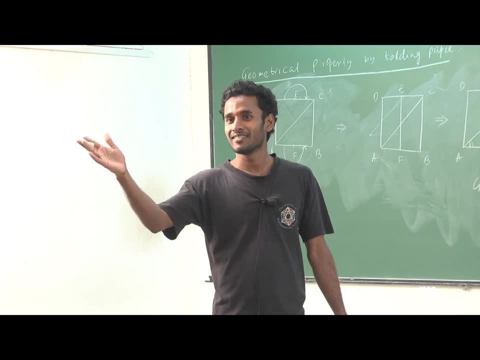 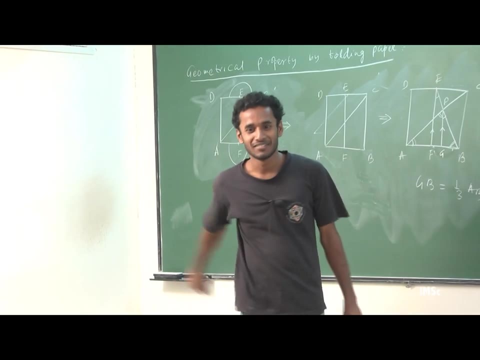 No sir, No sir, Continue, Continue. Anyone need break for 5 minutes or 10 minutes? Nothing, Continue. Are not you getting bored? No, Okay, So how to get Sir, instead of making 2 marks? 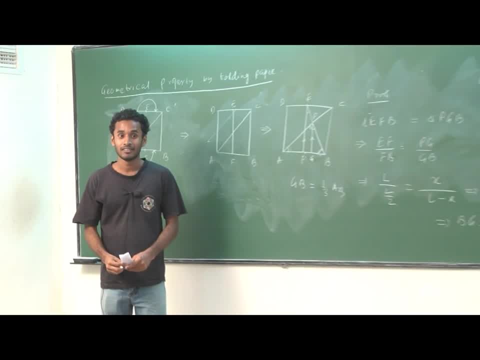 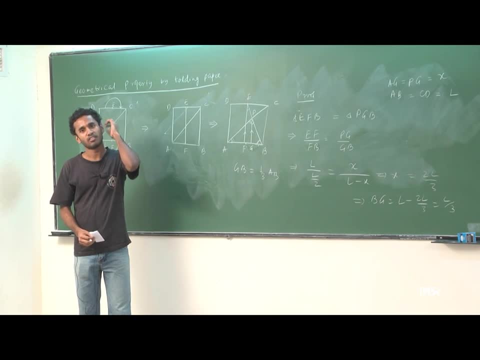 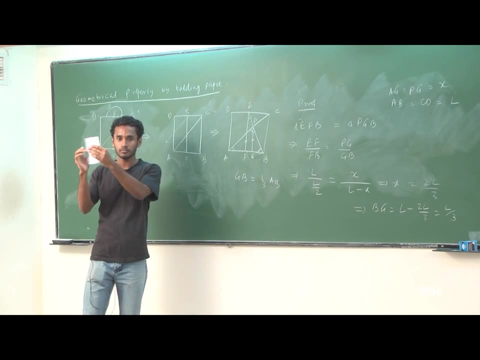 make 4 arcs, like, instead of making 2 arcs like here- I am not making any arc there, No, sir- like by folding paper or by construction, Anything, So by construction, By construction, you can just make 4 arcs, 4 arcs, Yeah, And by this Now one fifth. I have got this. g b is one third. Now I want. 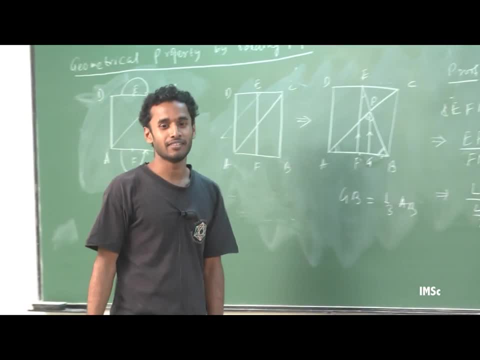 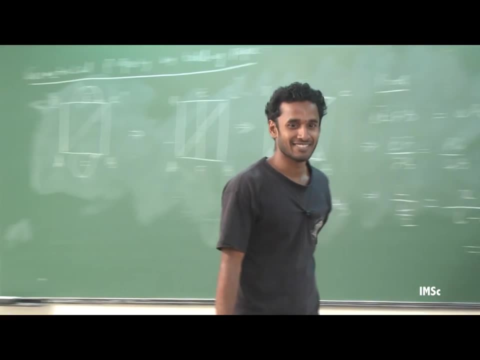 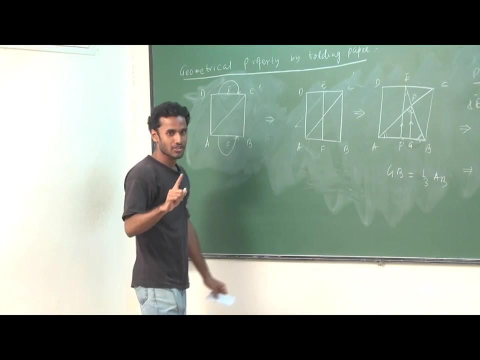 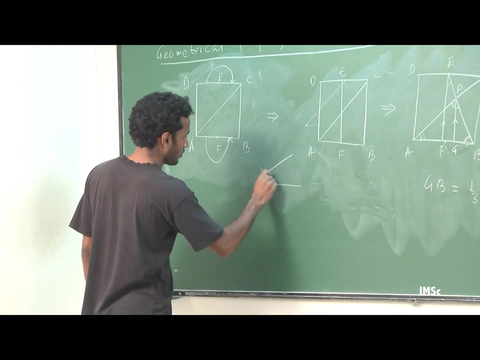 to get one fifth of a, b. So sink it, Okay, Okay. So I have told you to sink 2 sinks Right At first, that construction, Yeah, Why that should work. It is one third. So what I have done, I have drawn same angles and take same 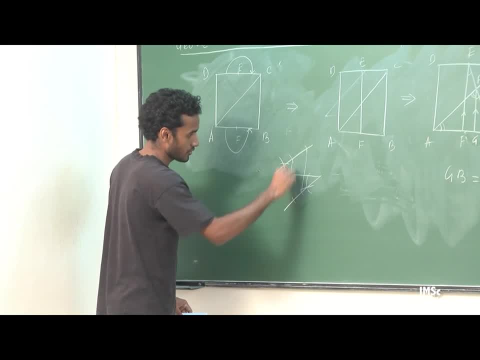 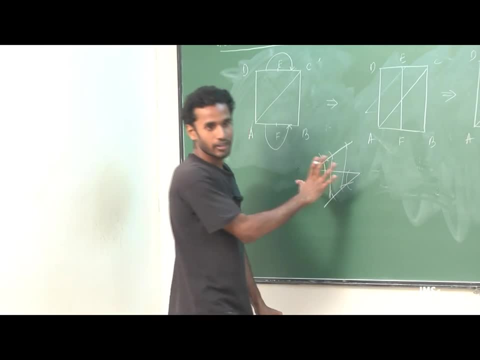 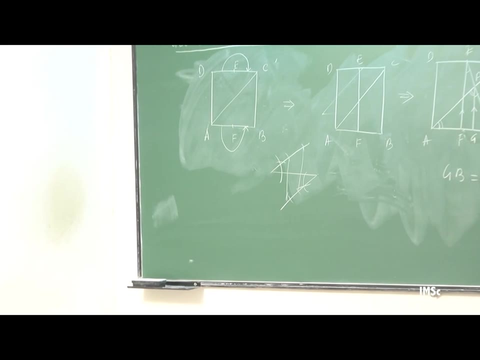 arc, Same arc And again same arc, and then join this And the claim is: this is one third of this pole And the. now the question is: why does this work, Sir? similarity, Sir, Just prove it. Yes, Okay, not now, Sir, break. 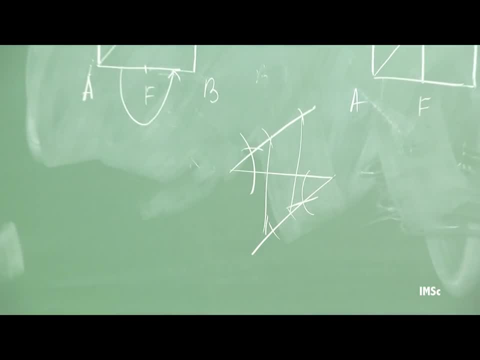 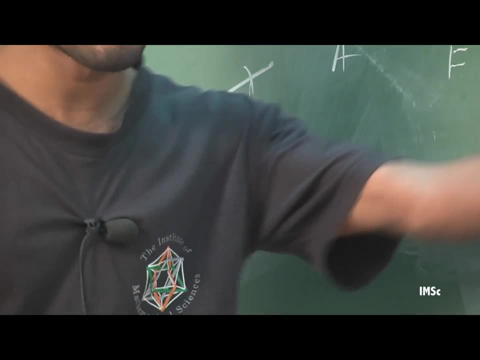 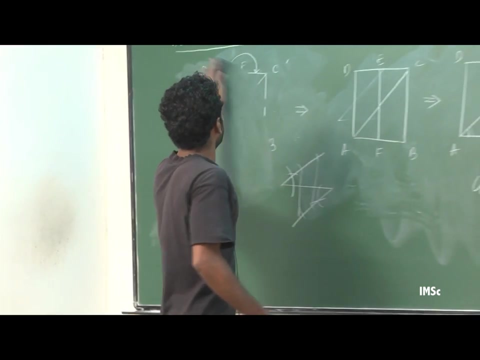 Break. Yes, You want break. No, sir, We have proved the break. Okay, Okay, Just, and this one, and how to get one fifth. I have got one third. How to get one fifth? Okay, My third thing, right. 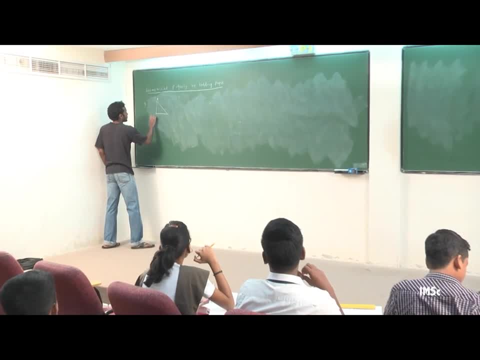 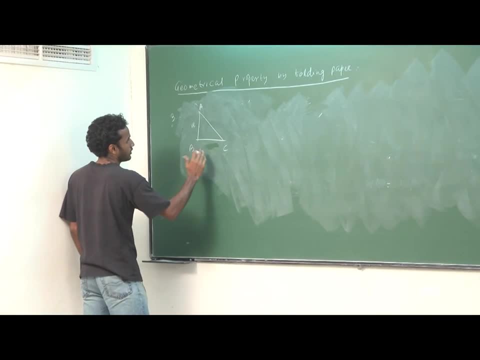 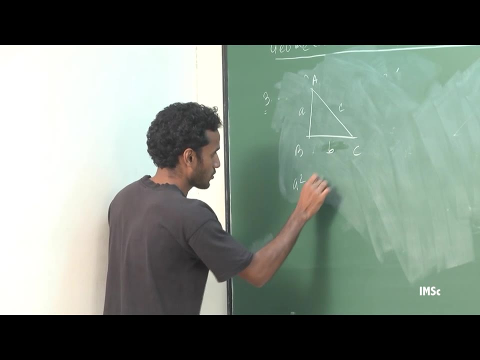 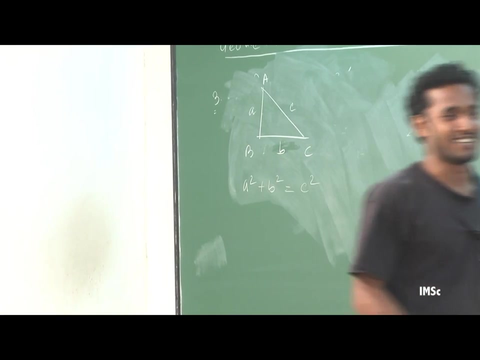 So if you have Come on a right angle triangle, Let me call it: length is a, the height is a and the. this is b and hypotenuse is c. So a square plus b square equals to c square. 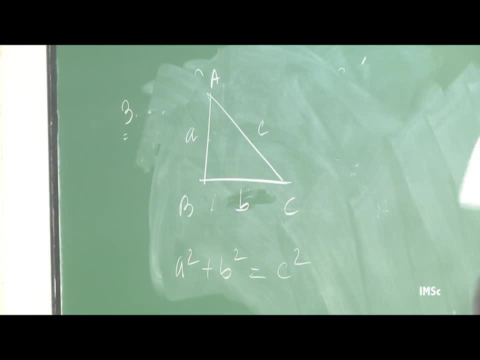 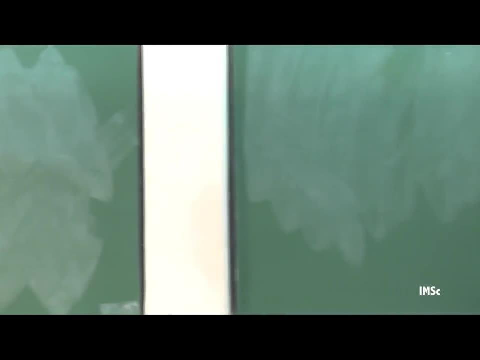 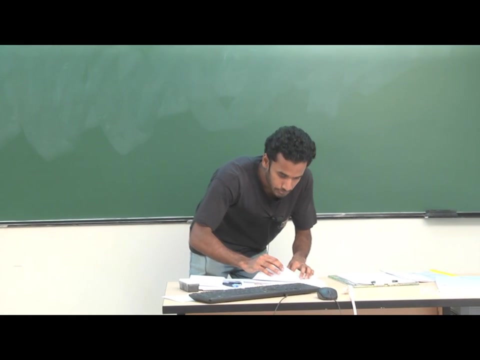 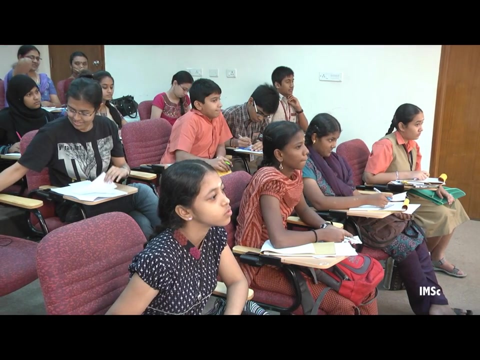 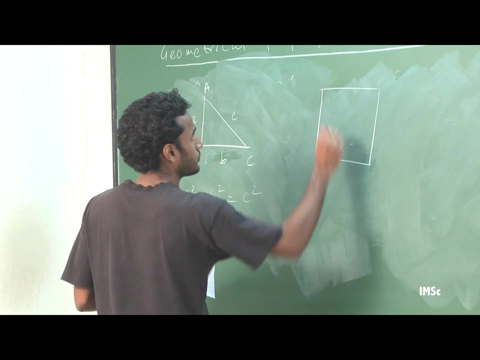 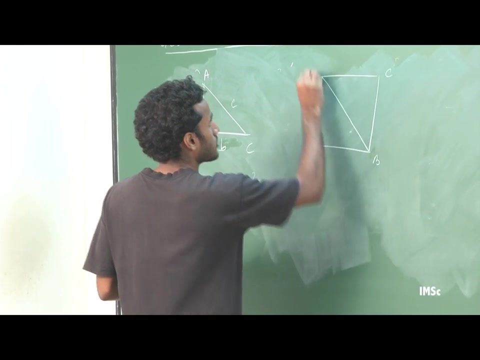 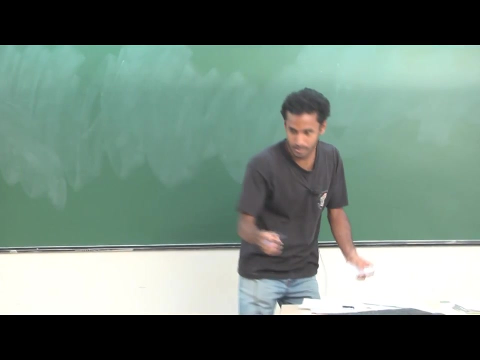 You have one, this small rectangular sheet of paper right Now. make a square of this, like previous thing: Any square, make any square and do it carefully, or else you will not get the thing correctly. So make a square. Let me call it a, b, c, d. Just name this square along these vertex. Just name it like that: a, b, c, d. 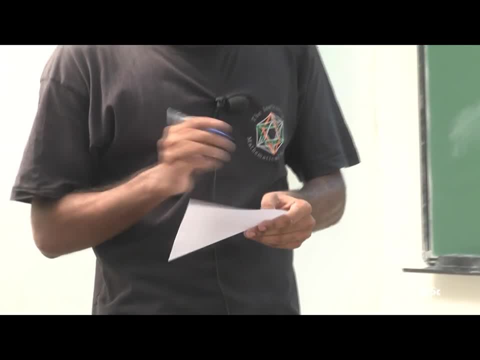 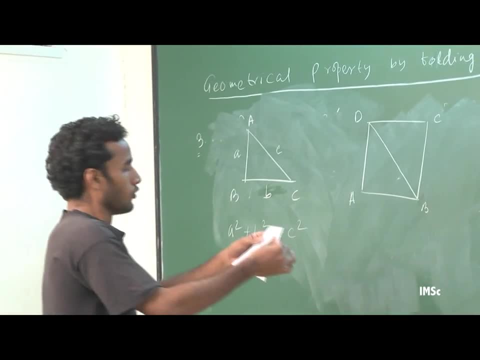 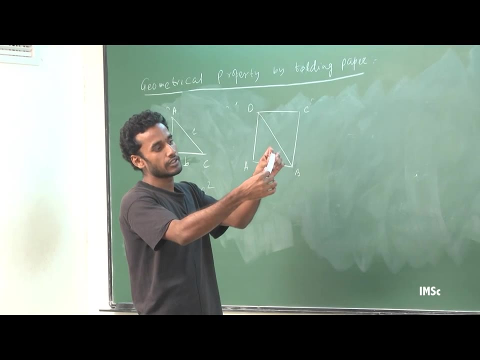 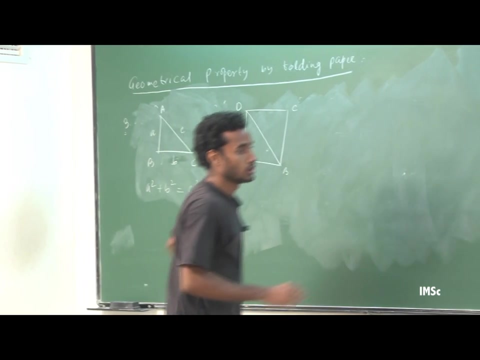 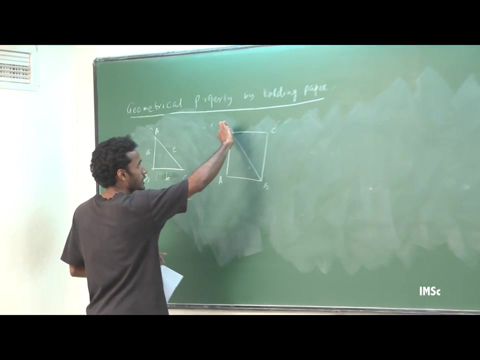 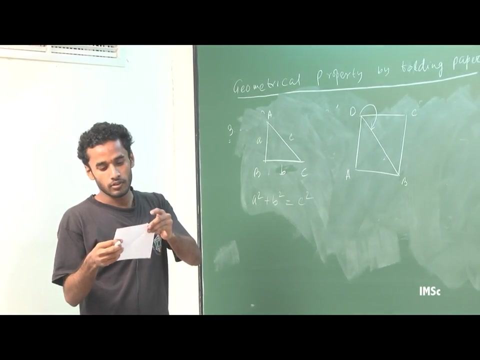 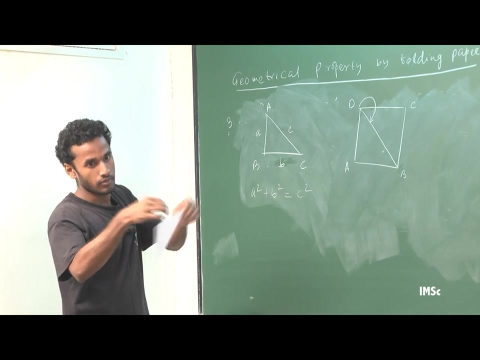 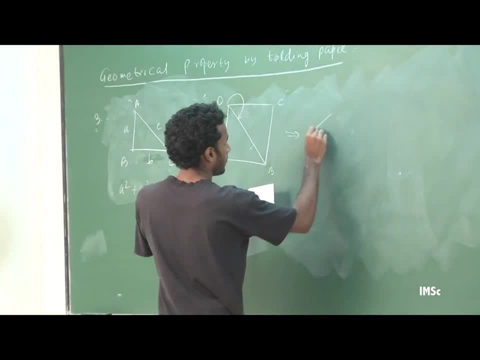 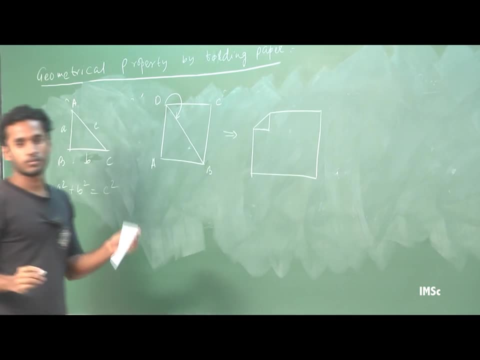 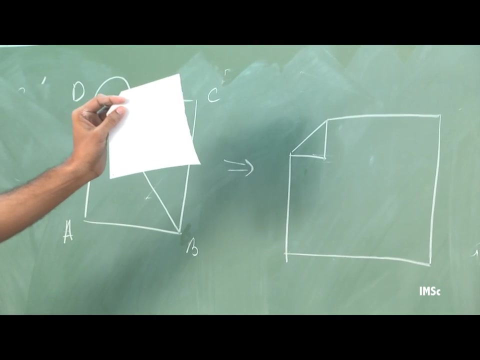 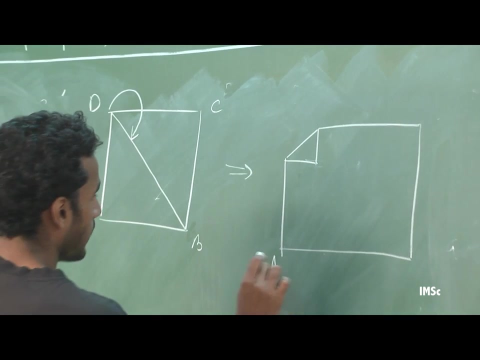 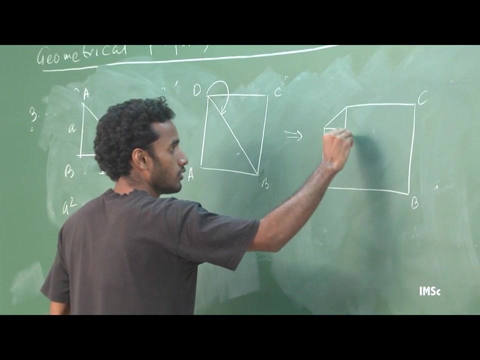 got. the figure should look like this. So what you have got. the figure should look like this: Everyone has got this right, Everyone has got this. This is this Now. this is my a. Now this is b, this is c and this is the diagonal. Now fold this opposite vertex b such that it touches the diagonal, like this: 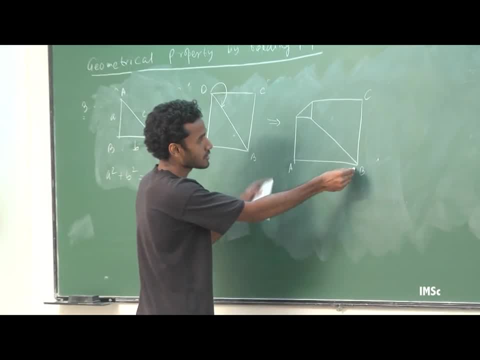 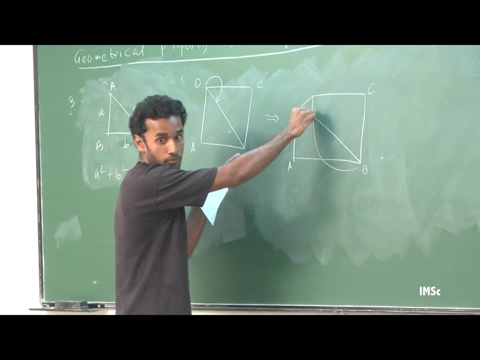 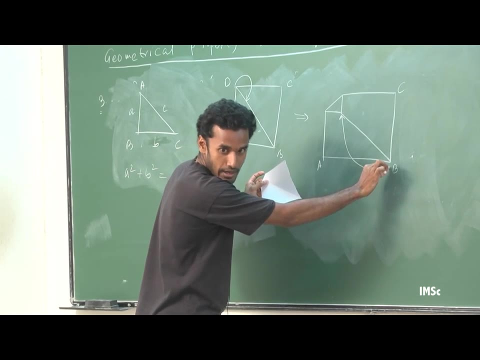 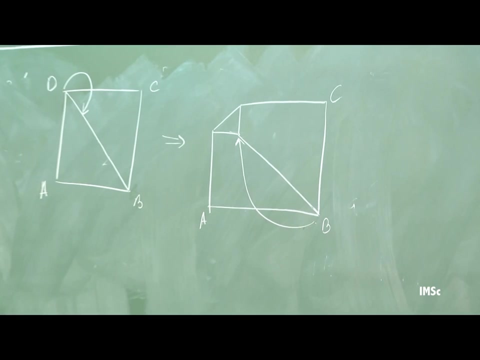 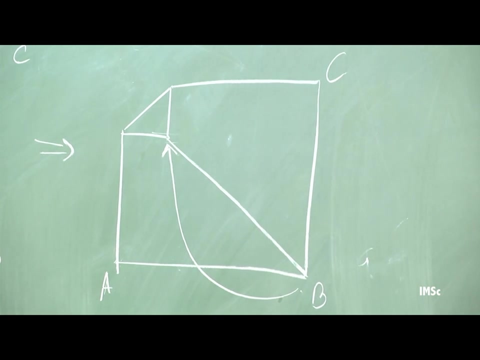 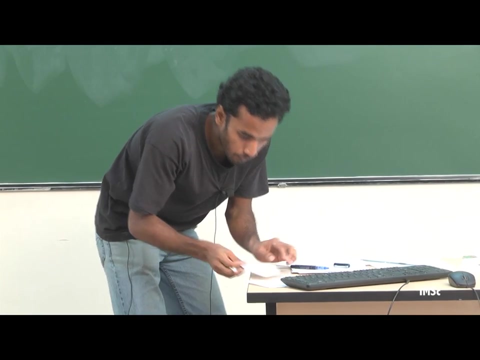 Now fold this opposite vertex b such that it touches the diagonal, like this to the diagonal and touches to this point also. Everyone has got this. Fold this D such that it touches the diagonal and touches that point also, like Everyone has done this It. 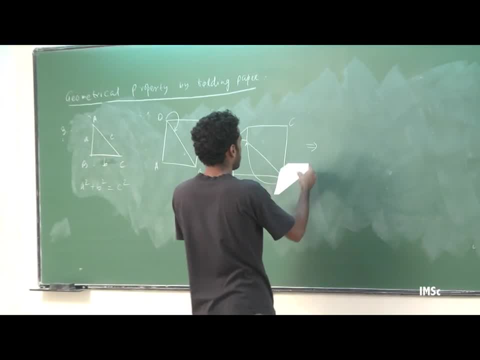 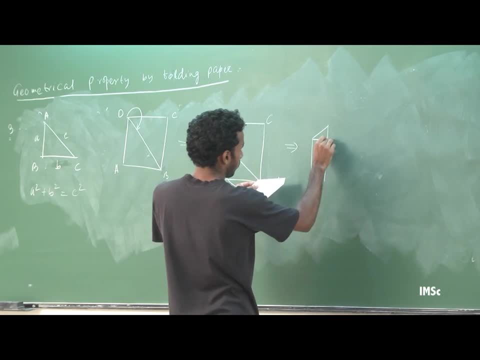 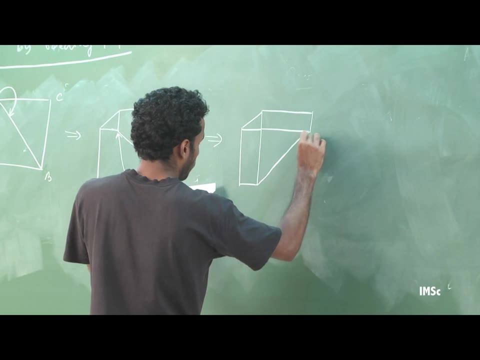 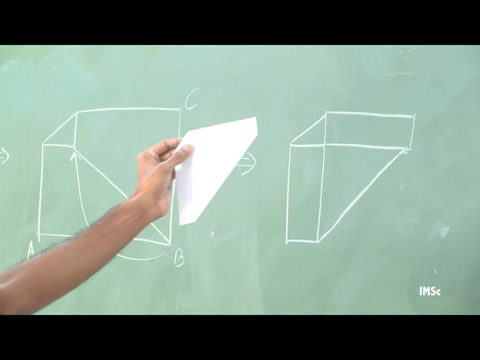 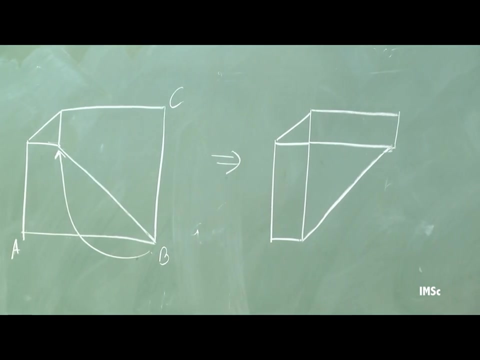 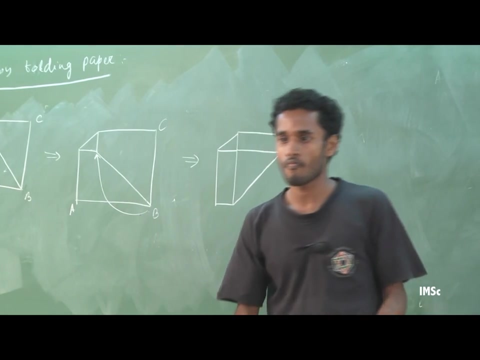 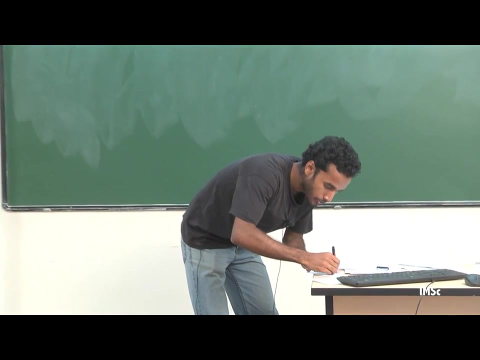 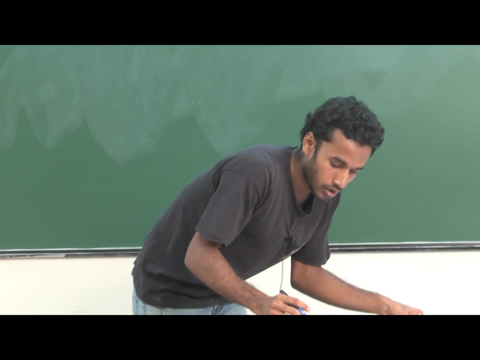 should look like. It should look like This one, Like this, Everyone has like this. Now draw lines with your pen or pencil along these lines: This one and this one. Draw a line along these lines. Draw a line along these lines. 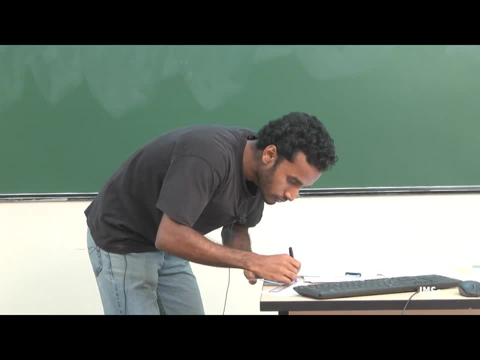 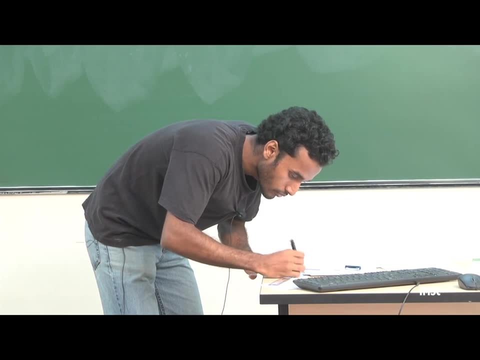 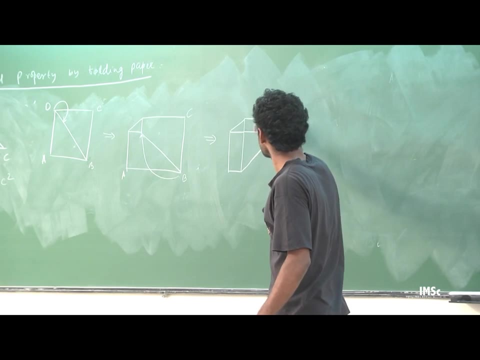 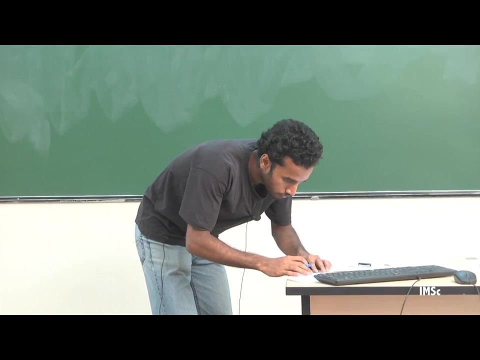 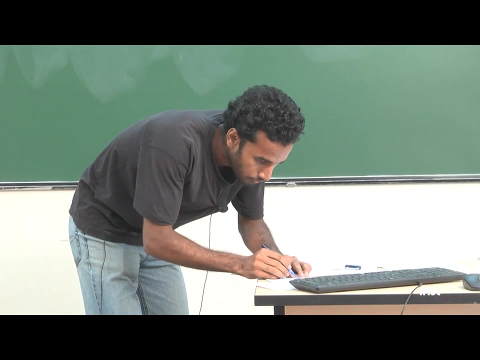 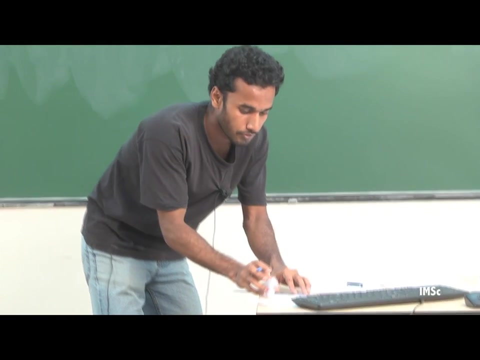 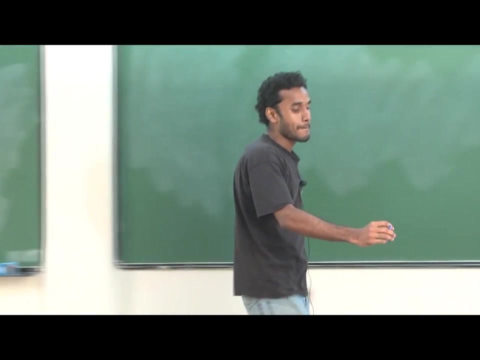 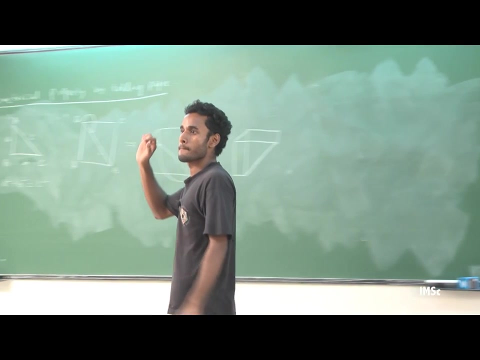 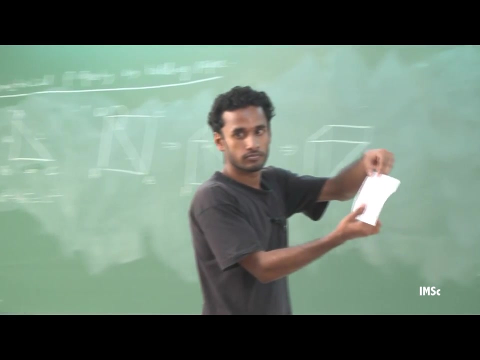 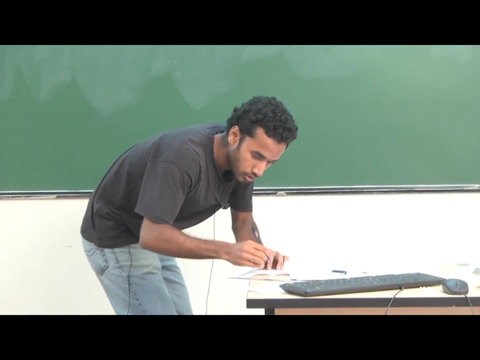 Draw a line along these lines. Draw line along this one and this one, this and this. All of you have drawn this line and unfold it like this. So, if you have drawn line properly, it will look like the figure will look like this: 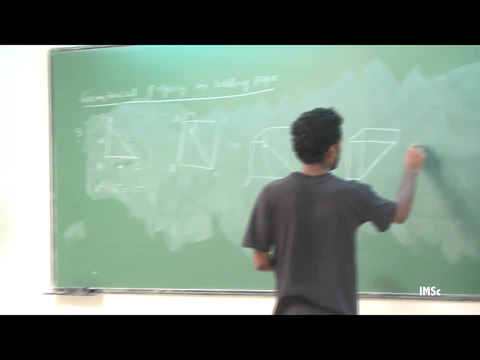 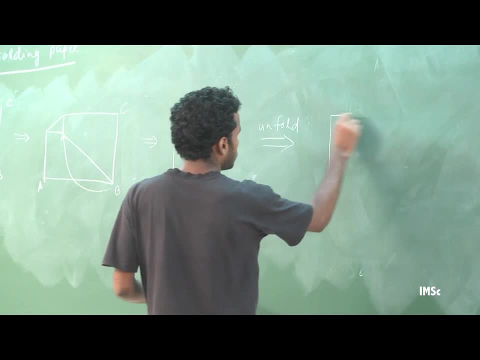 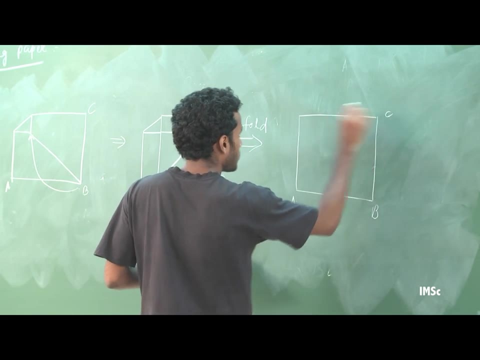 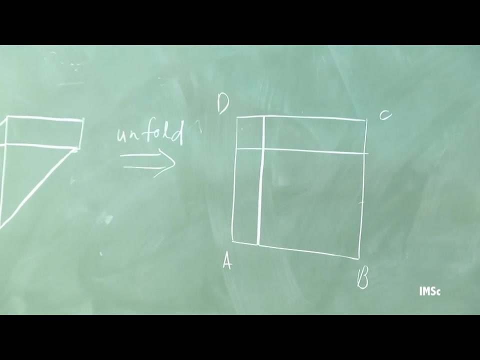 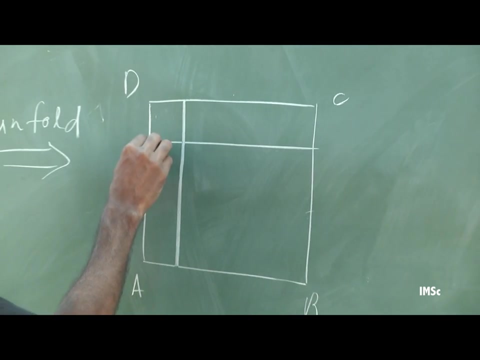 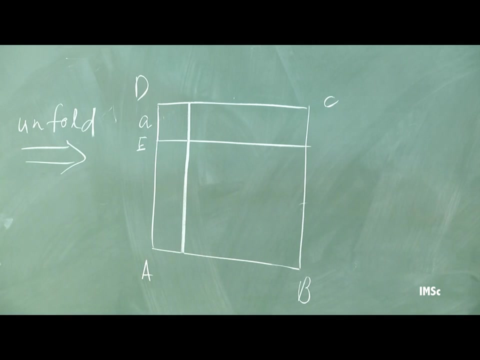 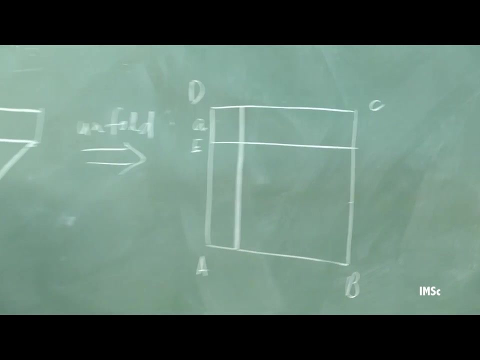 Unfold it and have A, B, C, D, Right, Everyone has got like this. Yes, Okay, Let me call this. This small length we call A, Let me call E, And this small length, D, E is A. 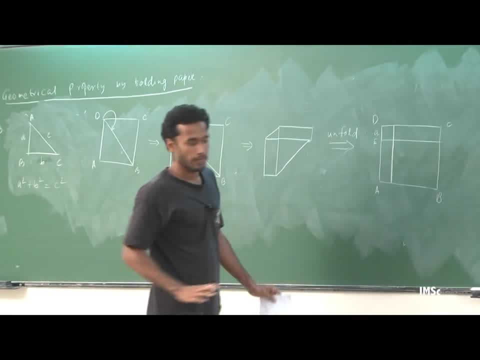 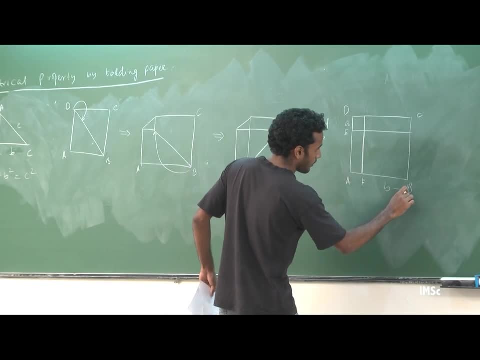 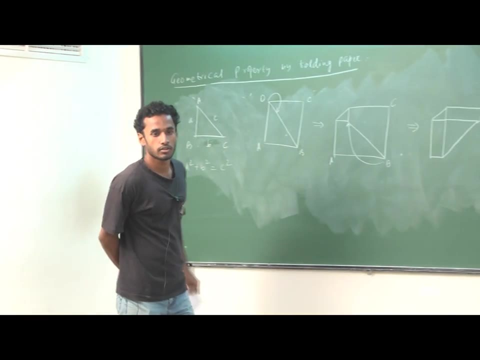 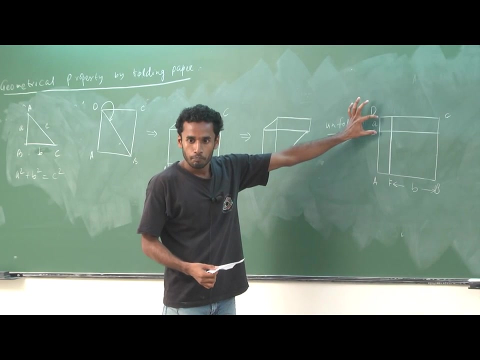 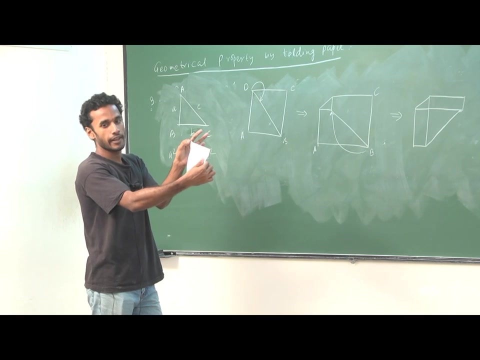 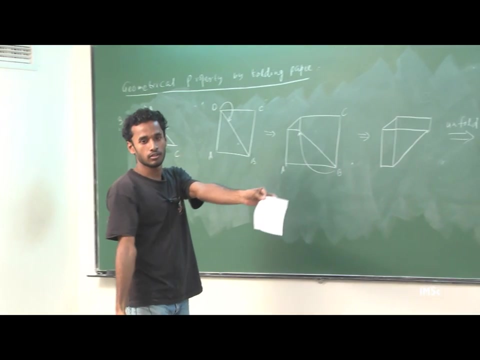 Let me just let me call that A And okay, let me call it F And let me call this length B. F is small, b, Right. So I have told you this length is A, Right. So when I have folded this side, that means this side, A. when I have folded this point D along the diagonal. 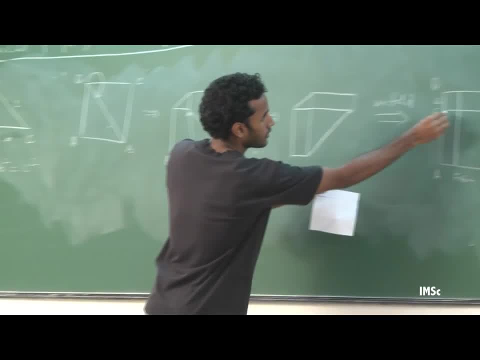 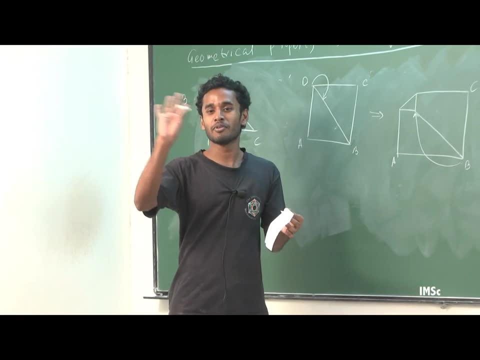 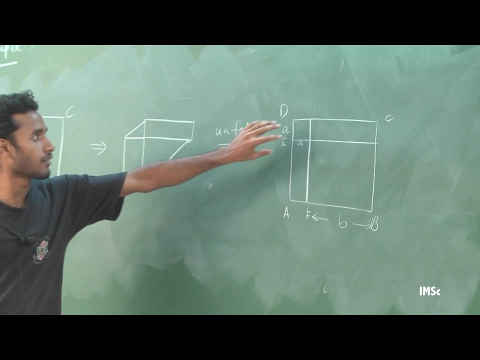 So now, what is this length now A? This length, A A. Everyone agrees with this. Yes, Yes, Everyone, Yes, Good, This is also A Right, And this small quadrilateral is now a Square Square. 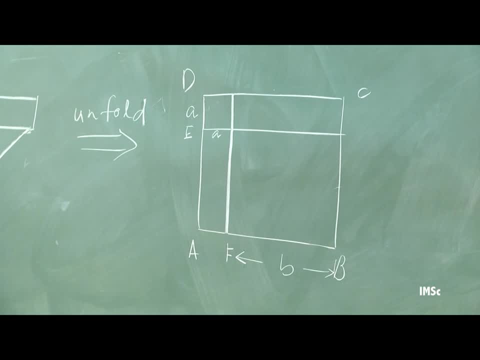 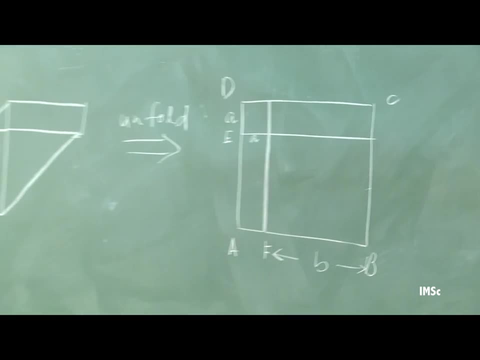 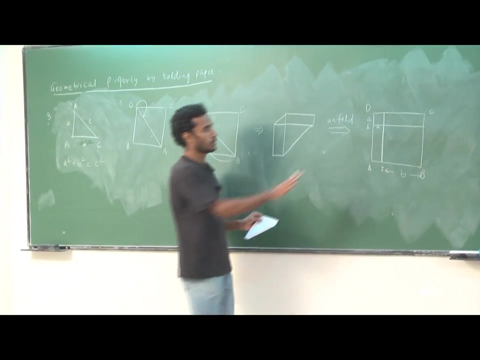 Good Square of length A, A. So now I have done the same thing for the vertex B also, Right? Yes, So if this is B, this is also B, B. So this is also a square of length. 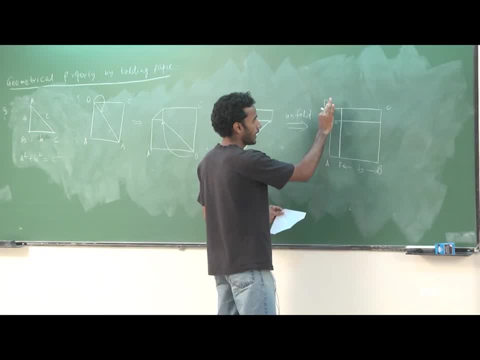 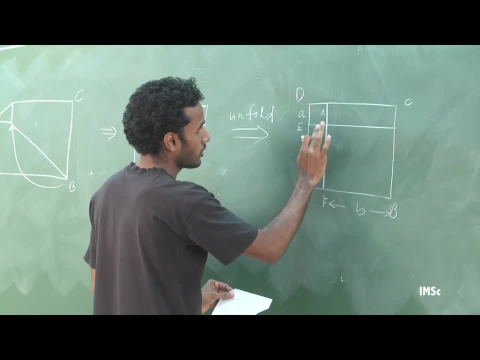 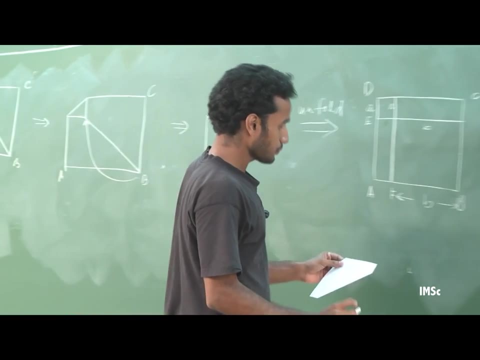 B, B, Right, And if this is A, this length should also be A. So let me write it here: This is A Here. If this is B, this is also B, Right, Yes, So now I have done A and this is also B. Where is B? 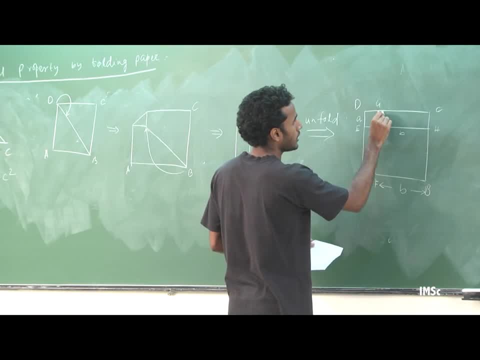 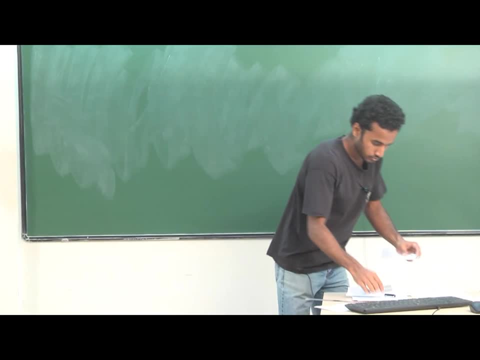 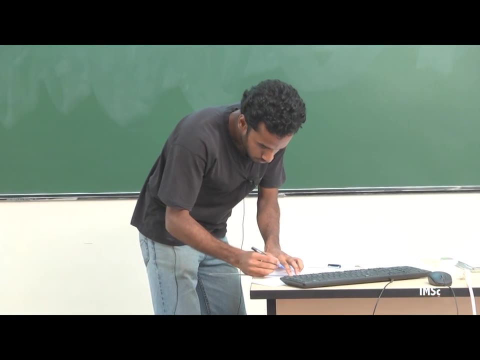 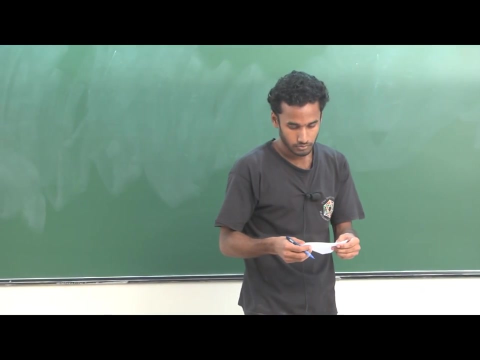 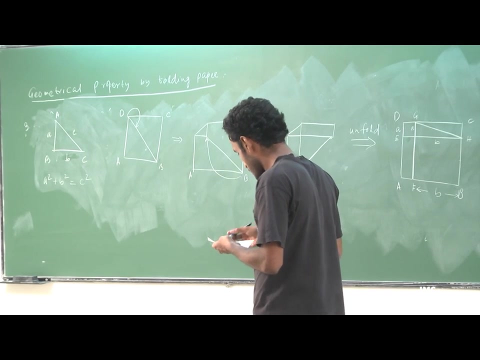 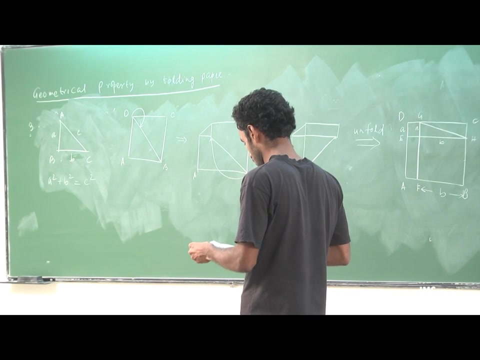 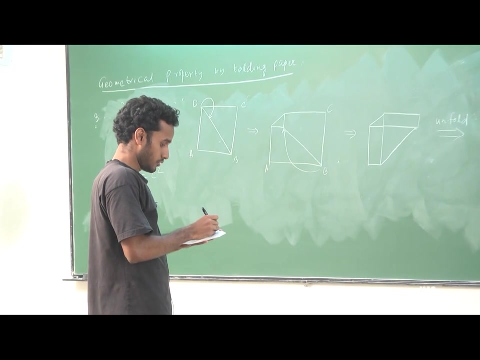 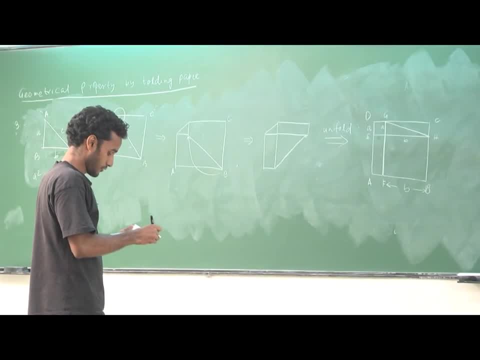 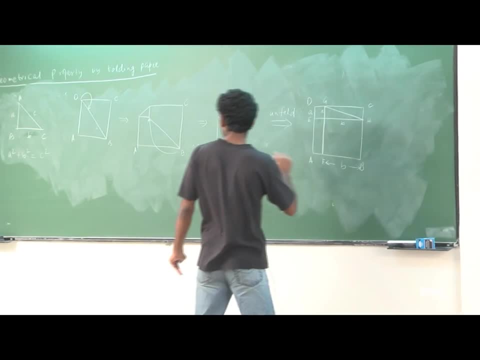 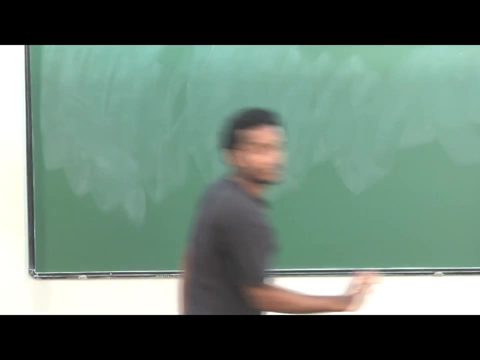 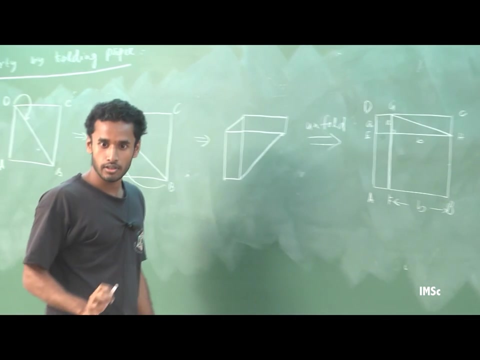 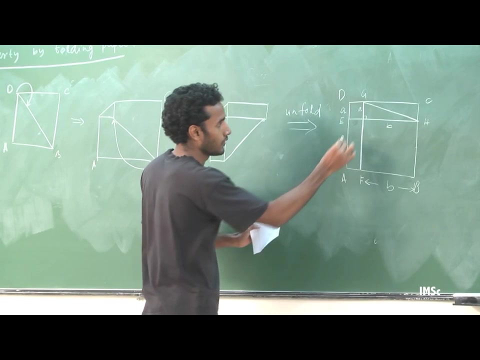 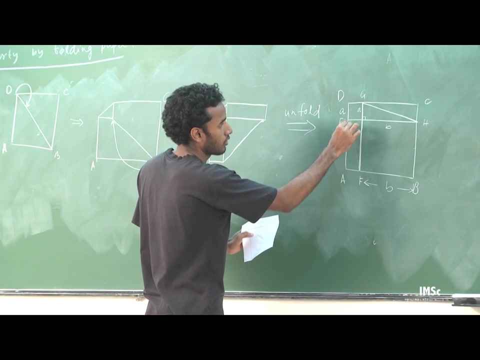 Just let me name these things, What I have done here. I have created a small square, a big square and two rectangles, and this one is a right angle triangle and here this one is also a rectangle, So you have two rectangles. So if you draw a diagonal, just for it is a, again here there is two rectangles, right. 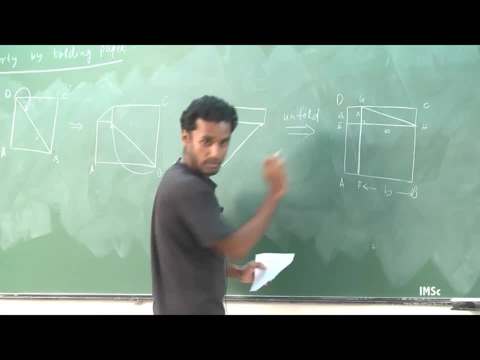 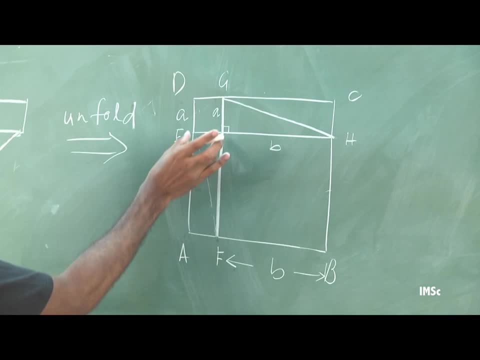 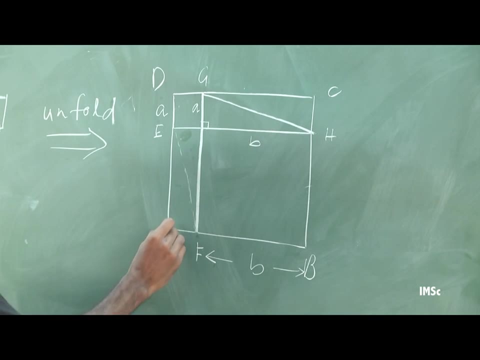 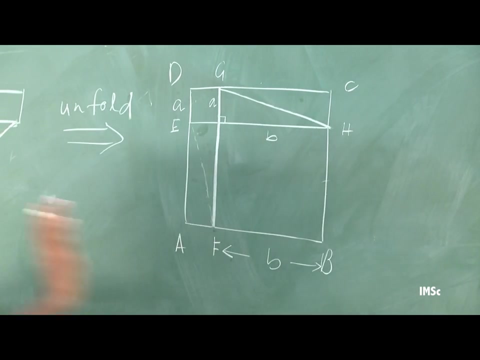 angle triangle. These two are also right angle triangle and the length are all the same. This is a, this is b. this is a. this is b and this is a. this is b. Yes, And this angle is common to both: 90 degree, So that means these four triangles are good. 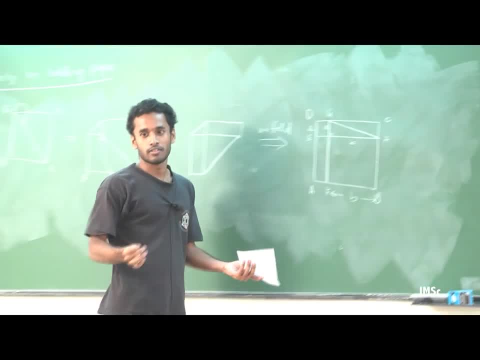 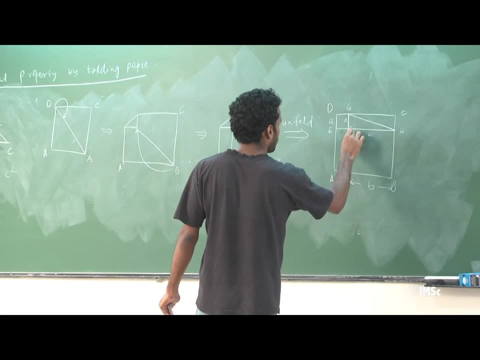 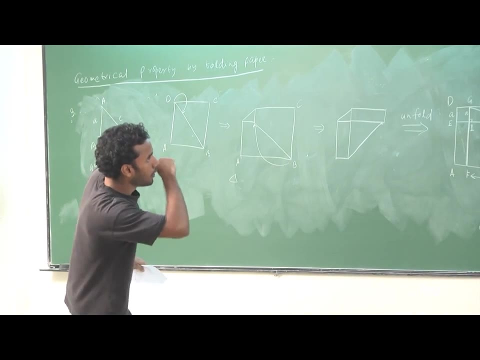 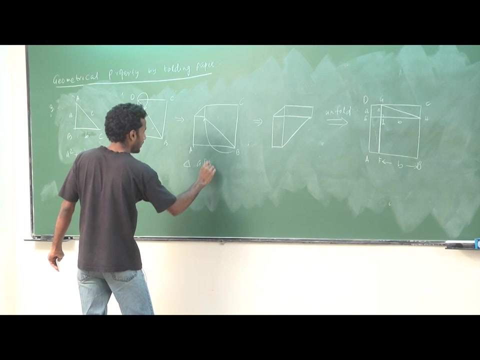 These four triangles are congruent to each other, right? Yes, Just let let me write it: g, h, i. So angle in front side. Yes, Right, Yes, So this is a right angle triangle: g, i, h, right. 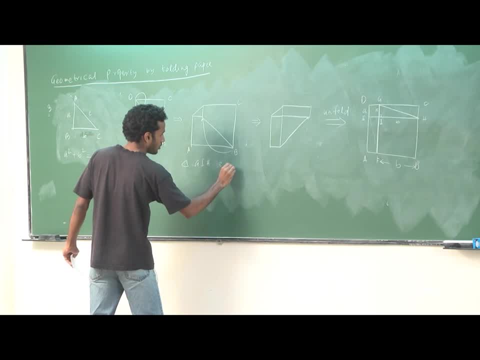 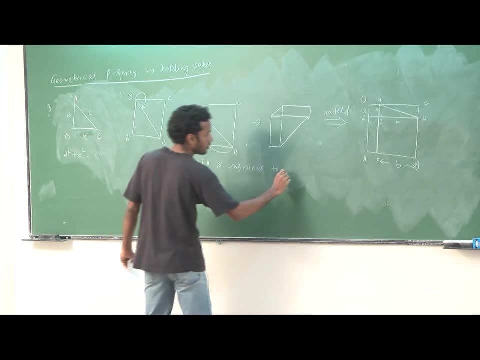 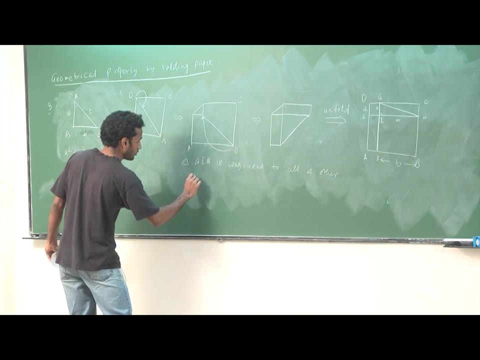 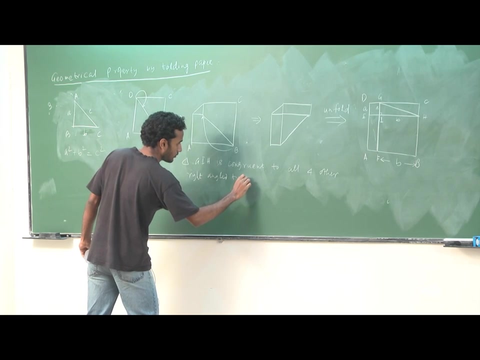 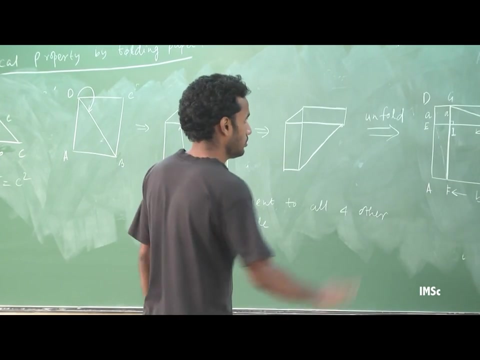 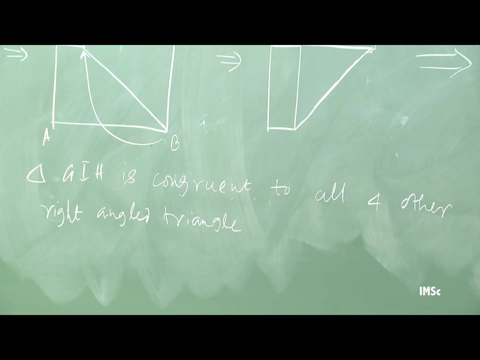 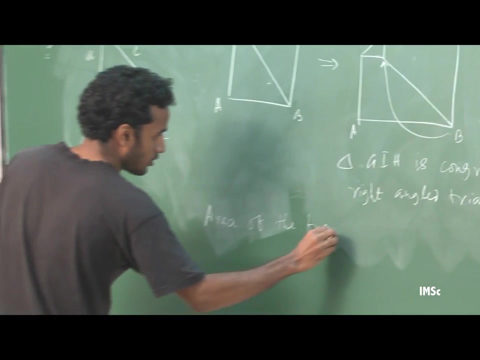 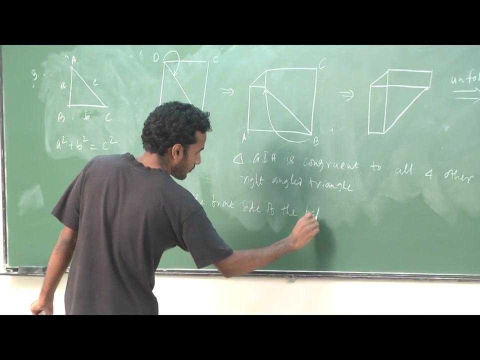 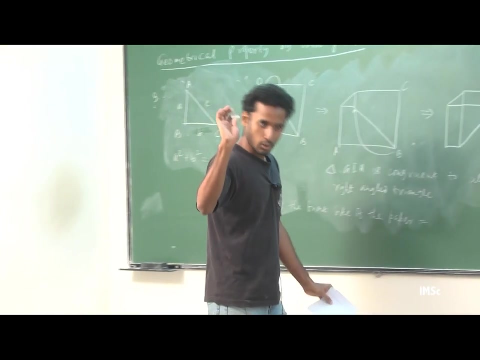 G, i, h is congruent to all four other right angled triangles. Okay, Yes, Yes. So now tell me what is the area of this paper? What is this? Yes, a plus b, whole square. So I can write this: a square plus b square. 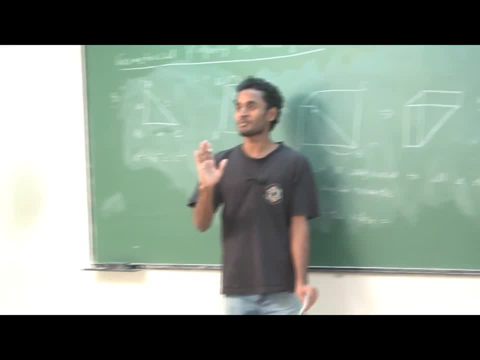 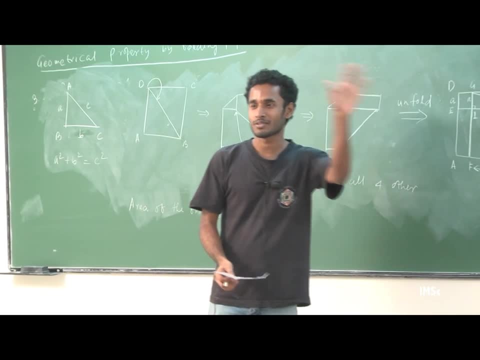 plus Yes, a square plus b. square plus 2 a b also. So that proves the that also a plus b square b whole square equals to a square plus b. square plus 2 a b. I am not going to that, So I. 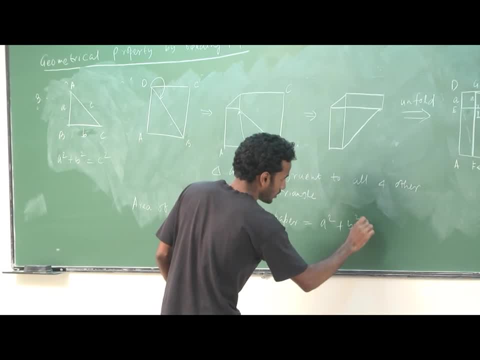 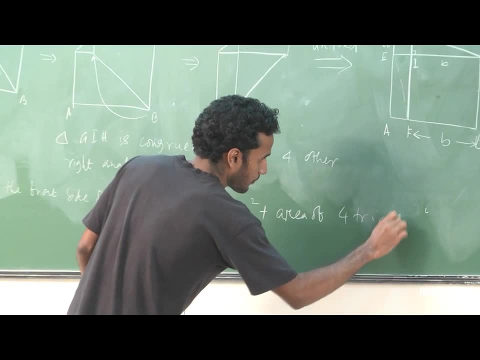 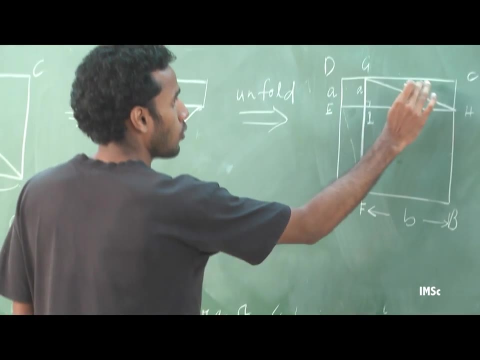 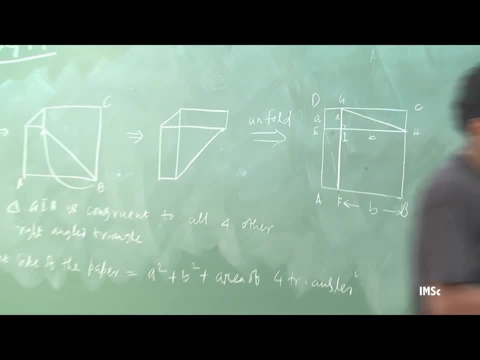 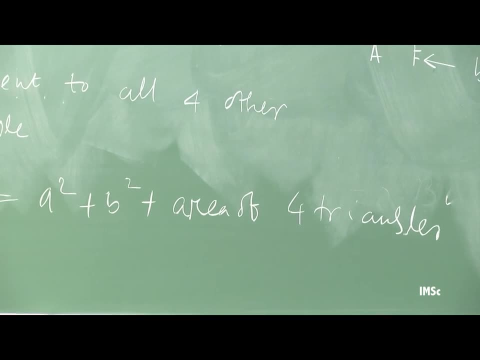 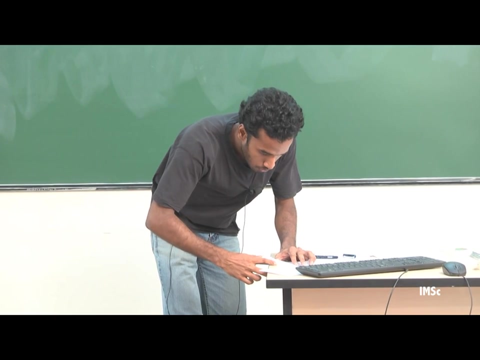 Yes, Now fold the back side of this paper along the hypotenuse g h. Let me just show you once again. Yes, Fold the back side of this paper along the hypotenuse g h. Let me just show you once again. 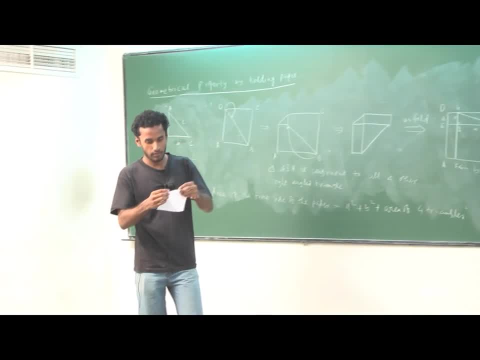 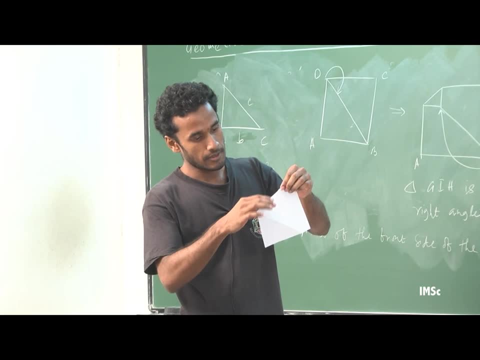 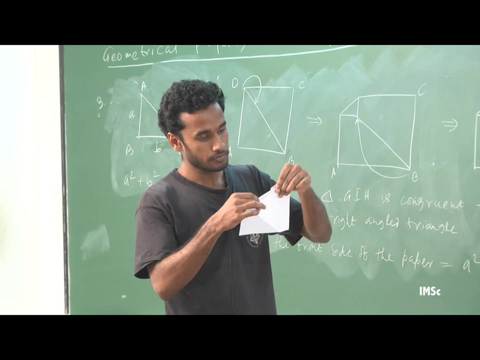 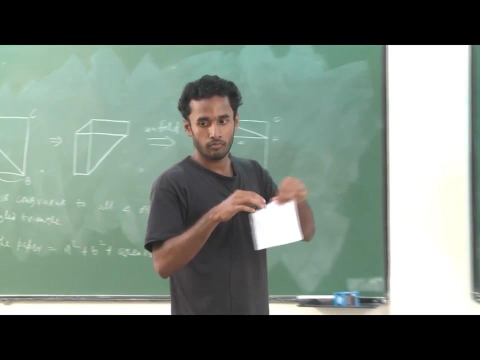 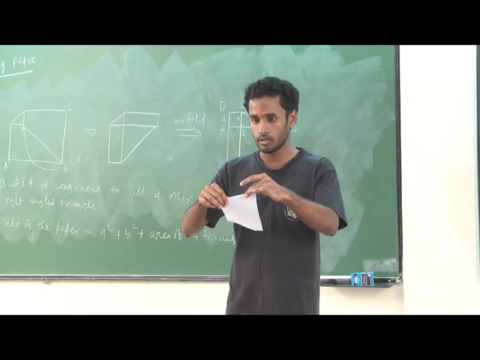 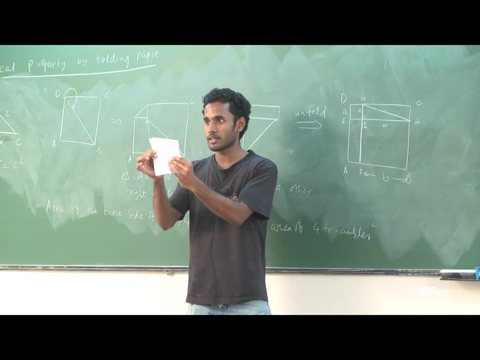 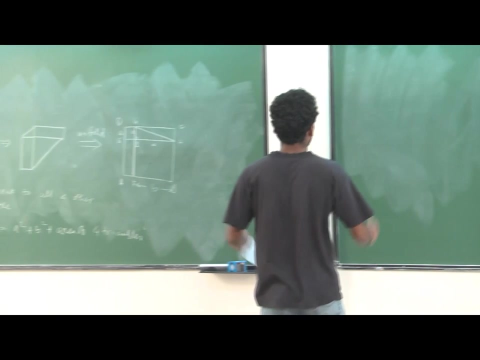 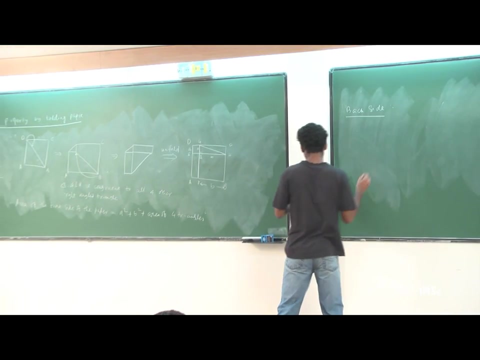 Yes. Now, now one more time: Yes, Like this, Yes, Yes, Yes, like this. and now look at the back side of this paper. Just rotate it and look at the back side of this paper. So how does it look? This is the front side. So this looks like: 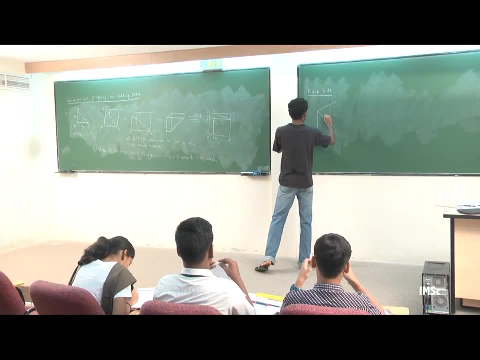 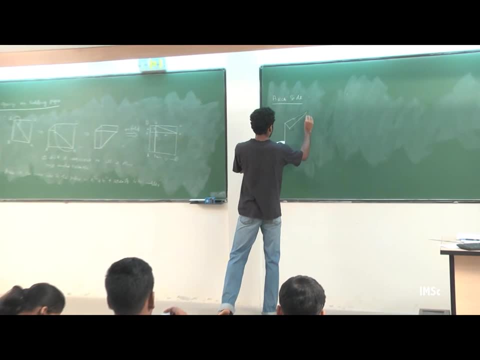 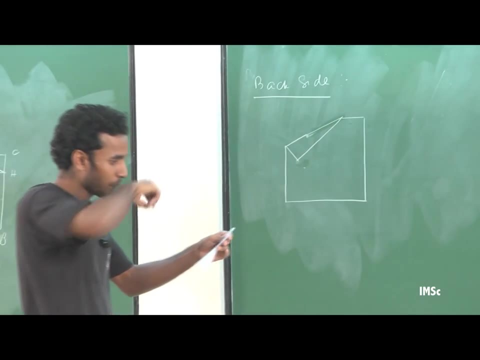 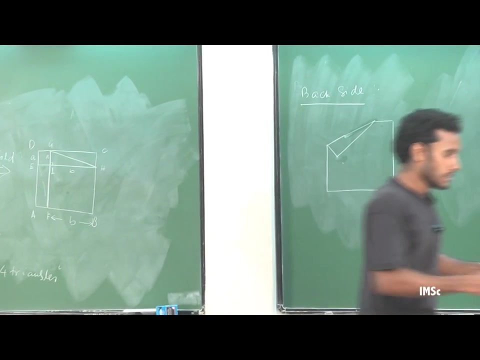 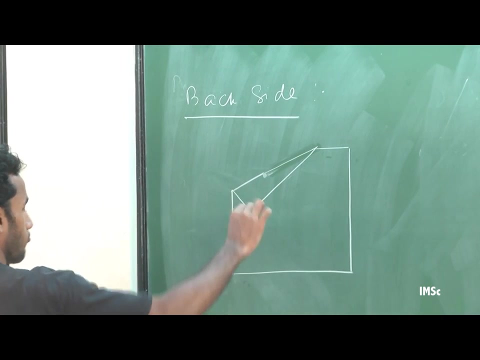 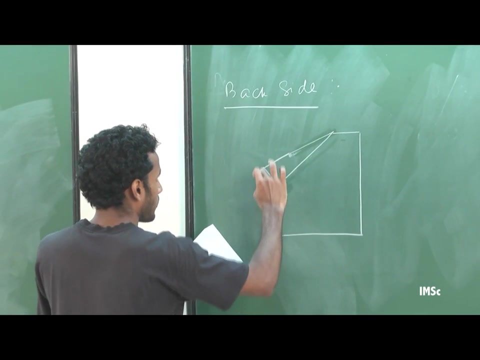 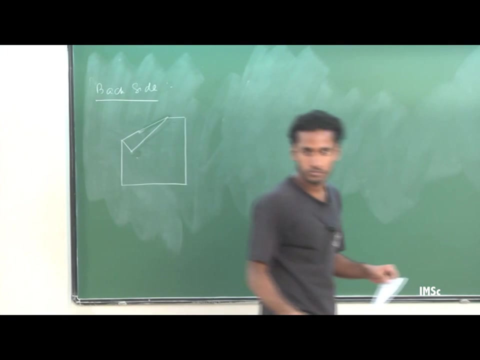 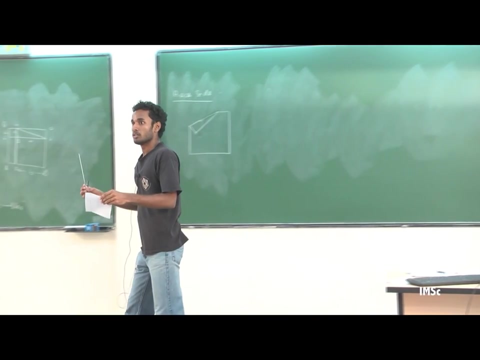 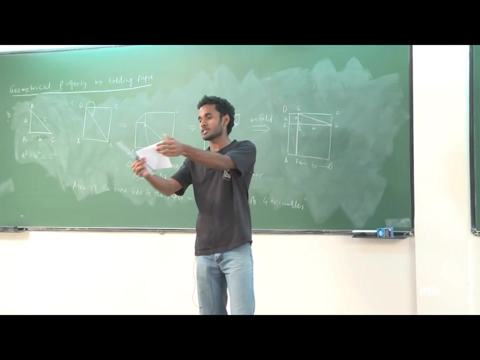 this, right. This looks like this, right. This looks like this. right Now, draw line along This. draw line along this one, this one and this one. Draw a line along this triangle Behind the seat, behind the seat. Everyone has got this. You fold with respect to this. 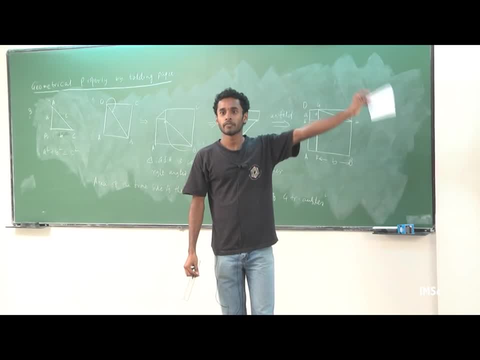 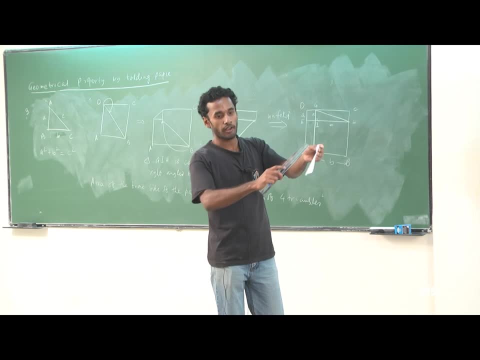 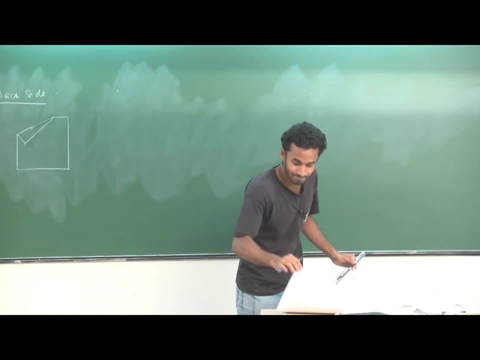 hypotenuse. in the back side- Now behind the seat, back side of this paper, draw line along this triangle. Sorry, Yes, Everyone has drawn this. Yes, So just draw along this, Yes. 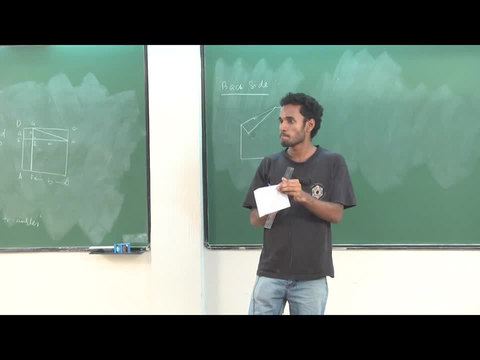 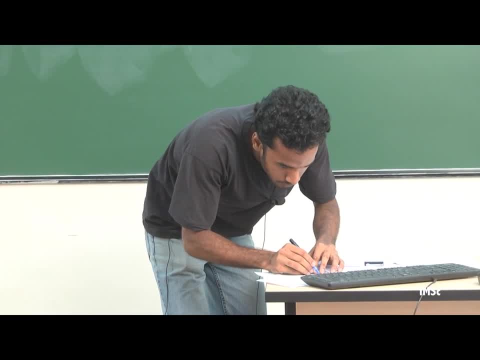 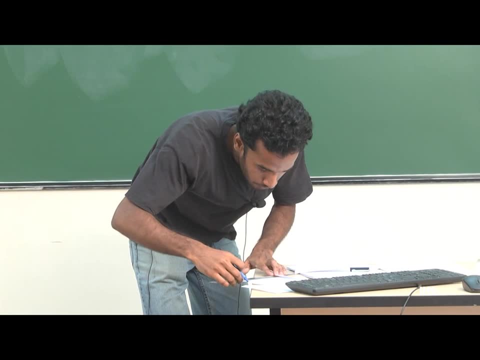 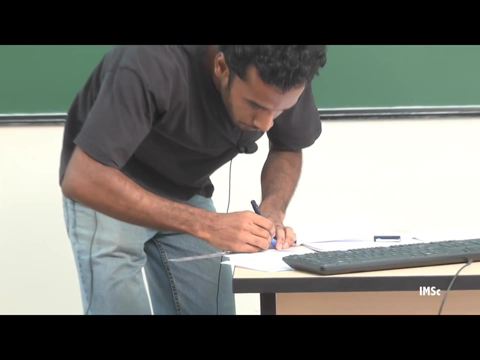 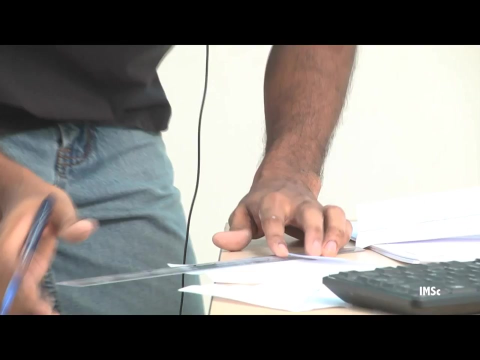 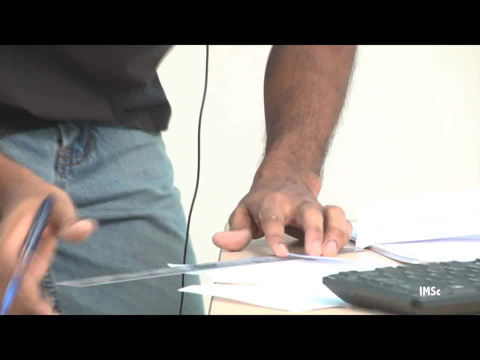 name those corner where there is A right, just A prime. A prime means just if in the back side it should be right A prime and it is now the A prime should be here. A prime, A prime, B prime- this is B prime. Now C prime has come here. just call them just prime. where? 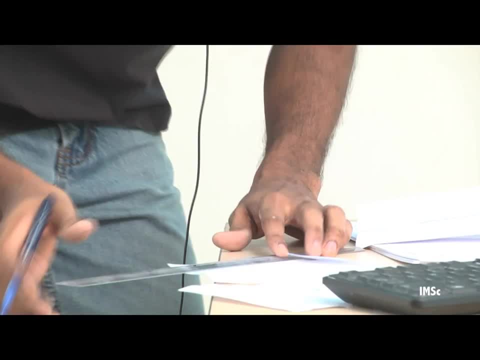 there is A, B, C, D in front side. just look at the back side. Subtitles by the Amaraorg community- wwwamaraorg. Subtitles by the Amaraorg community- wwwamaraorg. Subtitles by the Amaraorg community. 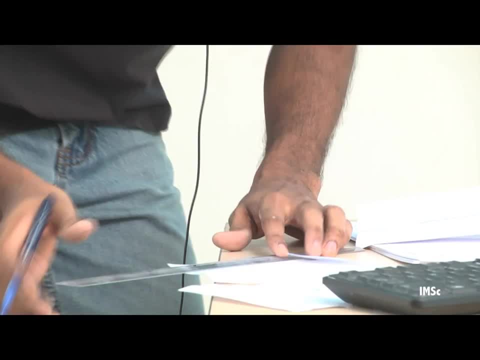 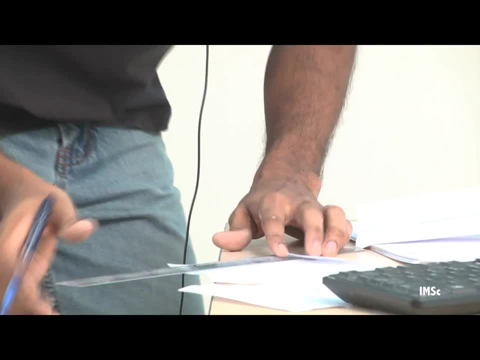 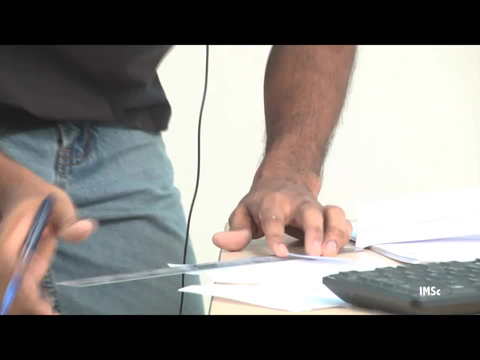 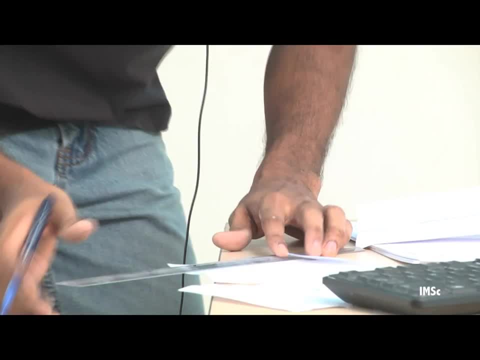 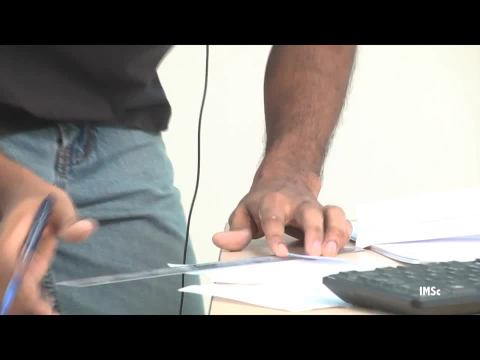